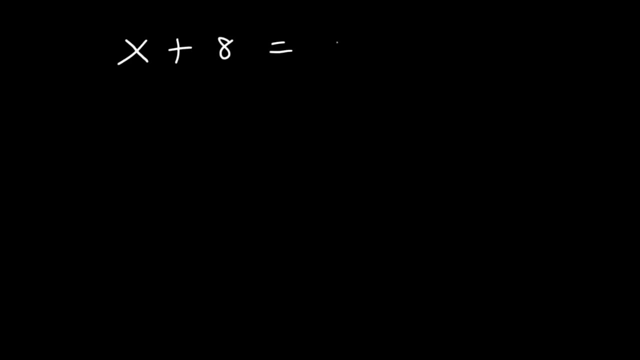 need to do is you need to be able to solve linear equations. So consider this equation x plus 8 is equal to 20. What is the value of x? x is basically a number. It's a number of which you don't know the value of. So whenever you see a variable, it's just an unknown number. 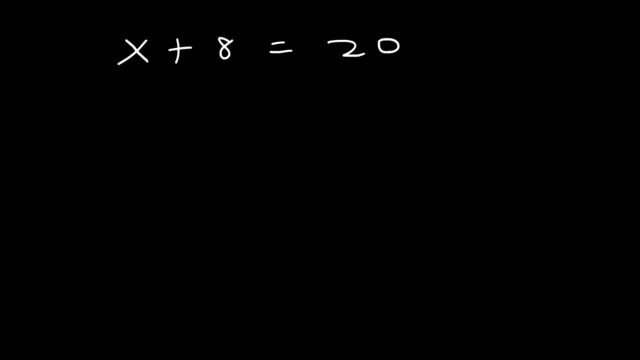 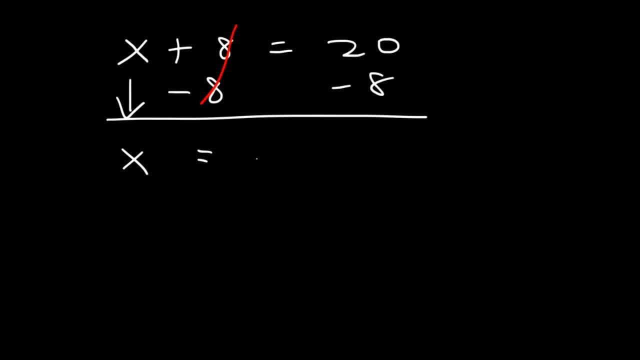 The answer to this question is x plus 8 is 0. You can bring down the x, and 20 minus 8 is 12. So that's the value of x. That's how you find it. Now what about this example? 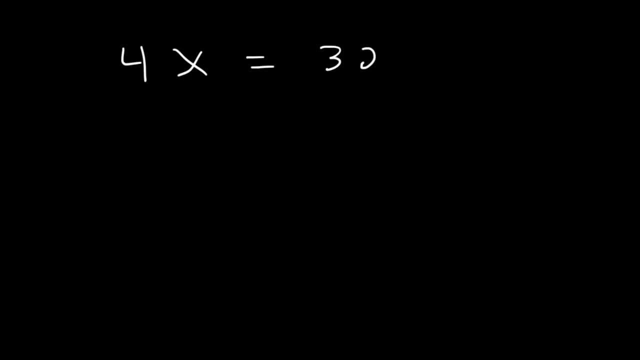 4 times what number is equal to 32? Well, we know that 4 times 8 is 32. So therefore, x has to be equal to 8. The 4 is multiplied to x. So in order to solve linear equations, or to find the value of x, you need to get x by itself on one side of the equation. 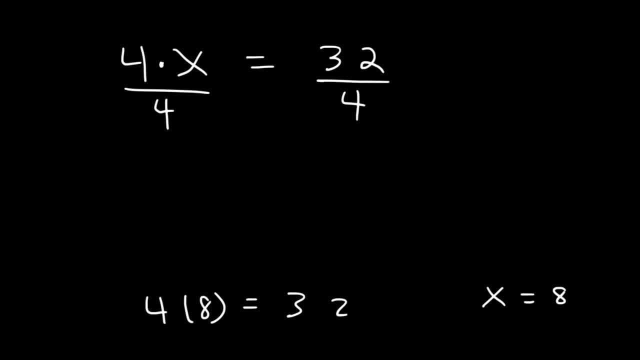 The opposite of multiplication is division, so we need to divide both sides by 4. 32 divided by 4 is 8, so that is the value of x. 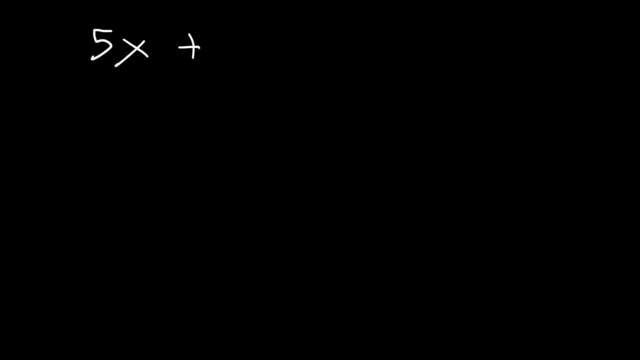 Let's try another one. 5x plus 7 is equal to 42. Feel free to pause the video and work on this example. 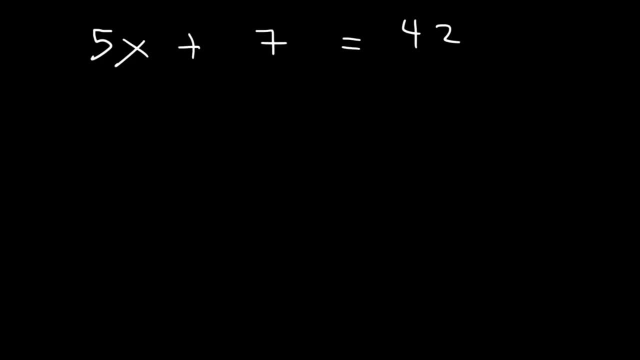 Now, we shouldn't divide everything by 5 at this point. The first thing we should do is subtract both sides by 7. Our goal is to get x on one side of the equation. 7 and negative 7 will cancel. We could bring down the 5x, so let's rewrite that. And 42 minus 7 is 35. Now, at this point, what we need to do is divide both sides by 5. So, therefore, the value of x is going to be, by the way, 5 divided by 5 is 1, so those numbers disappear. 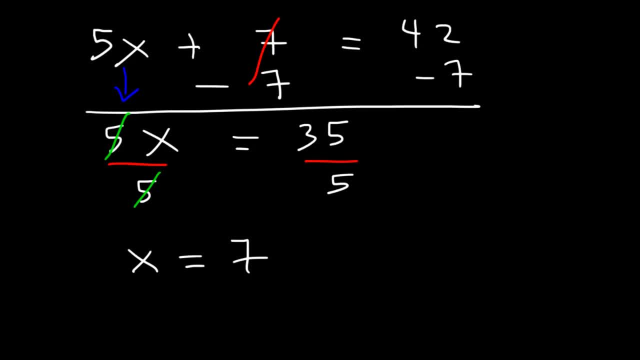 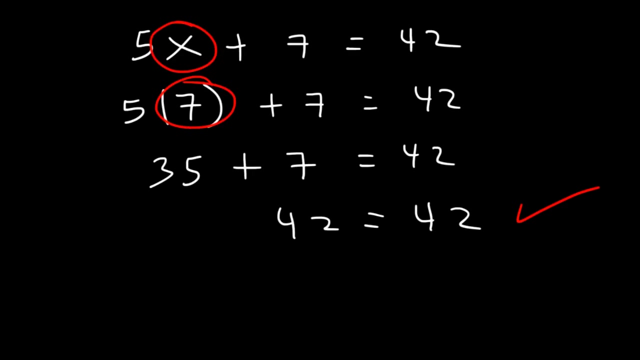 And 35 divided by 5 is 7, so x is equal to 7. And you could check to make sure that the answer is correct. And the way to check it is to plug it back in. Let's replace x with 7. 5 times 7 is 35. And 35 is 7. And 35 plus 7 is 42. So since the left side is equivalent to the right side, the equation is balanced. So x is indeed equal to 7. Now, here's another example for you. 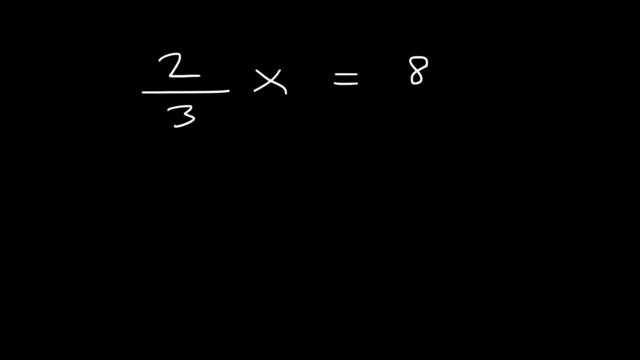 2 over 3 times x is equal to 8. What is the value of x? So how can we solve this particular equation? 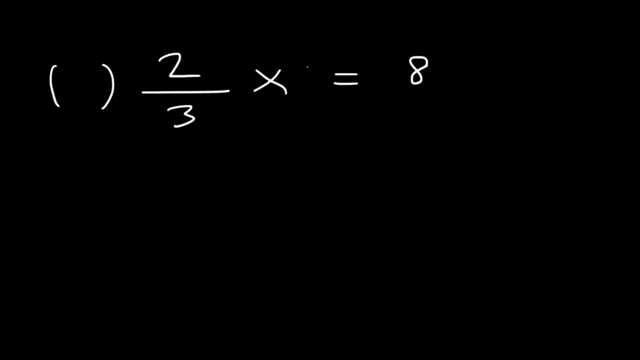 We have a fraction. What we should do is multiply both sides. Divide both sides by 3. And the reason why we want to do that is it's going to get rid of the fraction. 3 divided by 3 is 1, so those numbers cancel. 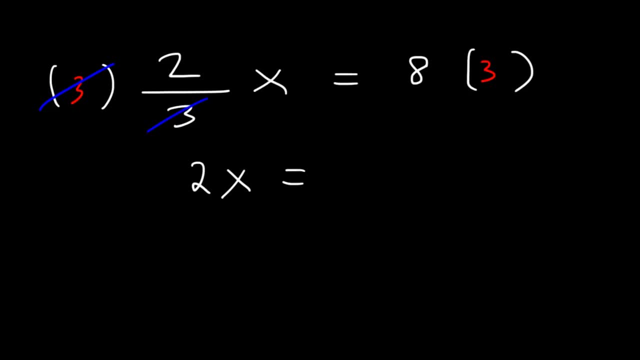 So on the left, all we have is 2x. On the right, we have 8 times 3, which is 24. Now the only thing that we need to do at this point is divide both sides by 2. So 2 divided by 2 is 1. So this is equal to 1x, which is the same as x. 24 divided by 2 is 1. 24 divided by 2 is 12. So therefore, x is equal to 12. 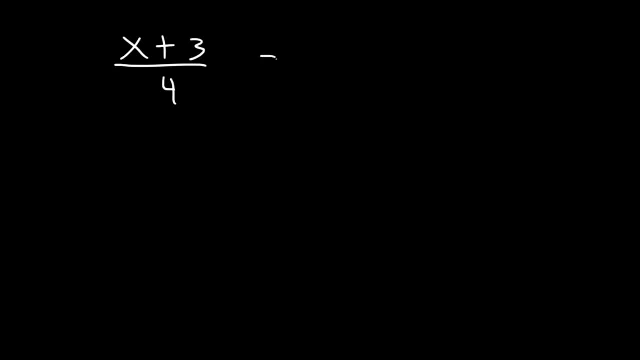 If x plus 3 divided by 4 is equal to 2 over 12, then what is the value of x? Whenever you have two fractions separated by an equal sign, a technique that you can use is cross multiplication. 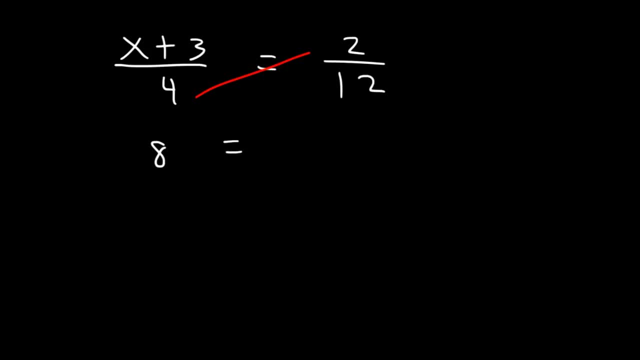 4 times 2 is 8. 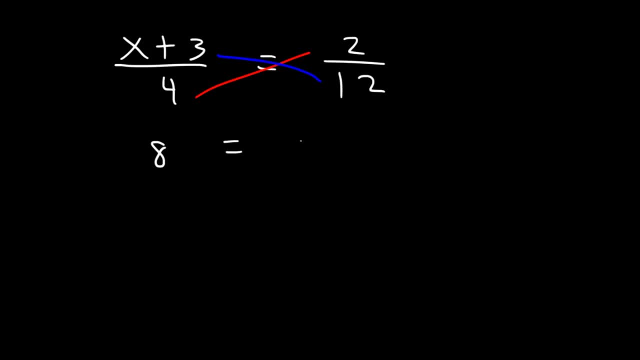 12 times x plus 3 is going to be 12x plus 36. You have to multiply x by 12 and 3 by 12. 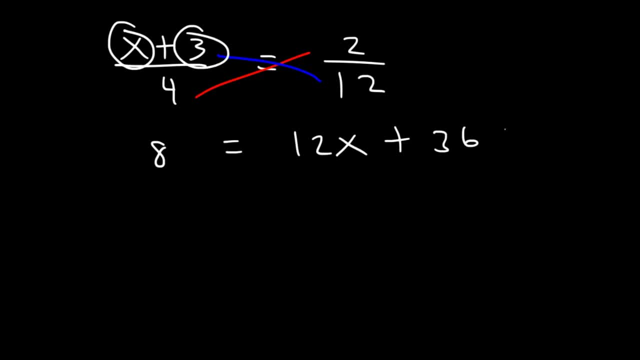 So you need to distribute 12 to x plus 3. At this point, let's subtract both sides by 36. 8 minus 36 is negative 28. 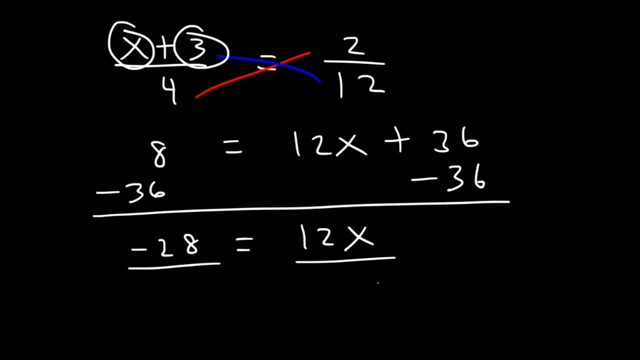 And that's equal to 12x. Now our next step is to divide both sides by 36. We are going to divide both sides by 12. 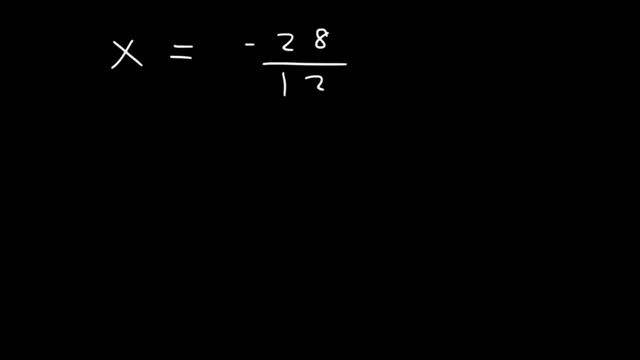 So x is equal to negative 28 divided by 12. So we have a fraction. Whenever you get a fractional answer, you want to check to see if you can reduce it. 28 and 12 are both divisible by 4. 28 divided by 4 is 7. So negative 28 over 4 is 7. 12 divided by 4 is 3. 28 divided by 4 is 7. 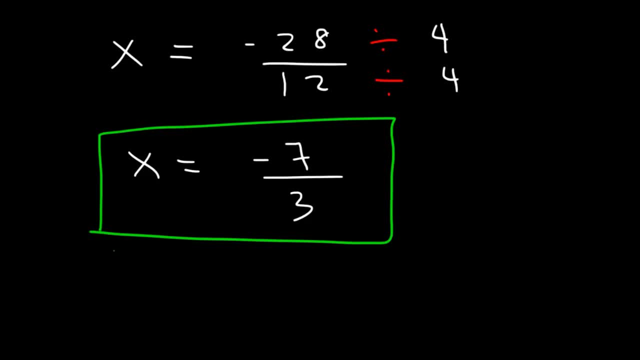 So therefore, x is equal to negative 7 divided by 3. 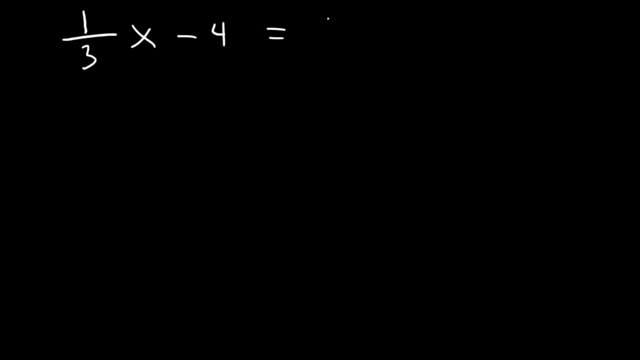 Here's another problem, one that has multiple fractions. Go ahead and find the value of x. In a situation like this, it's best to try to clear away the fractions. So you want to multiply it by a number that's going to get rid of the 1 3rd and the 2 5ths. So you need to multiply everything that is a multiple of 3 and 5. A multiple of 3 and 5 is 15. 3 times 5 is 15. Let's multiply everything by 15. So 15 times 1 3rd x, that's the same as 15 divided by 3 times x. 15 divided by 3 is 5. So this becomes 5x. 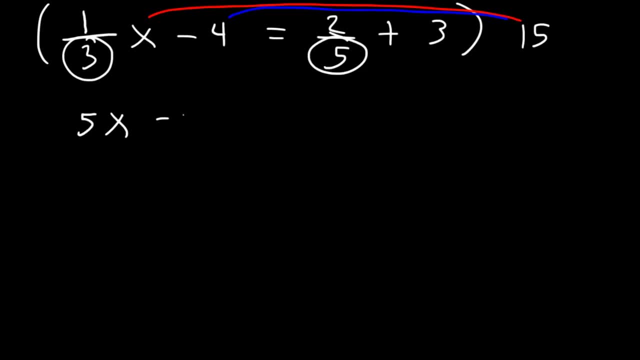 15 times negative 4 is negative 60. Now what is 2 5ths of 15? 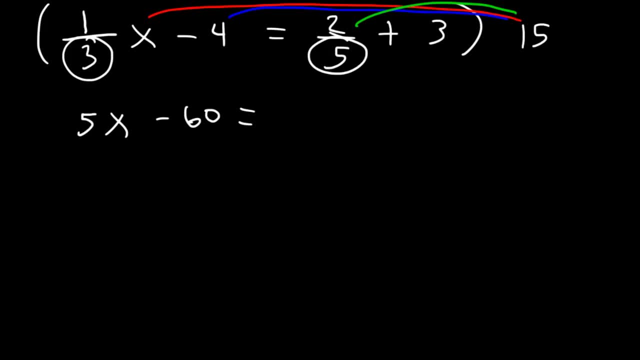 15 times 2 is 30. 30 divided by 5 is 6. 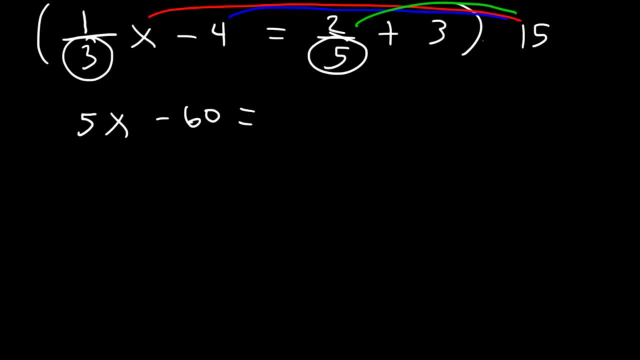 You can also do it this way. 15 divided by 5 is 3. 3 times 2 is 6. Sometimes it's easier to divide first and then multiply. Now 15 times 3 is 45. 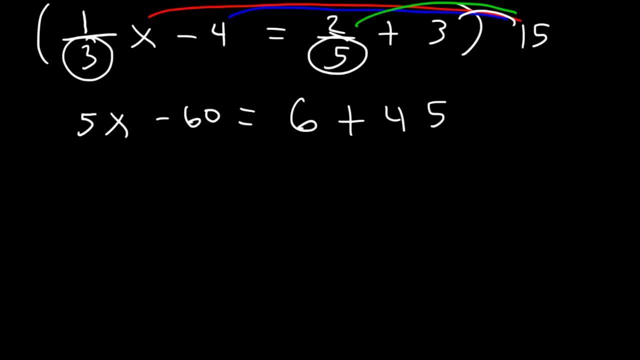 As you can see, this is a lot easier to solve. 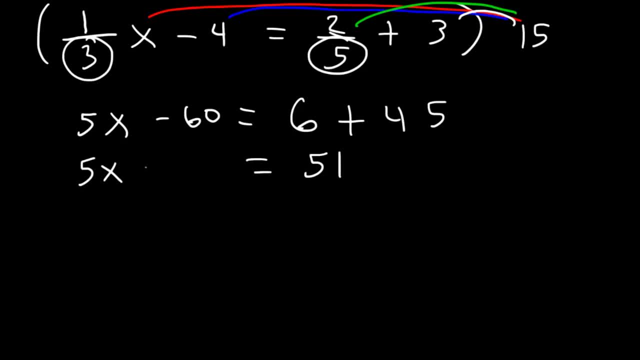 6 plus 45 is 51. Now our next step is to add 60 to both sides. Our goal is to get x by itself. 51 plus 60 is 111. So now we just have to divide both sides by 5. So x is equal to 111 divided by 5. And if we want to, we can divide both sides by 5. We can convert this into a mixed number. 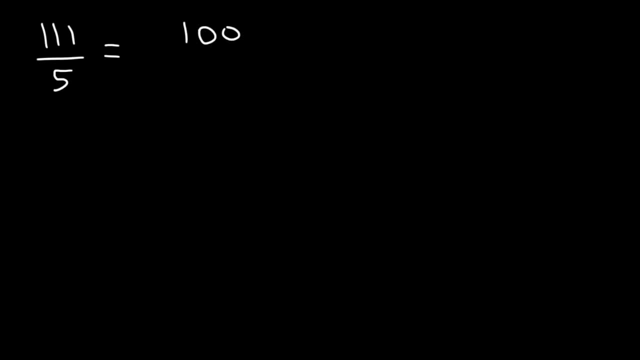 So 111, I'm going to break that into 100 plus 10 plus 1. And divide each number by 5. 100 divided by 5 is 20. 5 $20 bills make up 100. 10 divided by 5 is 2. And then we have plus 1 5th, which we can't reduce. 20 plus 2 is 22. So therefore, 111 over 5, which is an improper fraction, is equivalent to 22 and 1 5th, which is a mixed fraction or a mixed number. Now sometimes, 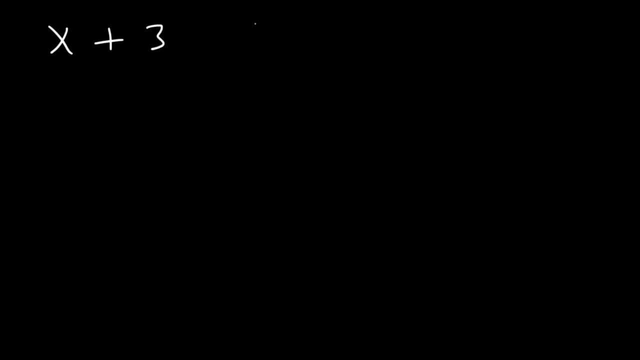 you may have to solve linear inequalities. And here's an example. Let's say that x plus 3 is greater than 5. Whenever you have an inequality, that means x is not just one particular number, but it can represent a range of numbers. For example, x can be equal to 4. 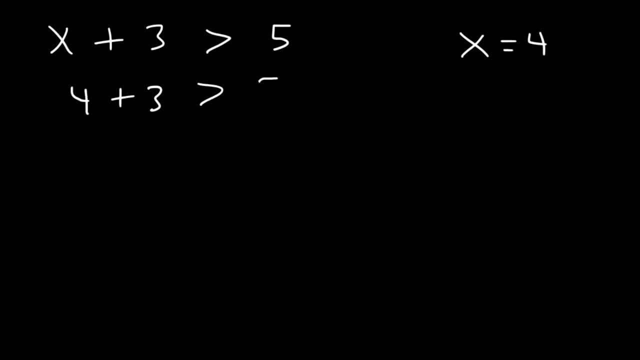 Because 4 plus 3 is greater than 5. 4 plus 3 is 7. 7 is larger than 5. x can be equal to 3. 3 plus 3 is still greater than 5. However, x cannot be equal to 2. Because 3 plus 2 is not greater than 5. Rather, it equals 5. So whenever you're dealing with inequalities, you need to realize that x is no longer a single number, but it is an integral number. 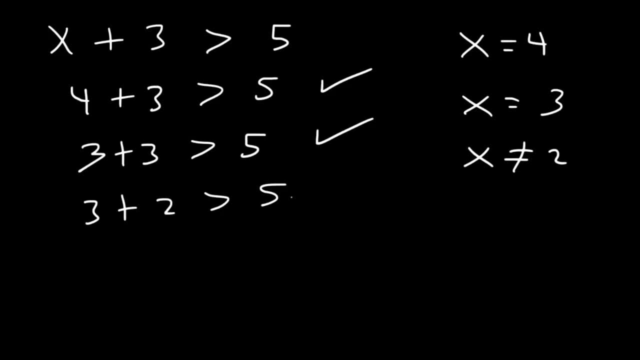 But it could represent a range of numbers. x can be 3.5, 8, 10. So how can we describe the solution that represents the value of x? 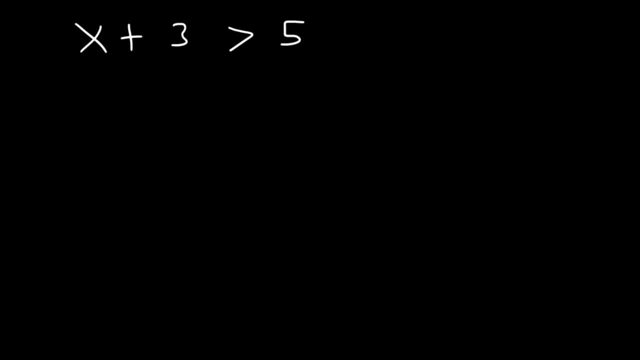 So what you would do is solve it as any typical equation. Let's subtract both sides by 3. 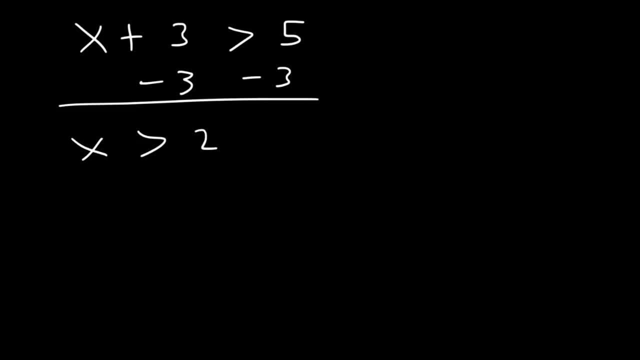 So 5 minus 3 is 2. Therefore, the solution is x is greater than 2, but not equal to 2. 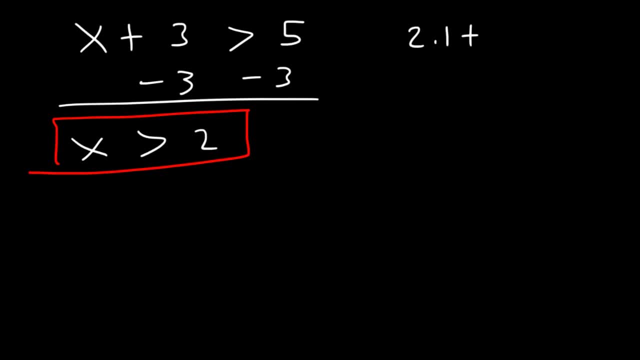 So x can be equal to 2.1. 2.1 plus 3 is greater than 5. Because 2.1 plus 3 is 5.1. And that's larger than 5. 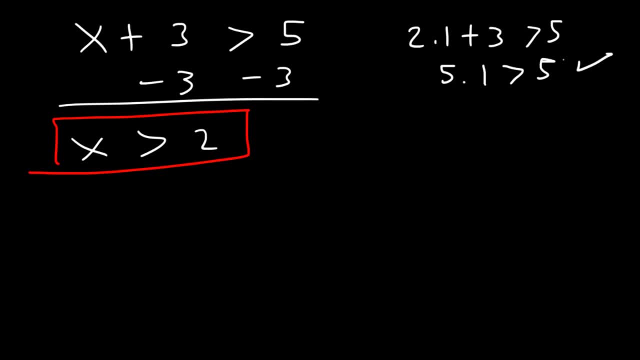 So x can be anything greater than 2. Now sometimes, you may need to 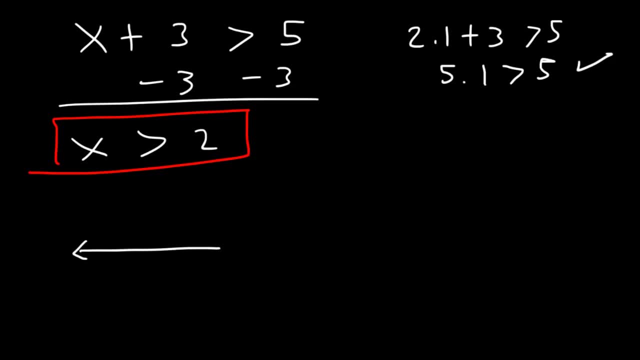 plot the solution on a number line. So how can we do so? Let's say this is 0. And here's 2. 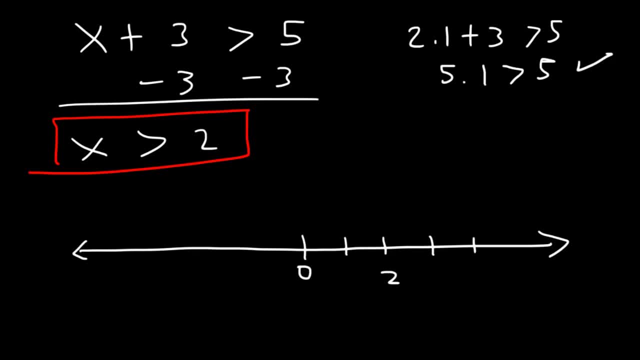 Now x is greater than 2, but does not equal 2. It does not include 2. Because it doesn't include 2, we need to use an open circle. And because x is greater than 2, we need to shade towards the right. If x was less than 2, we need to shade towards the left. 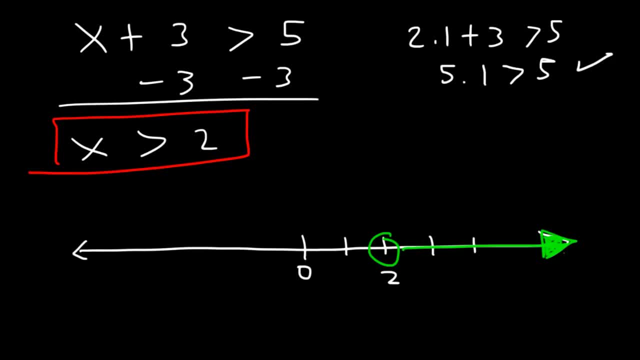 And so that's how you can graph the solution of an inequality 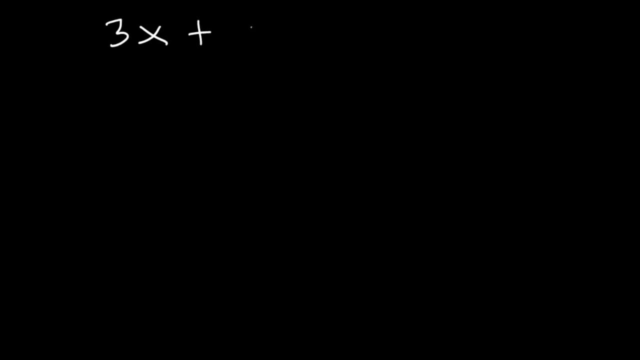 Now let's work on some more examples. Let's say we have this inequality. 3x plus 4 is less than or equal to 10. Solve the inequality and graph it on a number line. 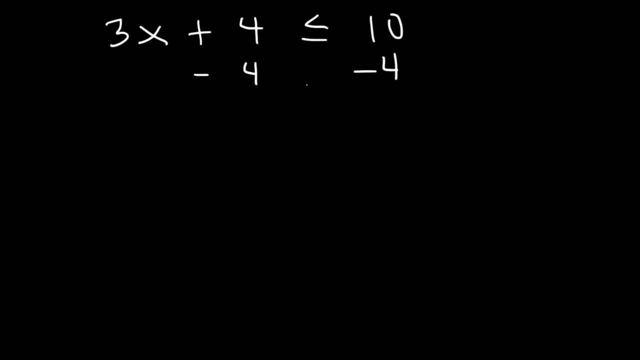 So let's begin by subtracting both sides by 4. 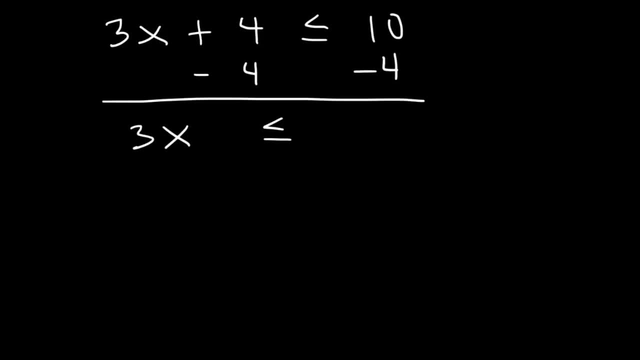 So 3x is less than or equal to 10 minus 4, which is 6. 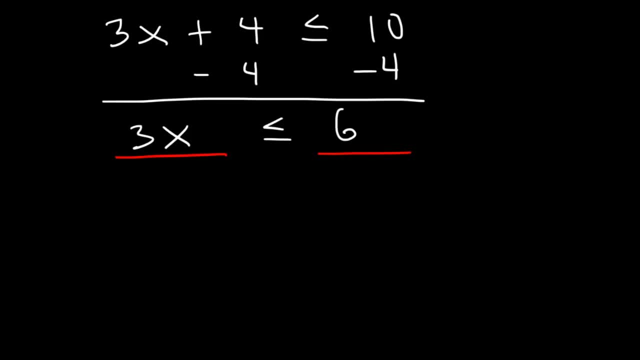 Now our next step is to divide both sides by 3. 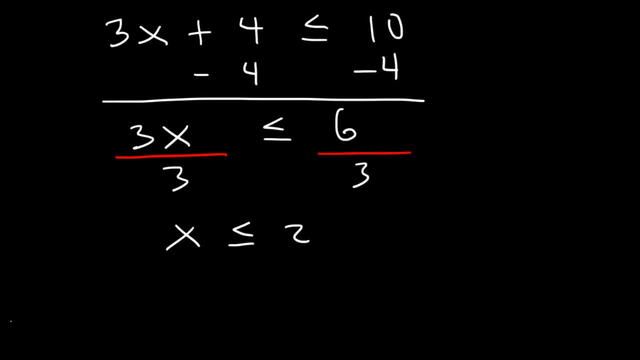 6 divided by 3 is 2. So x is less than or equal to 2. 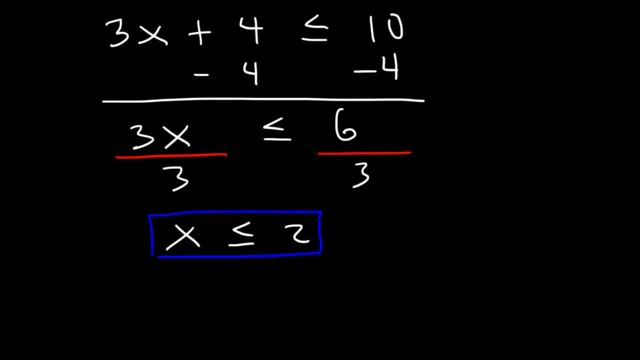 So how can we graph the solution on a number line? So here's 2. 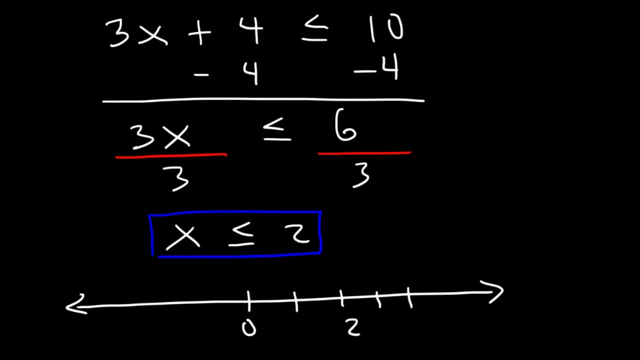 Because it's equal to or less than, we need to use a closed circle as opposed to an open circle. So anytime you see an underline here, use a closed circle. 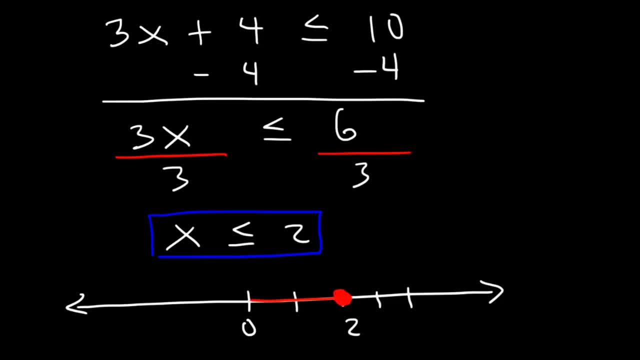 Because it could be less than 2, we need to shade towards the left. If it was greater than, we would shade towards the right. So that's how you can graph the solution on a number line. Here's another one that you can try. 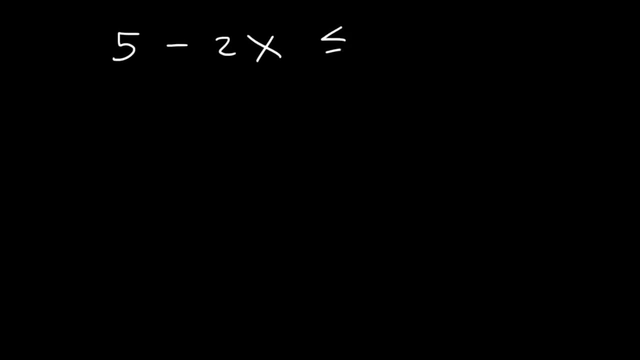 Let's say that 5 minus 2x is less than or equal to 3. 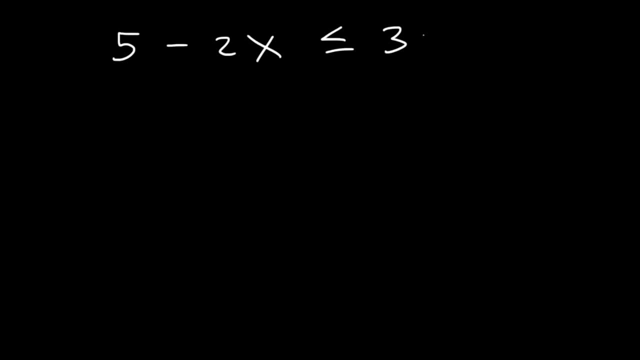 Feel free to pause the video and work on this example. So go ahead, take a minute and try it. 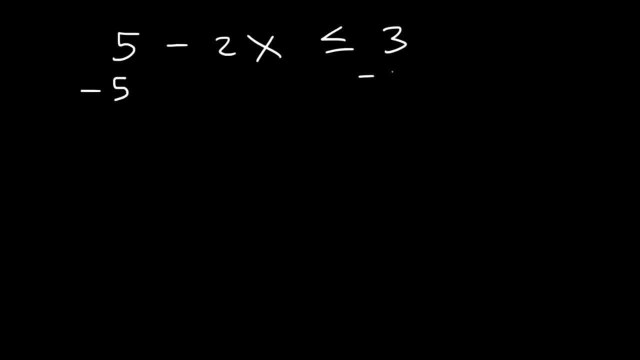 So let's begin by subtracting both sides by 5. 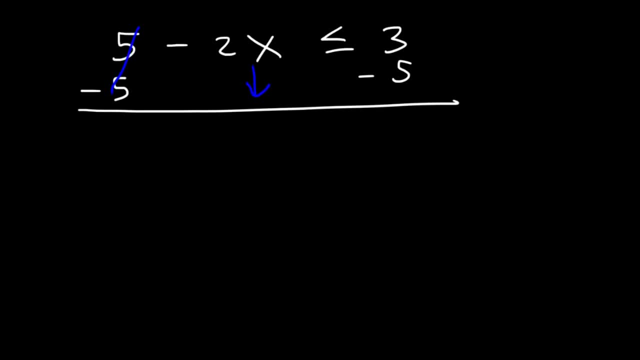 So these numbers will cancel. Let's bring down the negative 2x. So negative 2x is less than or equal to 3 minus 5, which is negative 2. Now our next step is to divide both sides by negative 2. 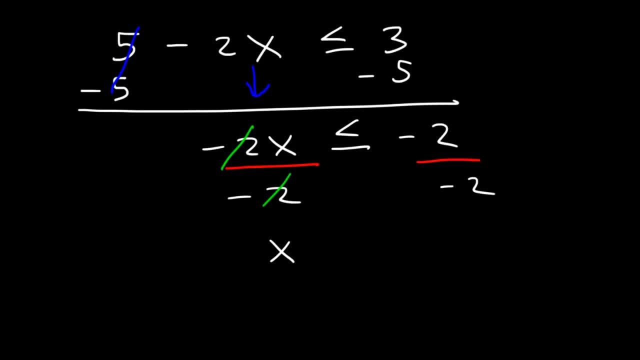 So we can cancel these numbers. Now this is something important that you want to keep in mind. 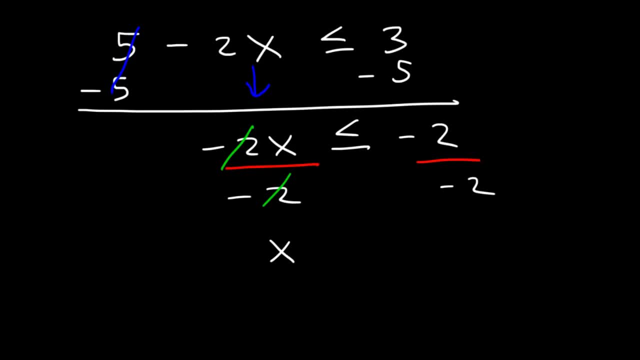 Whenever you multiply or divide by a negative number, the direction of the inequality changes. 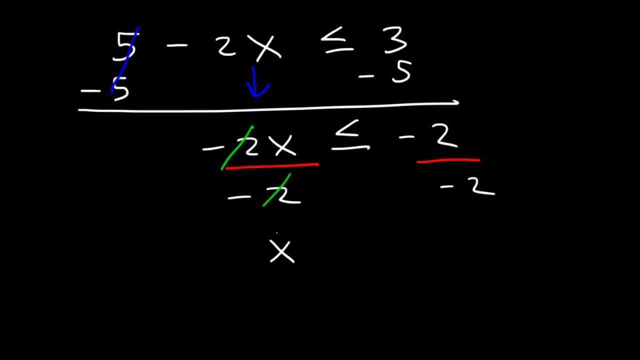 So here, it's to the left, the arrow. It's less than or equal to. Now it's going to be greater than or equal to. 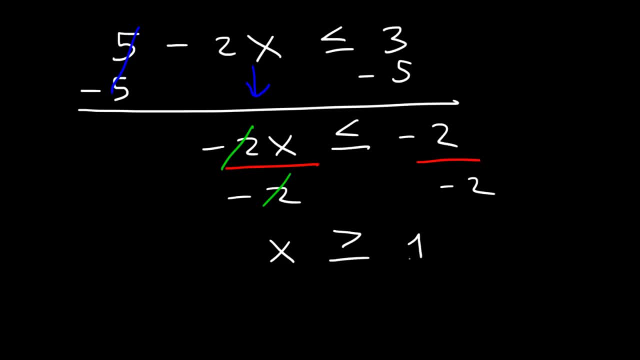 So never forget that point. Negative 2 divided by negative 2 is positive 1. So our answer is x is equal to or greater than 1. 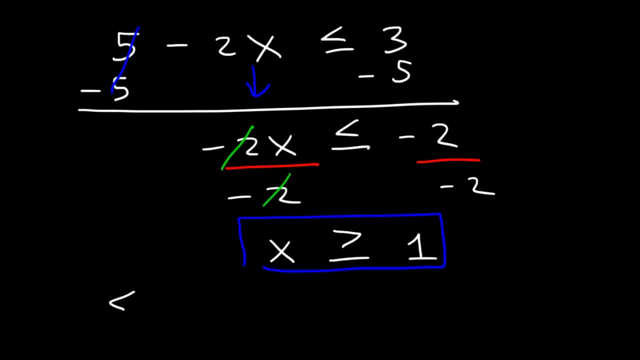 So now let's plot the solution on a number line. 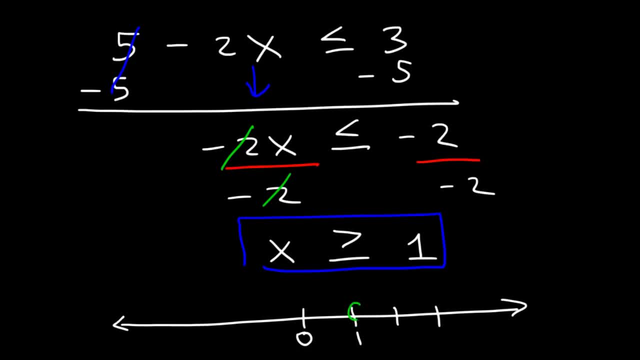 So here's one. And it's going to be a closed circle as opposed to an open circle. Because the solution includes one. And we're going to shade towards the right. So that's the answer. 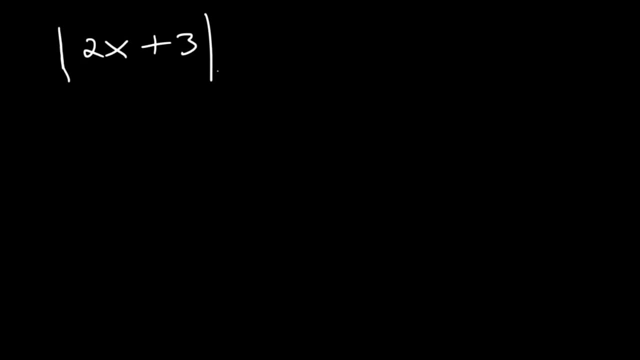 Consider this equation. The absolute value of 2x plus 3 is equal to 11. What is the value of x? So what do we need to do in order to solve an absolute value equation? Well, let's review a few basic things. 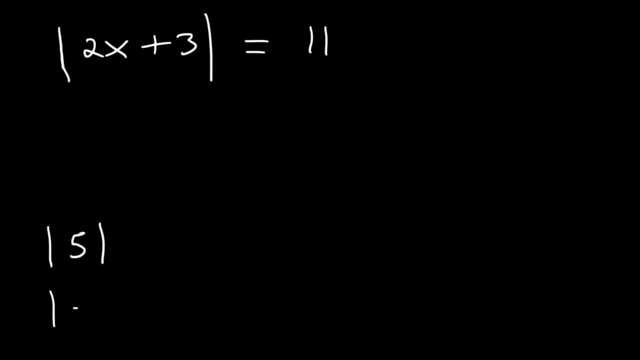 What is the absolute value of 5? And what is the absolute value of negative 5? 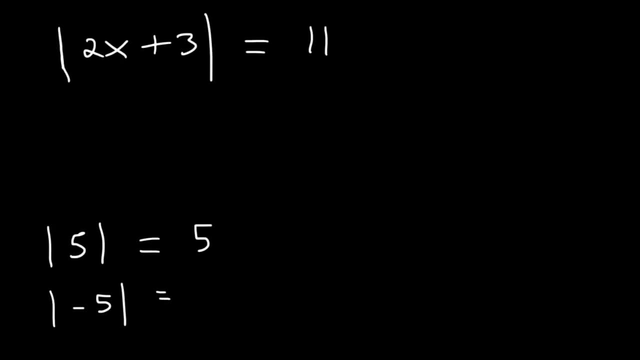 The absolute value of 5 is 5. The absolute value of negative 5 is 5. 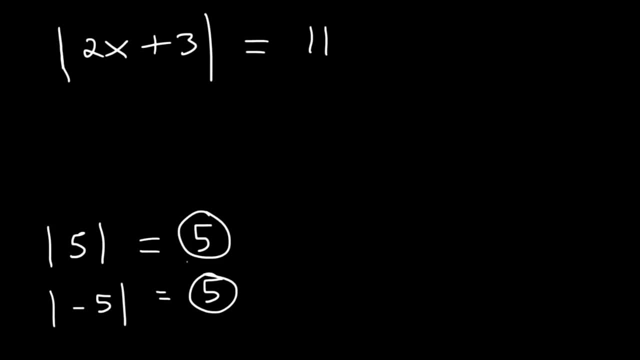 So notice that even though these two values are the same, what's inside is not the same. 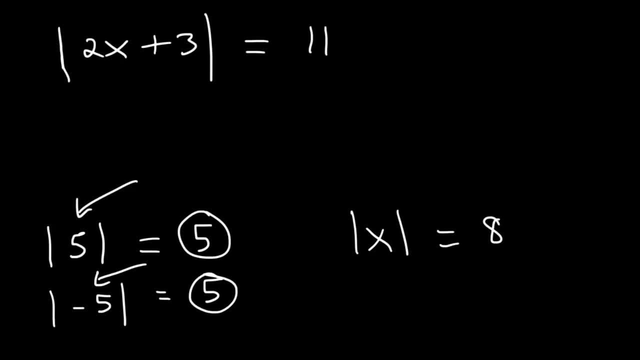 So let's say if the absolute value of x is equal to 8. What is the value of x? x can be two numbers. x is equal to 8 and x is equal to negative 8. Because the absolute value of 8 will give us 8, and the absolute value of negative 8 will give us the same answer, 8. 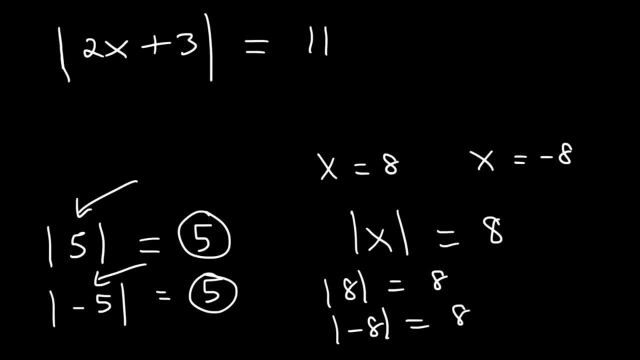 The absolute value function converts any negative values into positive values. 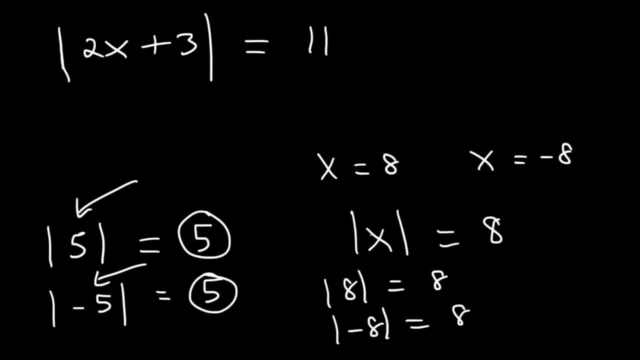 So notice that what's inside is equal to two things. 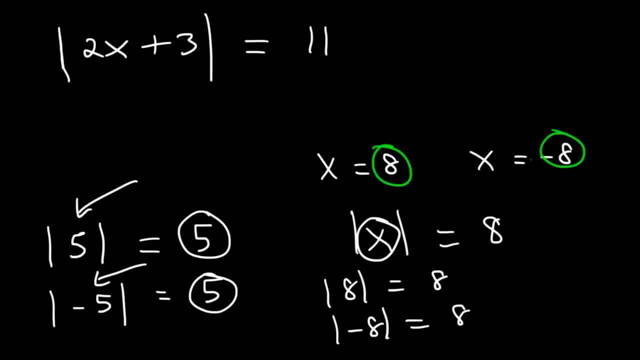 A positive answer and a negative answer. So therefore, we need to use that fact to solve for x in this equation. 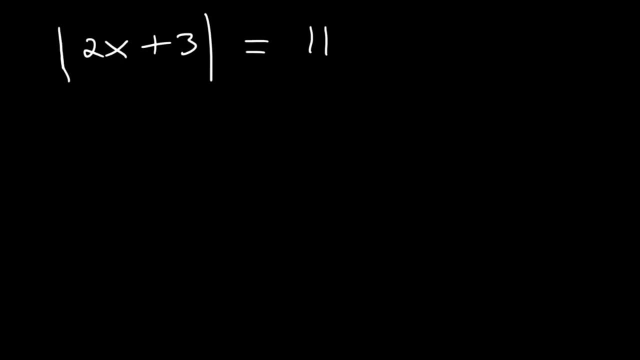 Whenever you want to solve an absolute value equation, to open the absolute value expression, set what's on the inside equal to two things. The original value that you see here, 11, and also negative 11. And the reason for that is because the absolute value of positive 11 and the absolute value of negative 11 is equal to this number, positive 11. 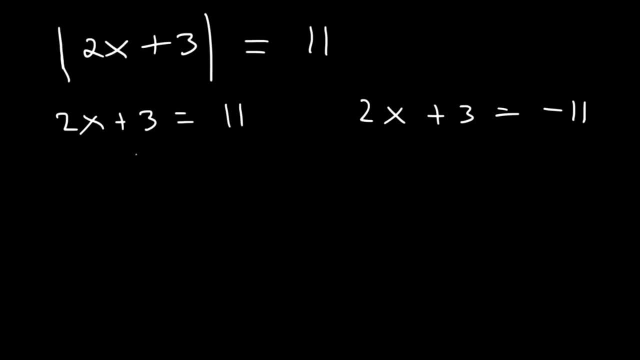 Now let's go ahead and find the value of x. So in the first equation, let's subtract both sides by 3. 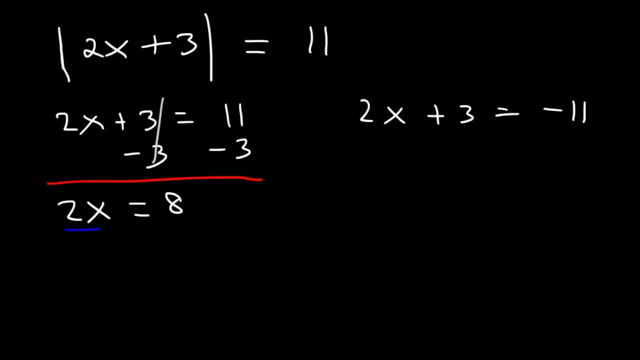 11 minus 3 is 8. Next, let's divide both sides by 2. 8 divided by 2 is 4. 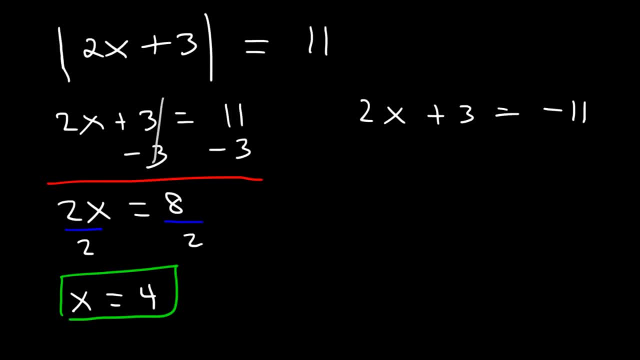 So this is one of the solutions. x is equal to 4. 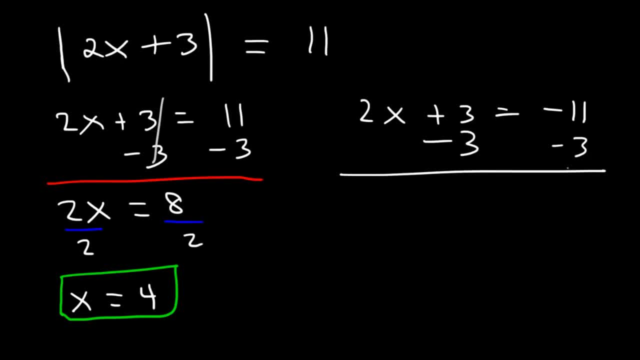 In the next example, let's subtract both sides by 3. Negative 11 minus 3 is negative 14. Next, let's divide both sides by 2. Negative 14 divided by 2 is negative 7. So that's the other answer. 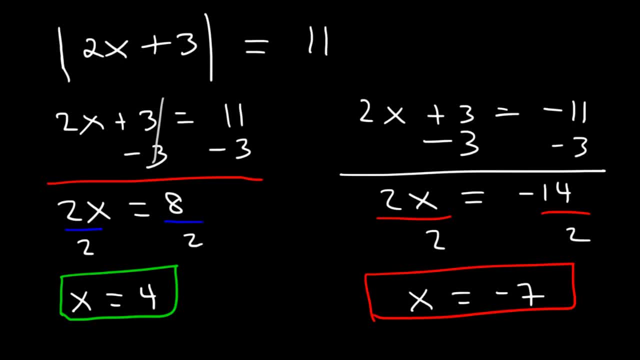 So x can be equal to 4 or negative 7. 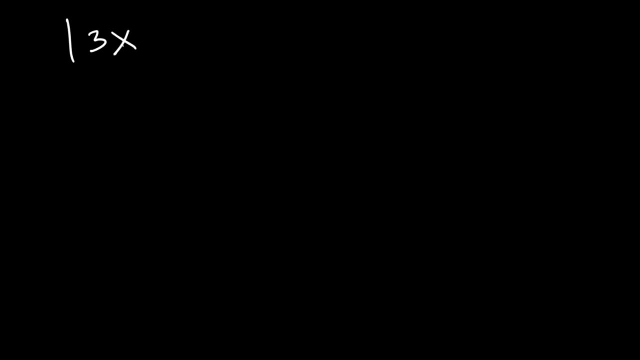 For the sake of practice, work on this example. 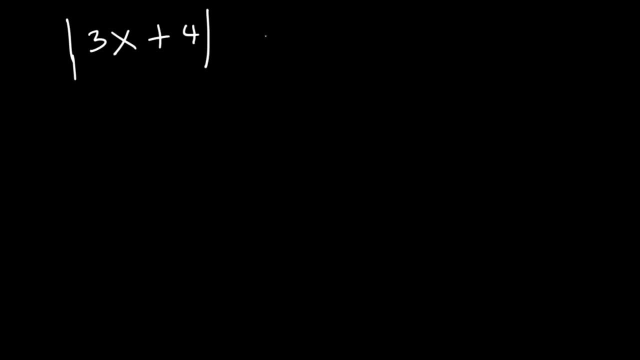 The absolute value of 3x plus 4 is equal to 19. What is the value? So let's write two equations. 3x plus 4 And 3x plus 4 is equal to negative 19. 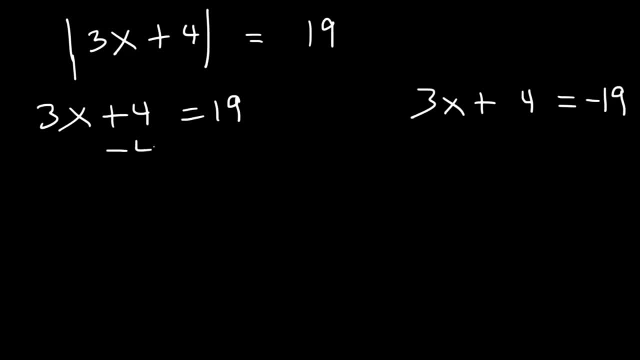 Let's find the value of x. So in the first one, let's subtract both sides by 4. 19 minus 4 is 15. 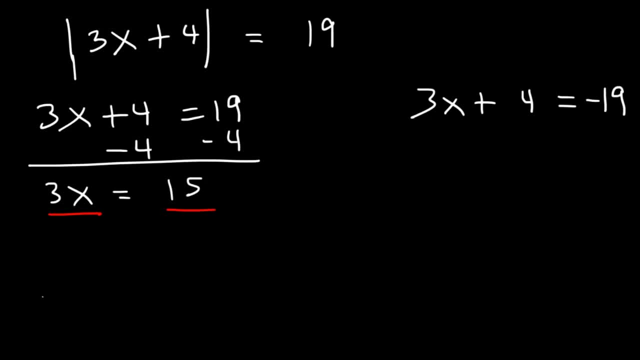 Next, let's divide both sides by 3. 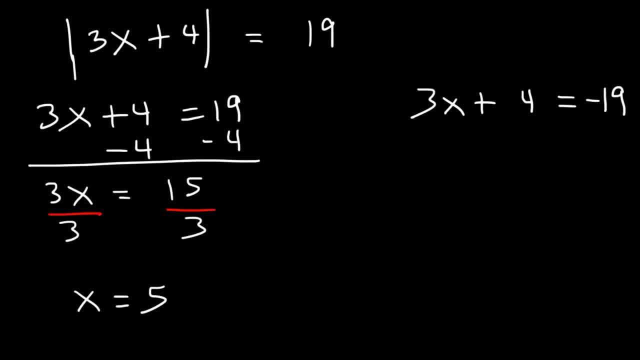 15 divided by 3 is 5. So the first answer is x is equal to 5. 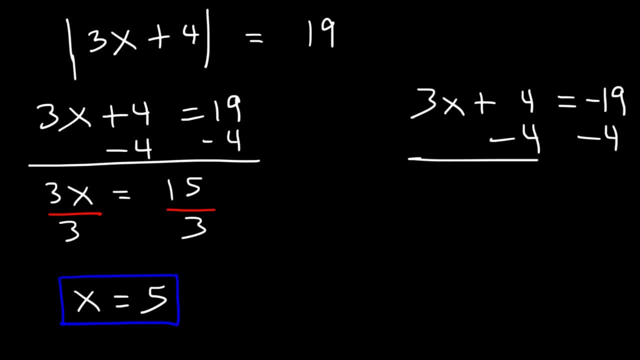 Now let's move on to the other equation. Let's subtract both sides by 4. Negative 19 minus 4 is negative 23. 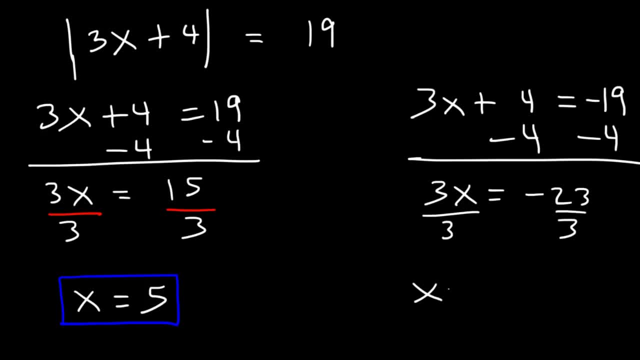 Next, let's divide both sides by 3. So the other answer is negative 23 over 3. We can't reduce that fraction. So we'll leave it like this. 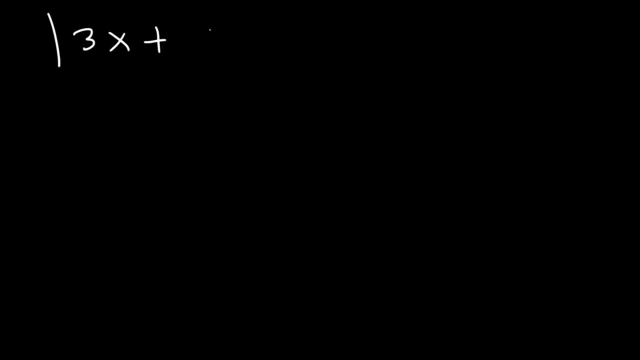 Now sometimes, you might have an equation that contains an absolute value expression along with an inequality. 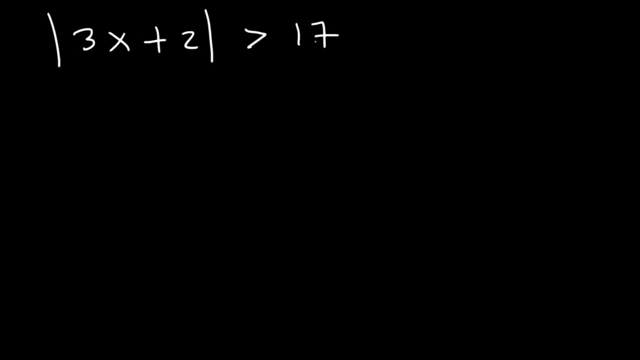 So what do you do in a situation like this? How can you find the value of x? So we're going to write two equations. The first one is going to be the same. Now the second one, there's two things we need to do. First, we need to change the direction of the inequality. 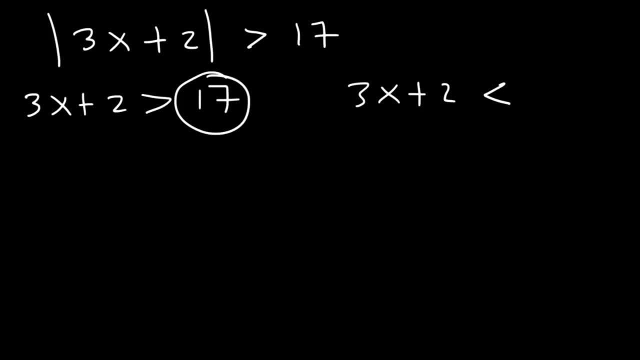 Next, we need to change positive 17 into negative 17. So make sure you make those two changes if you want to get the answer correct. 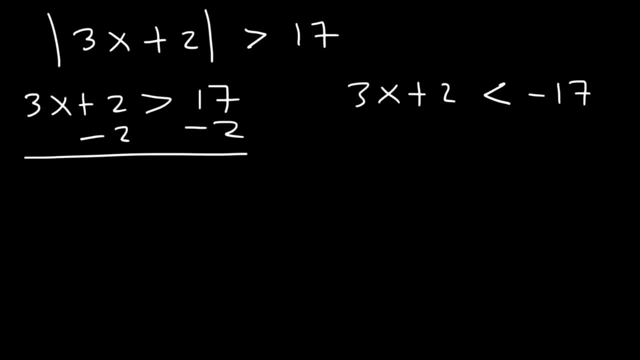 So let's begin by subtracting both sides by 2. 17 minus 2 is 15. Next, let's divide both sides by 3. 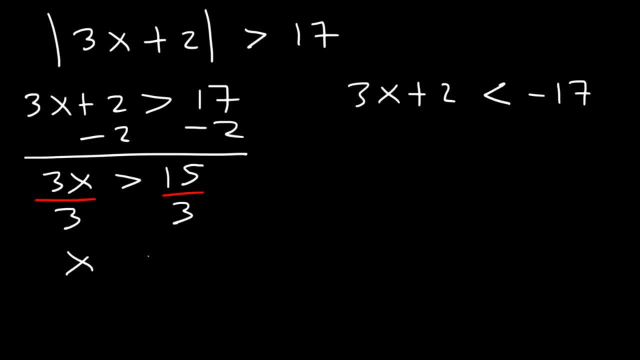 15 divided by 3 is 5. So x is greater than 5. That's the first solution. Now let's move on to the next equation. 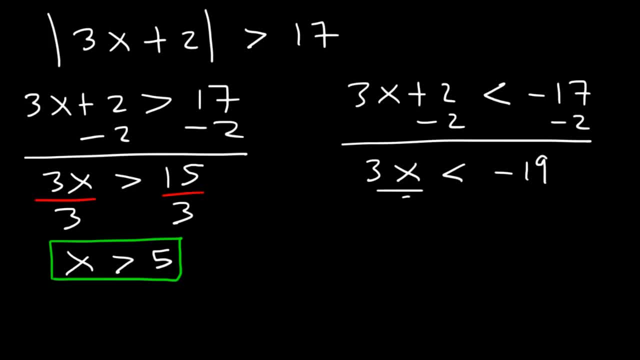 Negative 17 minus 2 is negative 19. If we divide by 3, we can see that x is less than negative 19 over 3. 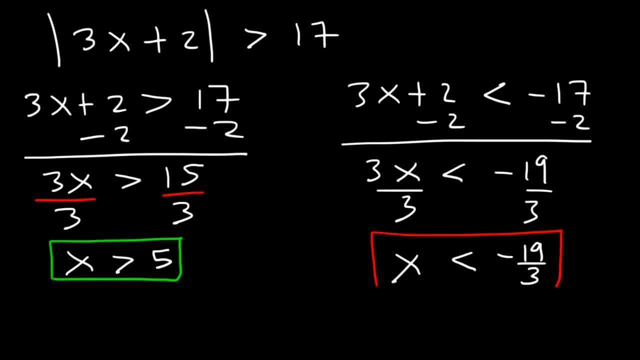 Now because we're dealing with inequalities, let's plot the solution on a number line. 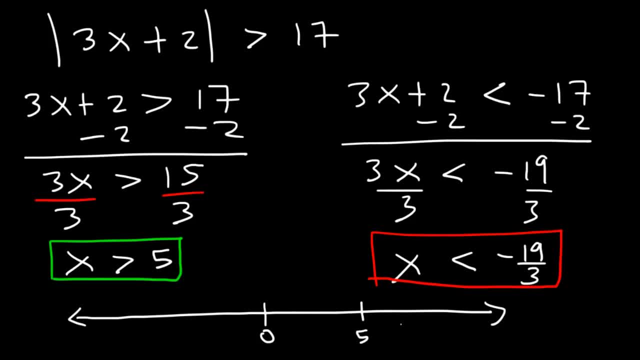 So this is going to be 0. 5 is towards the right. Negative 19 over 3, that's like negative 6.33. So that's going to be somewhere over here. 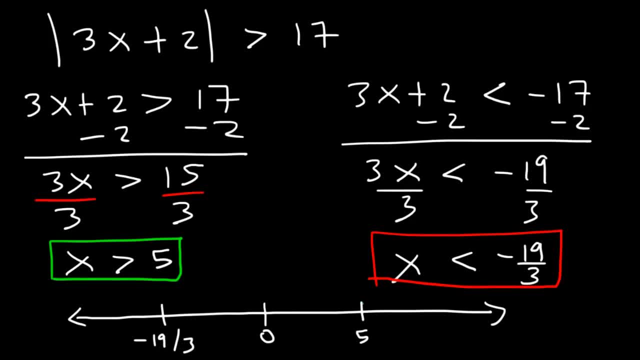 So first, x is greater than 5. 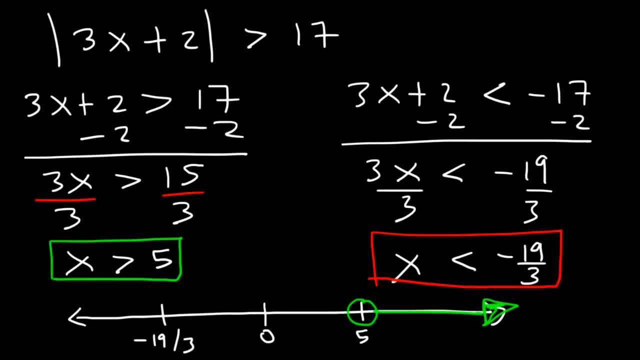 So we have an open circle shaded towards the right. 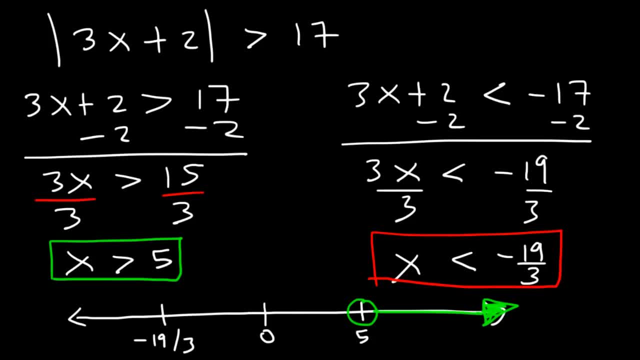 Next, x is less than negative 19 over 3. 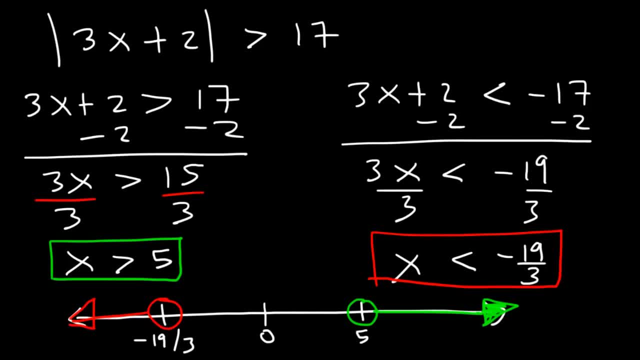 So that's an open circle shaded towards the left. 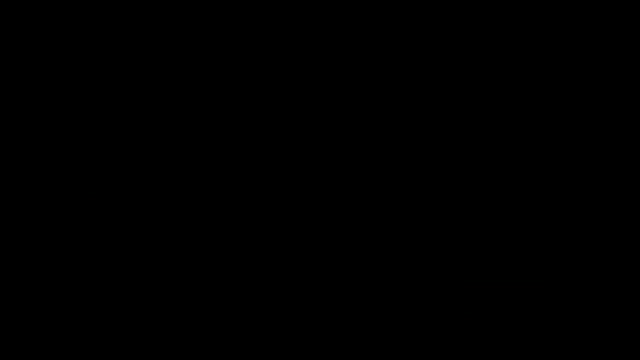 And so that's how you can plot it on a number line. 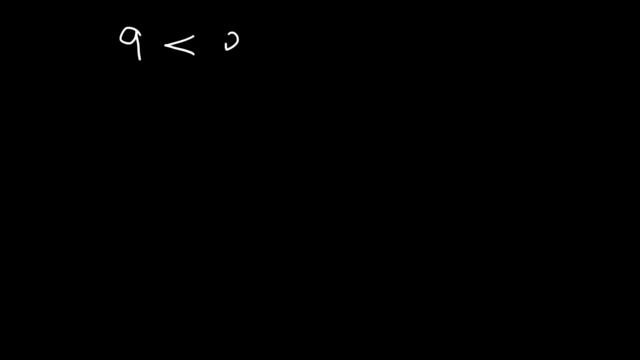 Now what if you were to see an inequality that looks like this? What would you do to solve it? 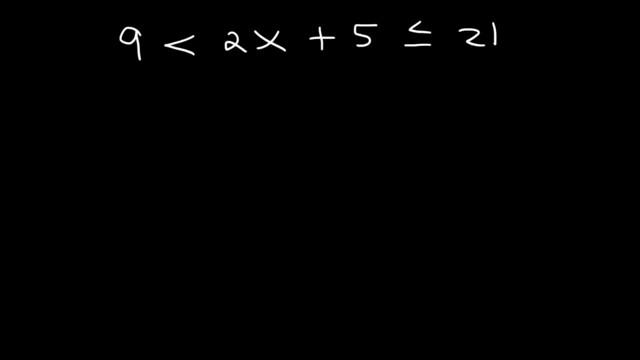 So it looks like there's three parts to the equation. There's three sides to it. The first thing we should do is subtract all three sides by 5. 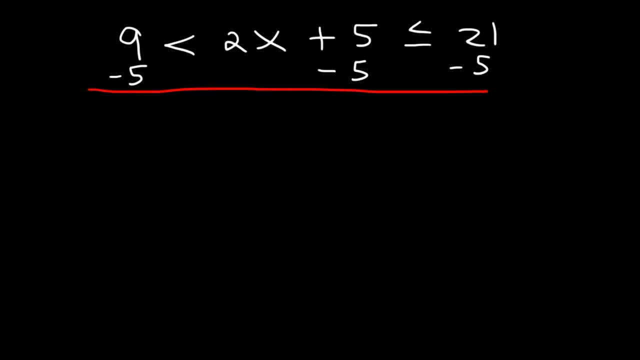 Whatever you do to one side, you must do to the other sides. 9 minus 5 is 4. 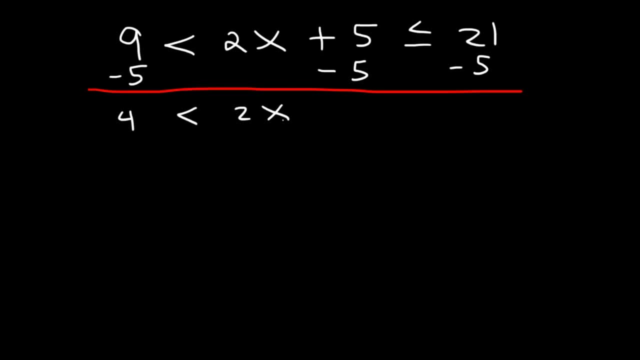 The 2x will remain the same. 5 and negative 5 adds up 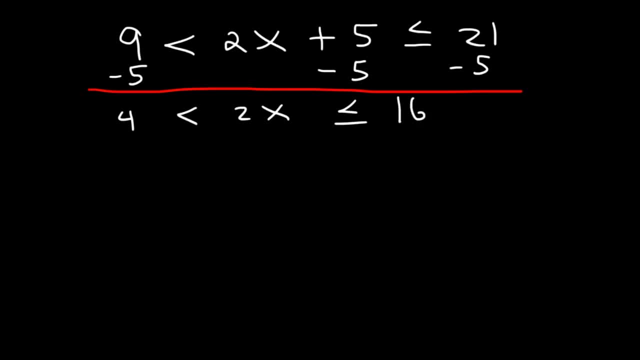 to 0. And 21 minus 5 is 16. 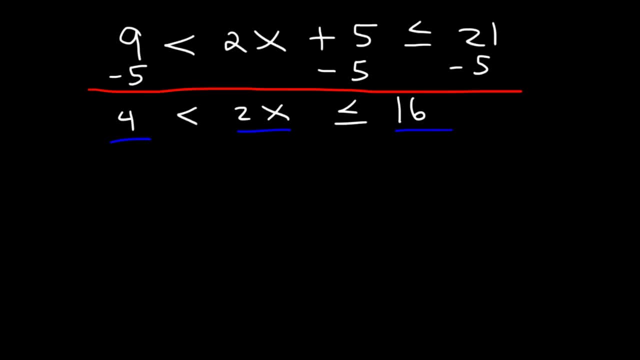 Next, we need to divide all three terms by 2 to get x by itself. 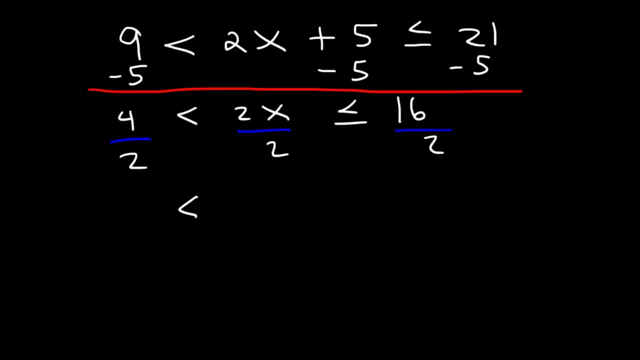 So 2x divided by 2 is just x. 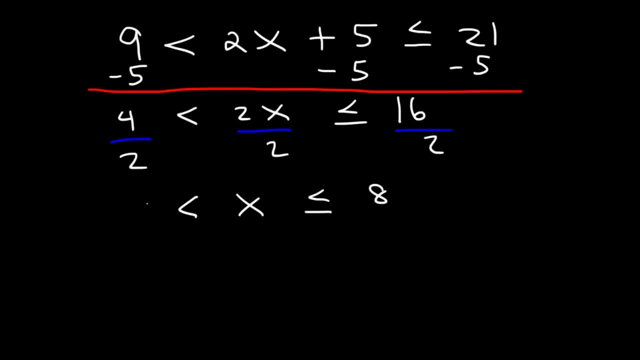 16 divided by 2 is 8. 4 divided by 2 is 2. 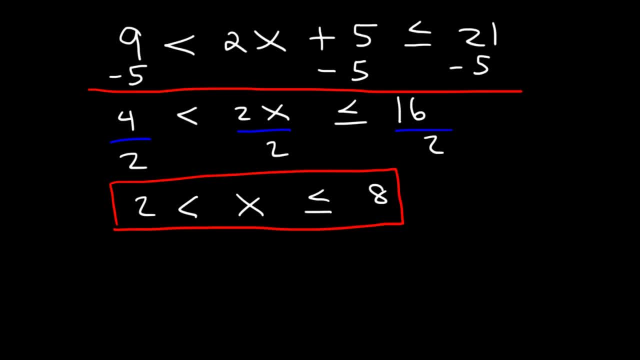 So we can see that x is between 2 and 8. 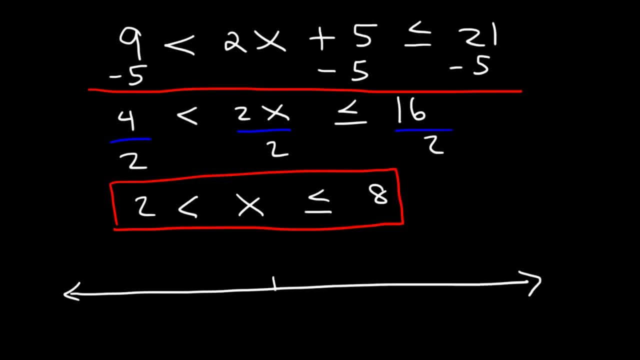 Now how can we plot the solution on a number line? So let's say 2 is over here and 8 is over there. 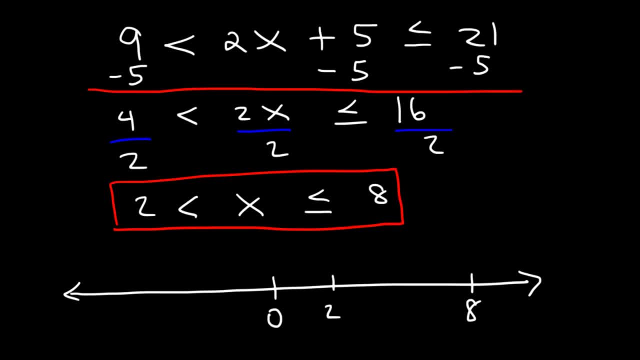 So if we look at the first part, x is greater than 2. 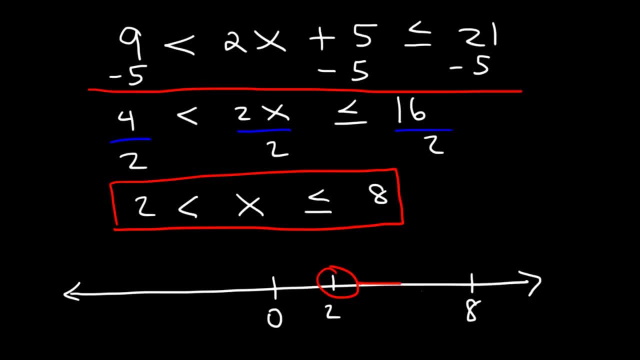 So we have an open circle shaded towards the right. 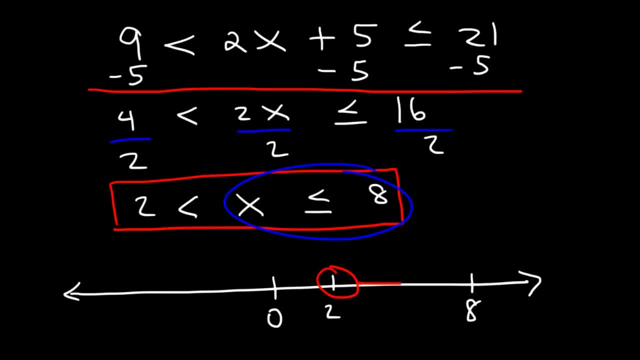 Now looking at the second part, x is less than or equal to 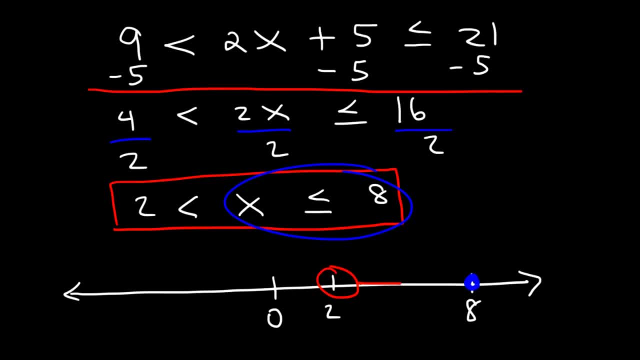 8. The closed circle, and because it's less than, is shaded towards the left. 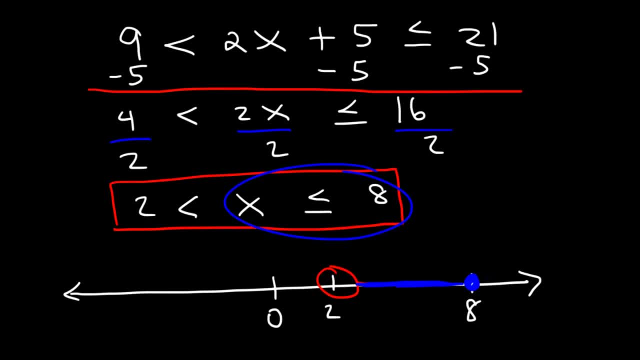 So notice that x is between 2 and 8. It includes 8, but it does not include 2. 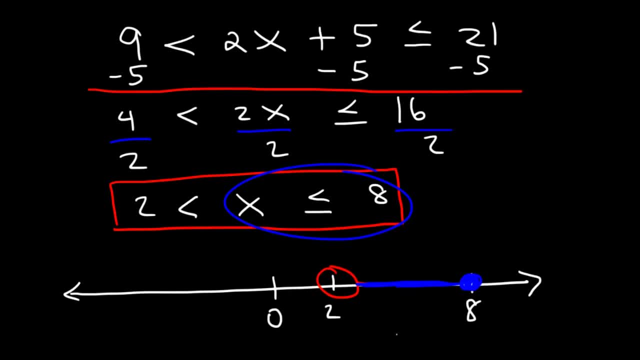 Now if you want to write the answer using interval notation, here's what you do. It's going to be parentheses 2 comma 8. 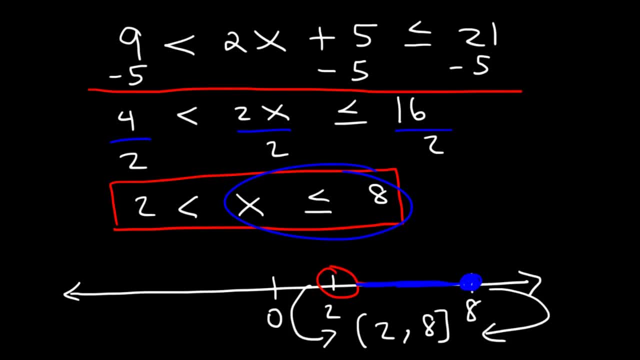 So it's from 2 to 8. The open circle is associated with the parentheses. 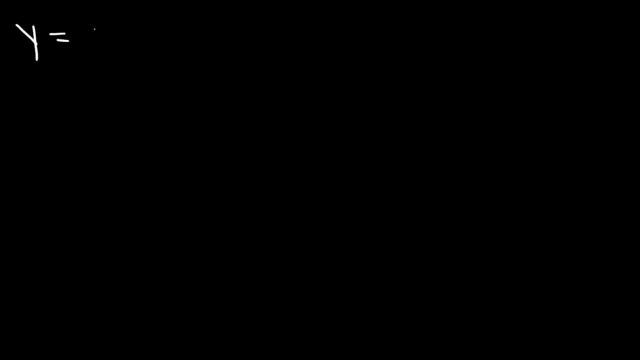 Now let's talk about how to graph linear equations. Let's start with this one. y is equal to 2x minus 3. Now this equation is in slope intercept form. 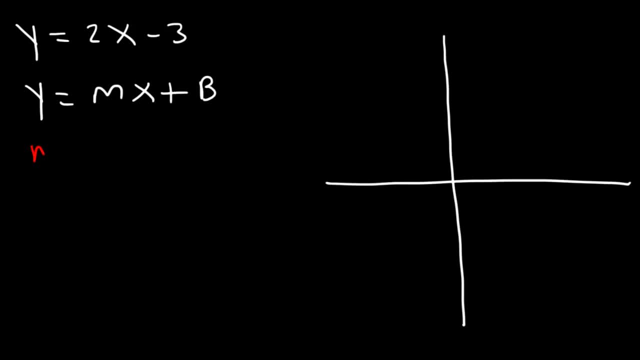 The slope, m, is the number in front of x. m is equal to 2 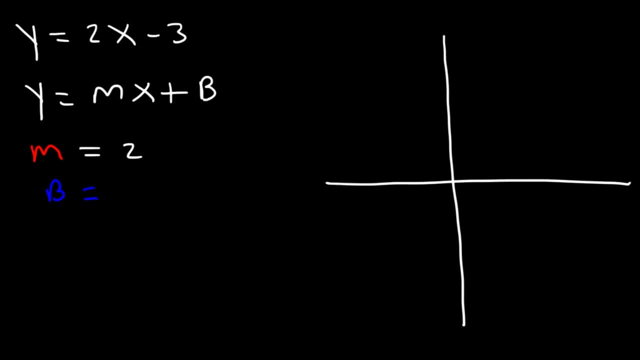 and b is equal to 3. 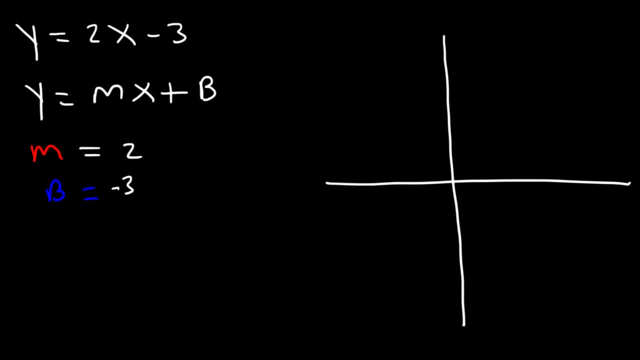 Well, negative 3 technically. b is the y intercept. 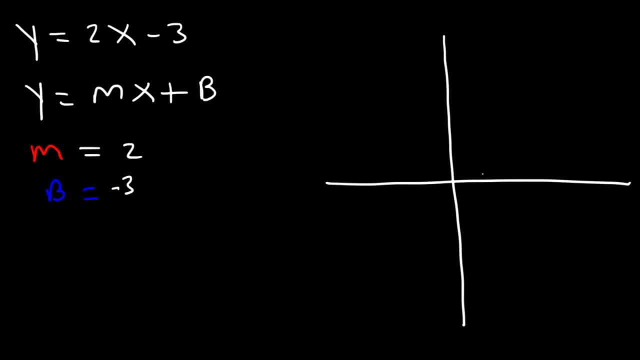 So to graph it using the slope intercept method, plot the y intercept, which is at negative 3. 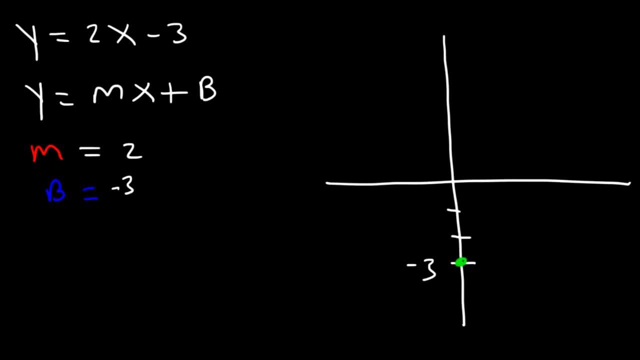 And then use the slope to find the other points. So the slope, which is 2, you can see it as 2 over 1. 2 represents the rise. 1 is the run. So we need to travel up 2 units and 1 to the right. So this will give us the next point. 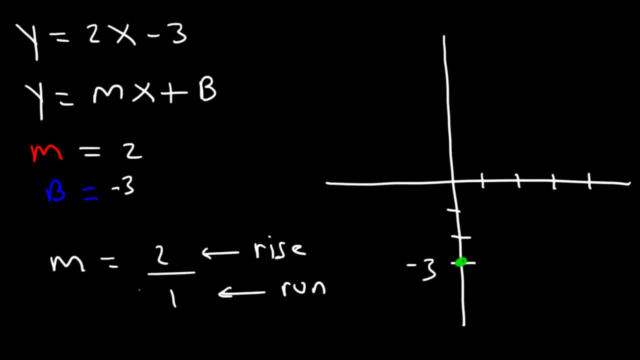 Which is at 1 negative 2. 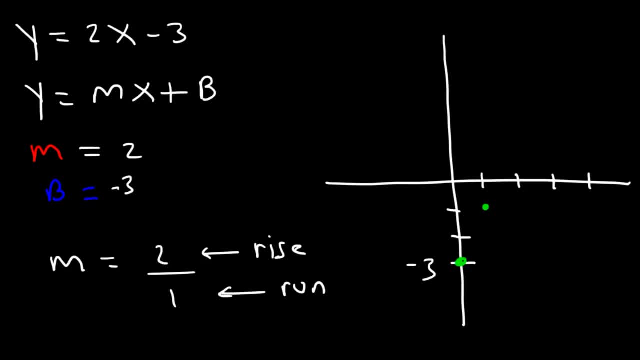 I mean 1 negative 1, I take that back. Not 1 negative 2. 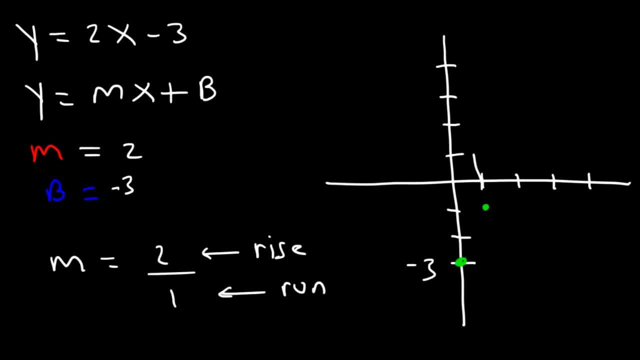 And then if we travel 1 unit to the right, we need to go up 2 again. So then we can get the next point, which is at 2 comma 1. 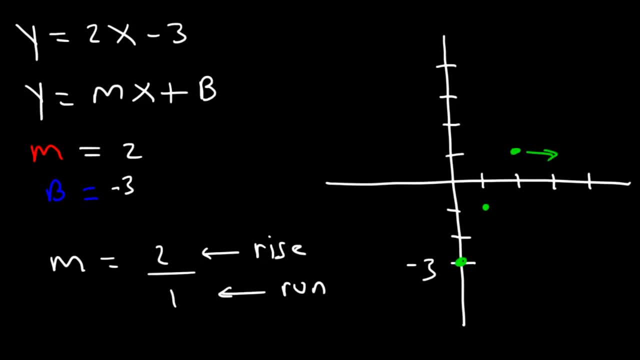 And then we can repeat the process. Travel 1 unit to the right, up 2. 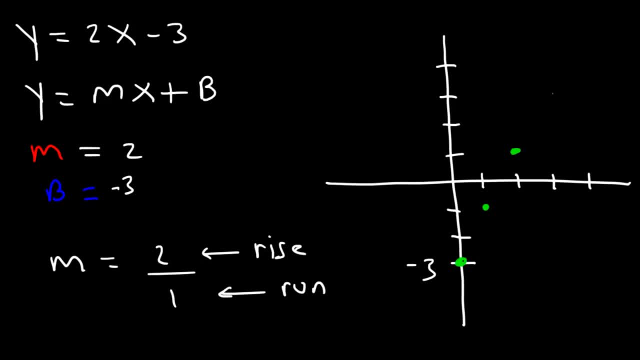 And that will take us to the next point, which is 3, 3. 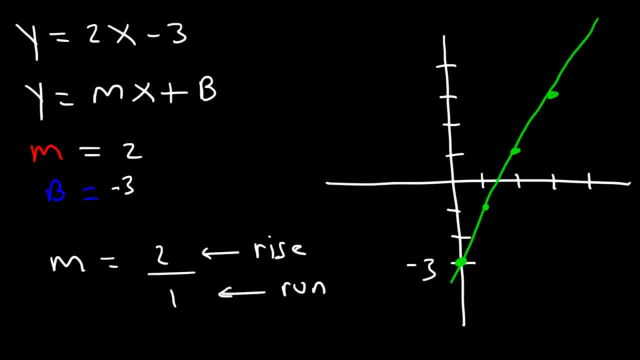 And eventually we can connect these points with a straight line. So that's how you can graph a linear equation using the slope intercept method. 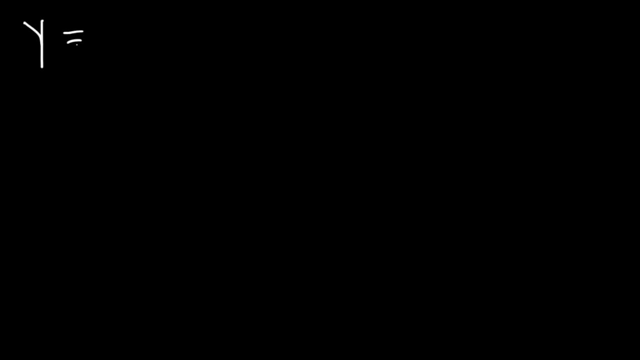 Let's try another example. Go ahead and 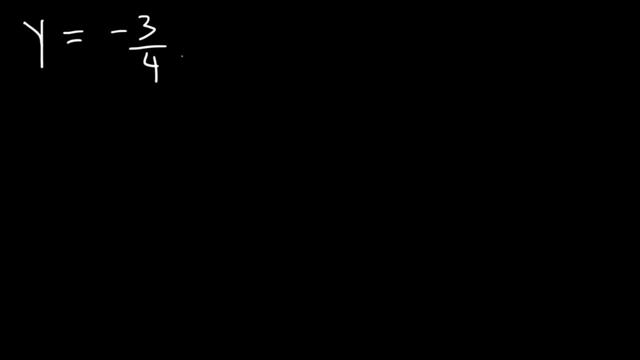 graph the linear equation. Let's say y is equal to negative 3 over 4 x plus 5. So first we gotta find the slope and the y-intercept. The slope is the number in front of x. 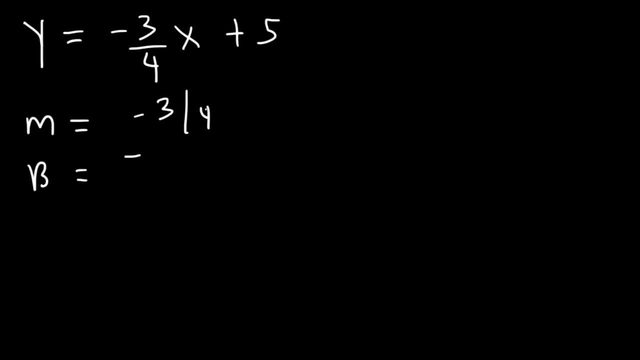 In this case, it's negative 3 over 4. The y-intercept is 5. So let's plot the y-intercept. 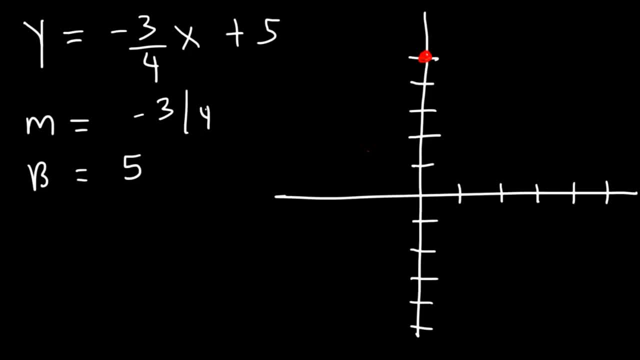 Now let's use the slope to get the next point. The rise is negative 3. The run is 4. 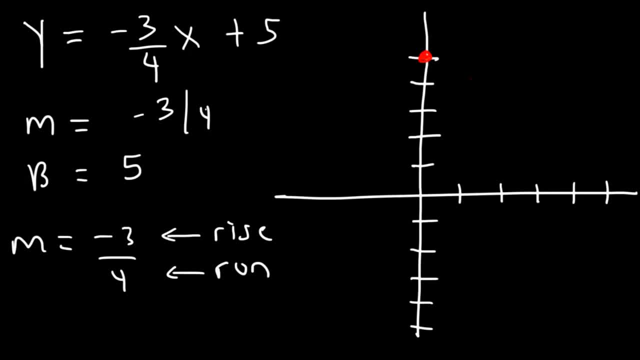 So because the rise is negative, we need to go down 3 units. 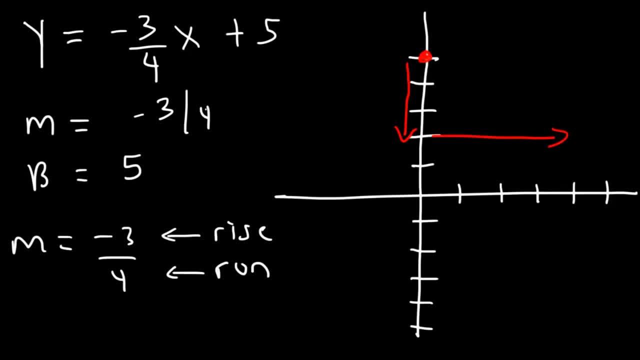 And the run is 4, so we gotta travel 4 units to the right. 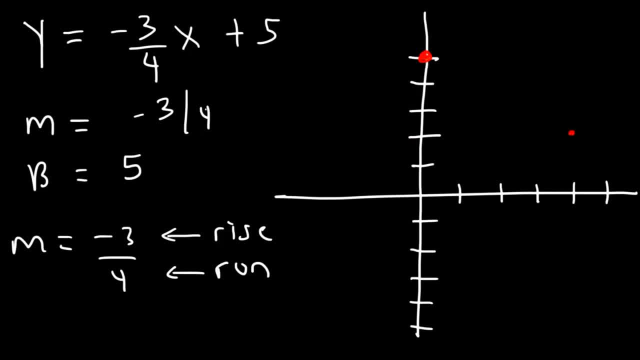 So this will give us the next point, which is at 4 comma 2. x is 4 when y is 2. 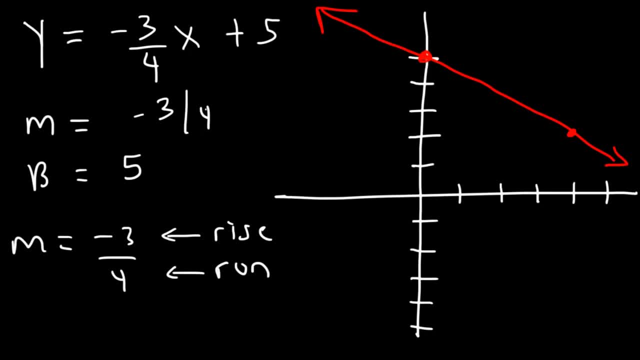 And then we could connect those points with a line. So that's how you can graph that particular linear equation. 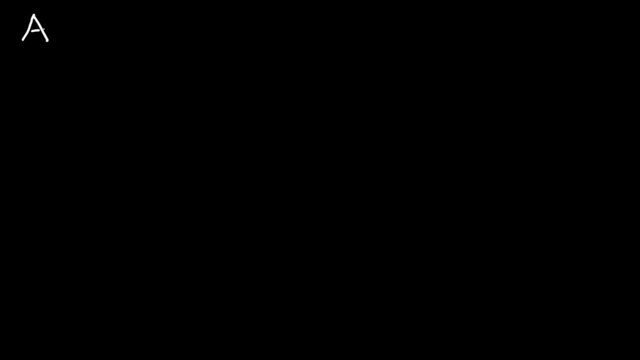 Now sometimes, you might have a linear equation in standard form. Standard form is ax plus by is equal to c. 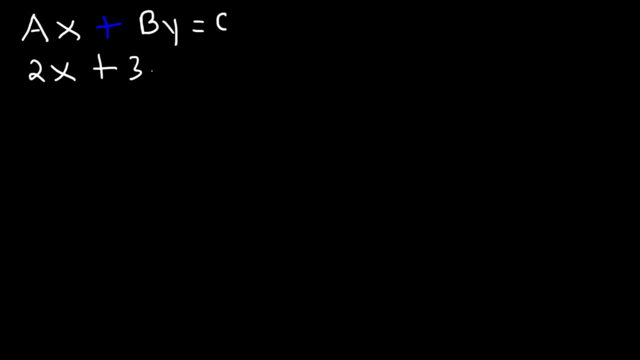 So let's say that 2x plus 3y is equal to 6. 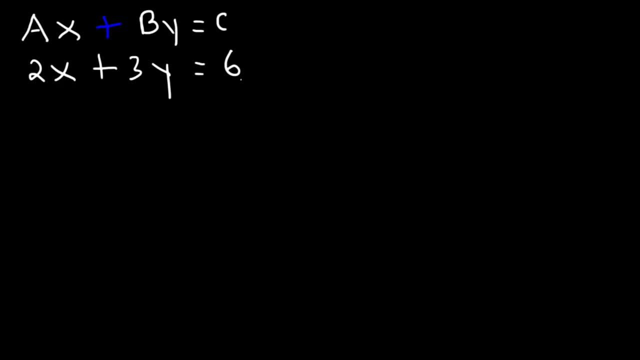 What can we do in order to graph this particular linear equation? 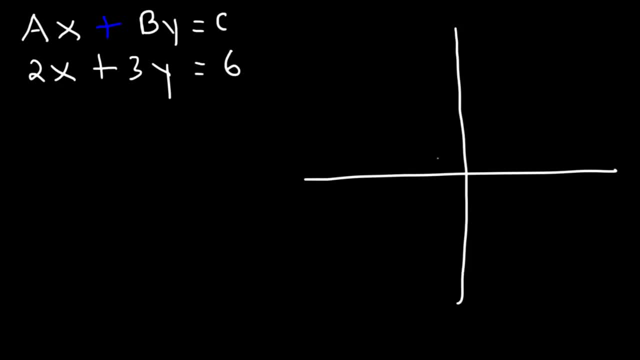 What I like to do is I like to find the x and y-intercepts. To find the x-intercept, replace y with 0. 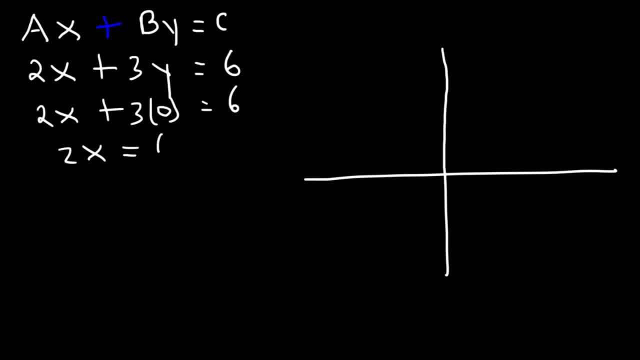 3 times 0 is 0. So therefore 2x is equal to 6. And 6 divided by 2 is 3. 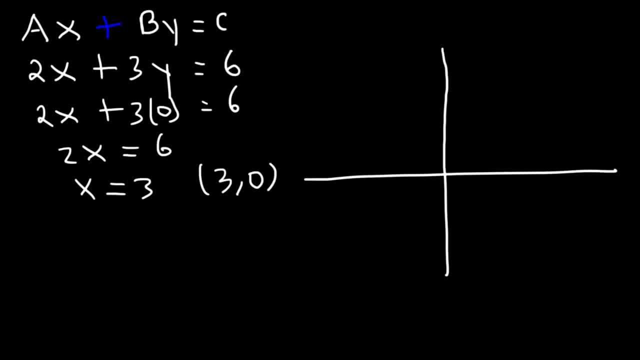 So the x-intercept is 3. The point is 3 comma 0. 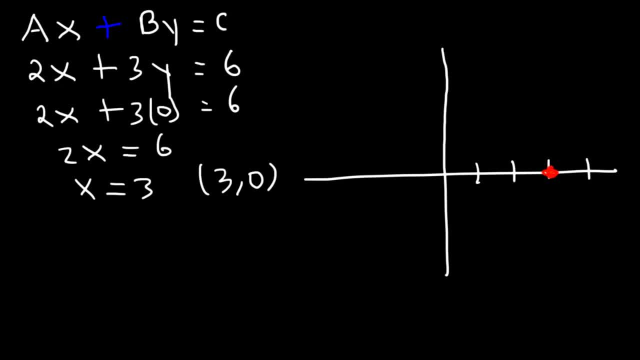 So we could plot this point here. Now let's find the y-intercept. 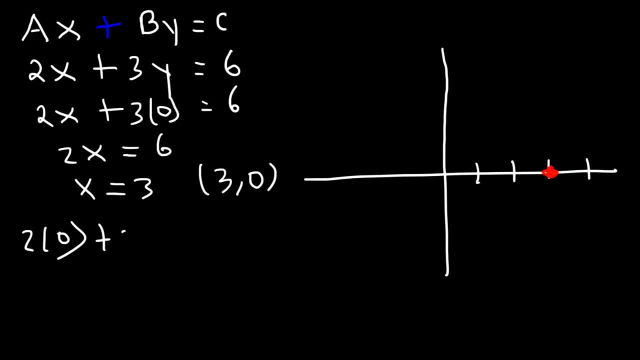 So let's replace x with 0 and find the value of y. So therefore 3y is equal to 6. And 6 divided by 3 is 2. So the y-intercept is 0 comma 2. 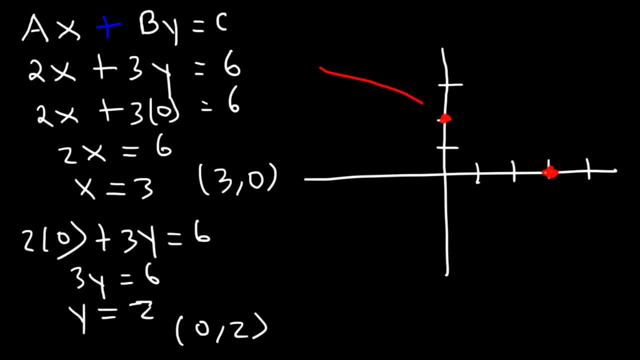 And then once you have these two intercepts, simply connect the two points with a straight line. And that's how you can graph it. 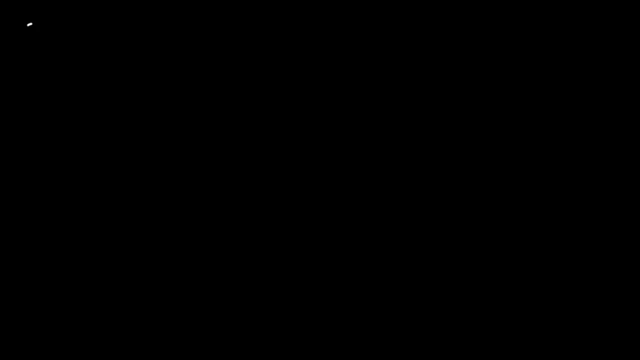 Let's try another example. Let's graph 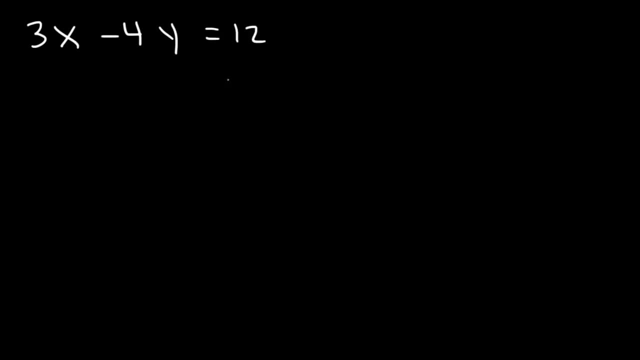 3x minus 4y is equal to 12. 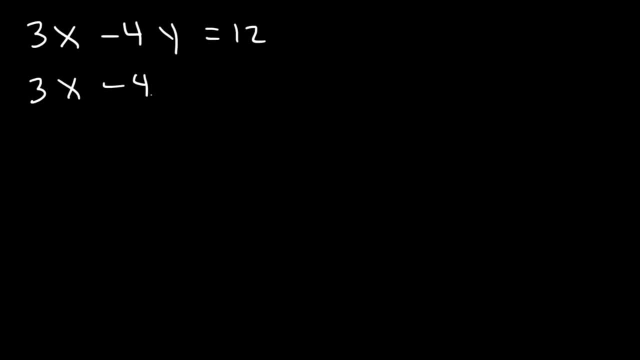 So let's find the x-intercept. So let's replace y with 0. So we can see 3x is equal to 12. 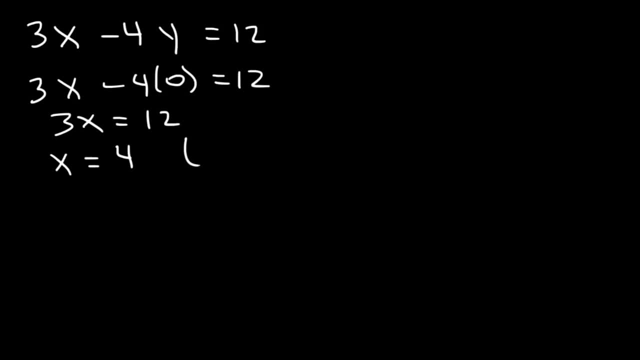 And x is 12 divided by 3, which is 4. 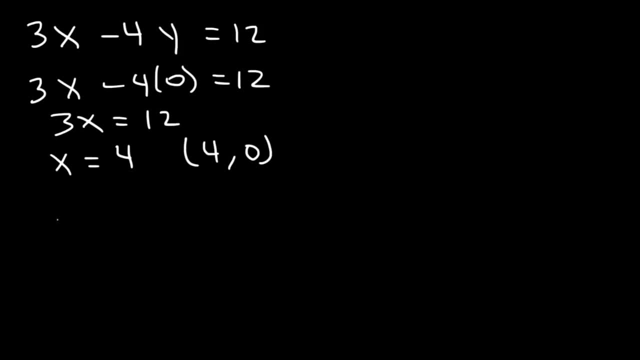 So we have the point . Now to find the 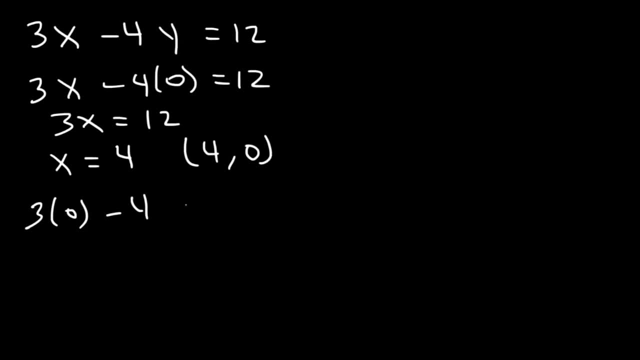 y-intercept, let's replace x with 0. So we have negative 4y is equal to 12. And 12 divided by negative 4 is negative 3. So we get the point . 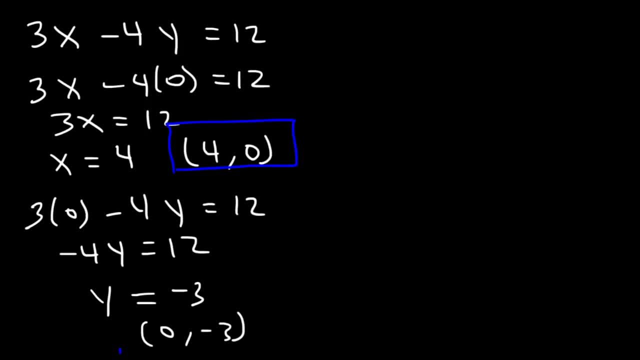 So this is the x-intercept and this is the y-intercept. 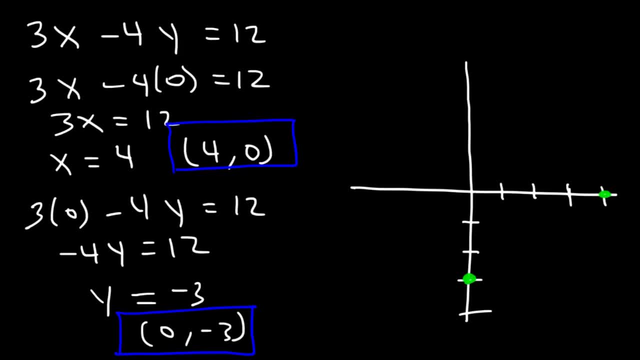 So we have the point and 4 is 0. And then just connect them. 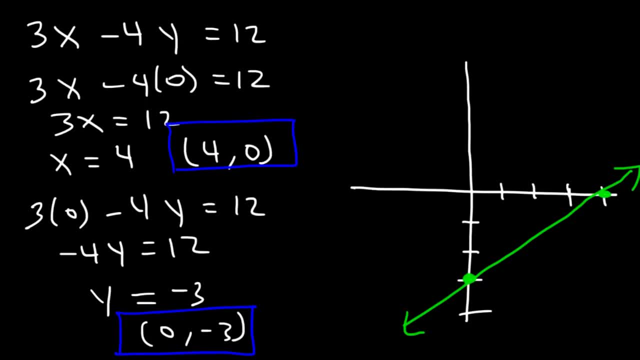 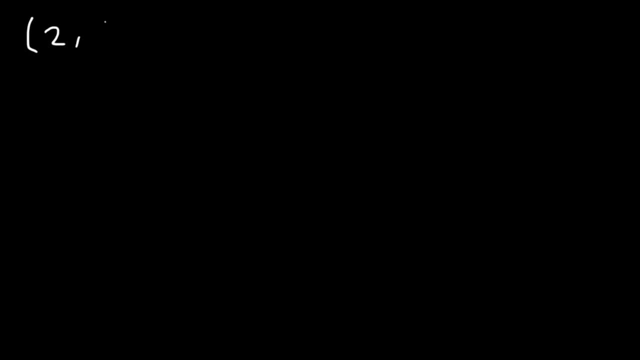 So now you know how to graph linear equations. The next thing that you need to be able to do is you need to know how to calculate the slope between two points. 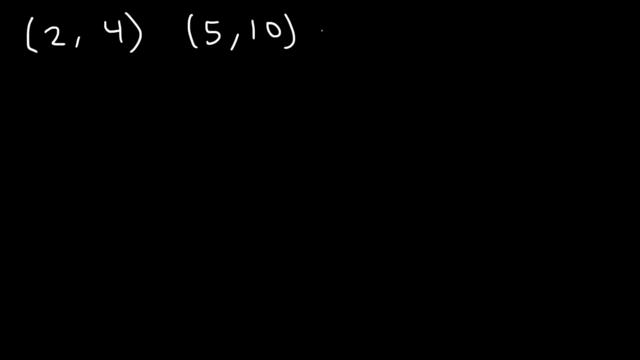 So given these two points, what is the slope of the line that connects these two points? 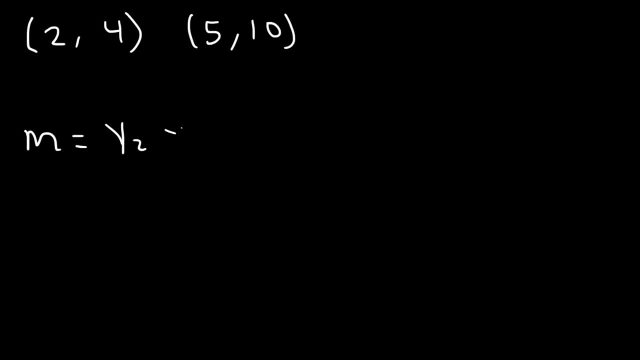 The slope is equal to y2 minus y1 divided by x2 minus x1. 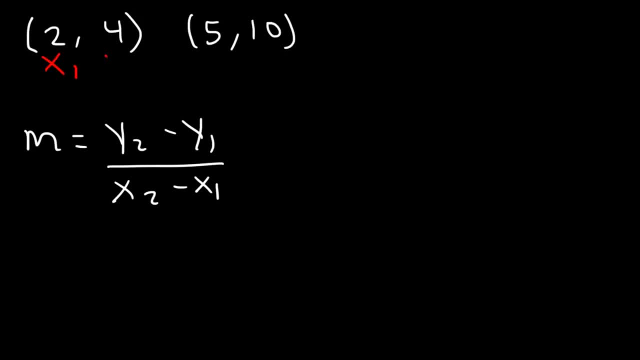 So let's call this point x1 and this one is y1. And this is x2, y2. 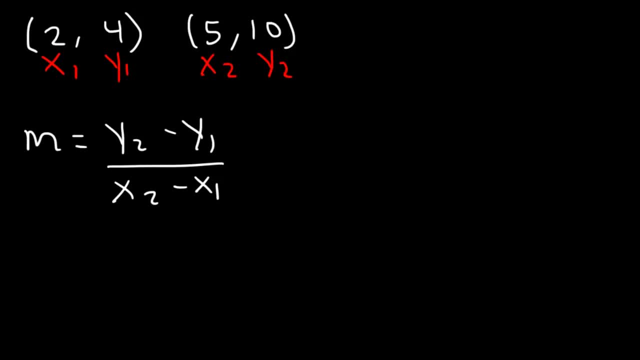 x is the first point or the first number and y is the second one. 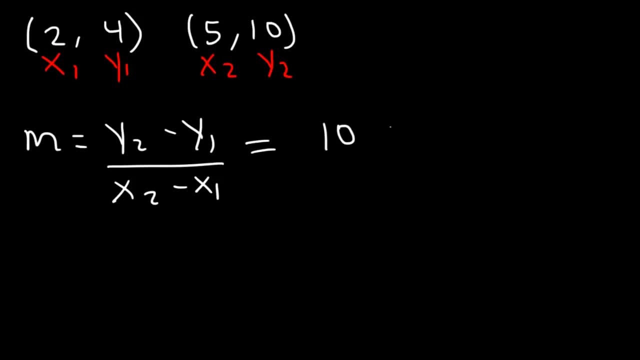 So y2 is 10. 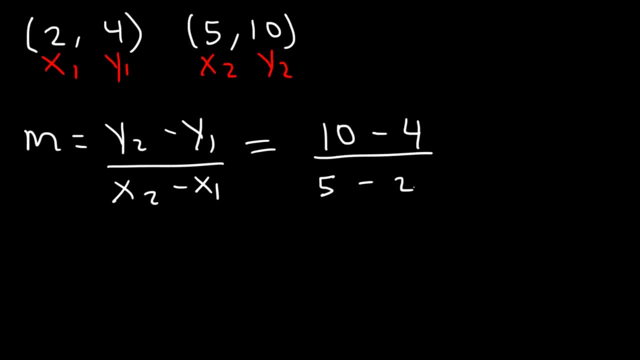 y1 is 4. x2 is 5. x1 is 2. 10 minus 4 is 6. 5 minus 2 is 3. 6 divided by 3 is 2. 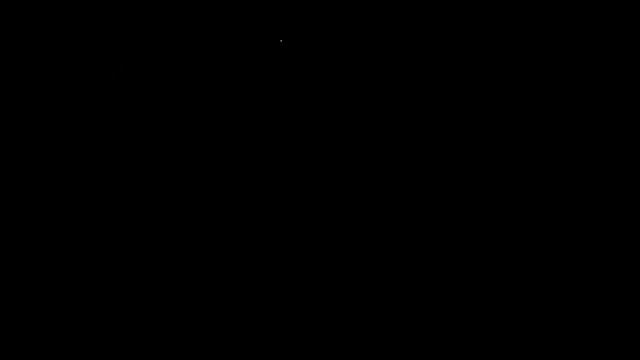 So that's how you can calculate the slope between the two points. Now try this one. 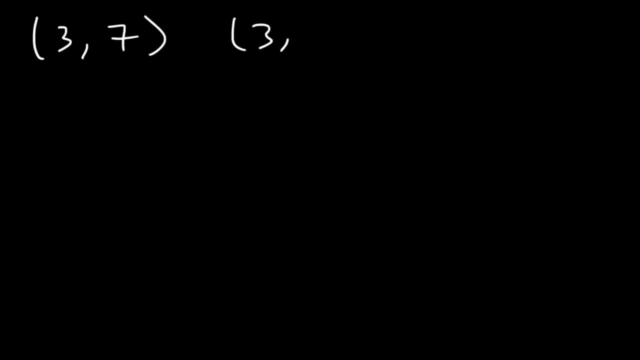 What is the slope between these two points? 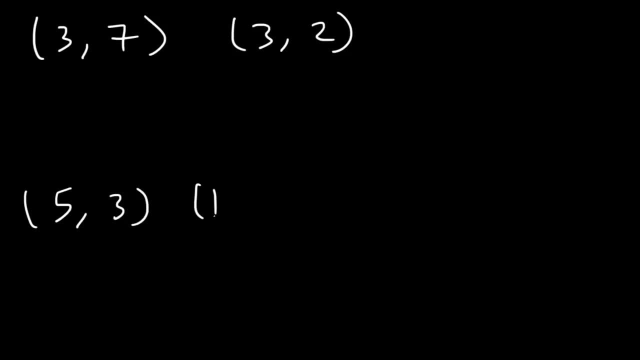 And what is the slope between these two points? 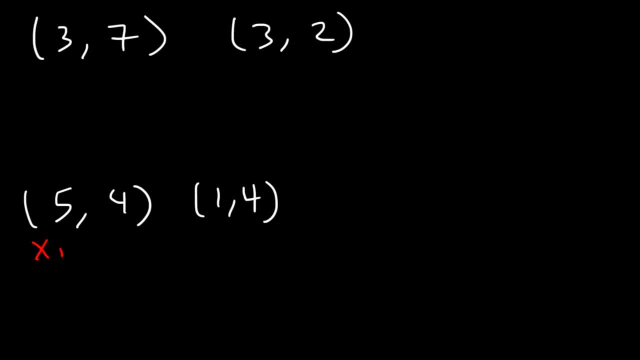 So let's start with the example below. This is x1, y1, x2, and y2. 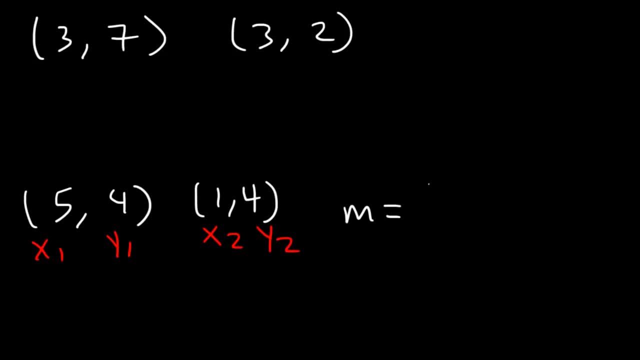 So the slope m is going to be y2 minus y1. That's 4 minus 4. Divided by x2 minus x1. That's going to be 1 minus 5. 4 minus 4 is 0. 1 minus 5 is negative 4. And 0 divided by negative 4 is 0. 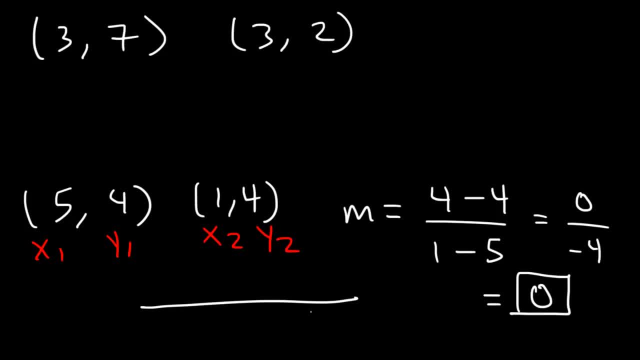 Whenever you have a slope of 0, basically you have a horizontal line. 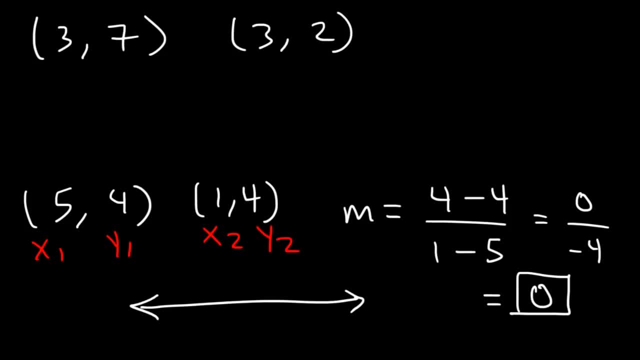 Now for the example above, this is x1, y1, x2, and y2. So the slope is going to be y2 minus y1, 2 minus 7, divided by x2 minus x1, 3 minus 3. 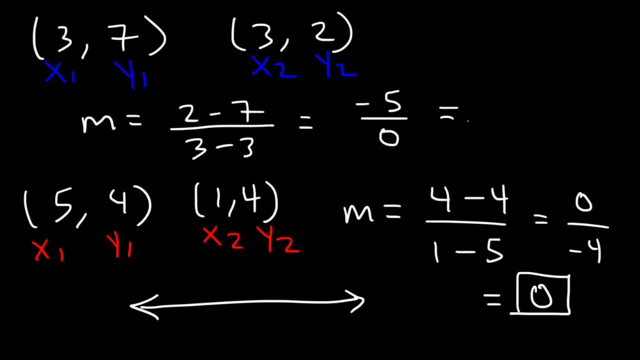 So it's negative 5 over 0. Whenever you have a 0 in the denominator, it's undefined. 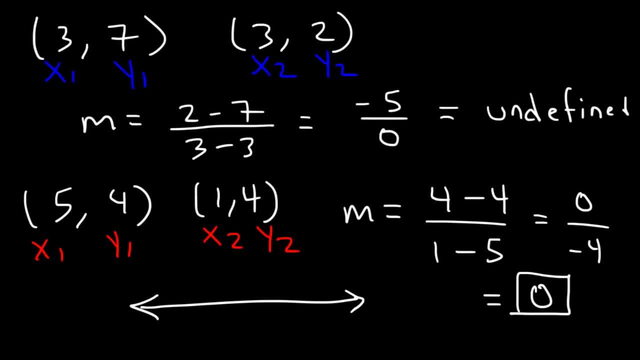 So you can't put a value to the slope. But what it means is that you have a vertical line as opposed to a horizontal line. 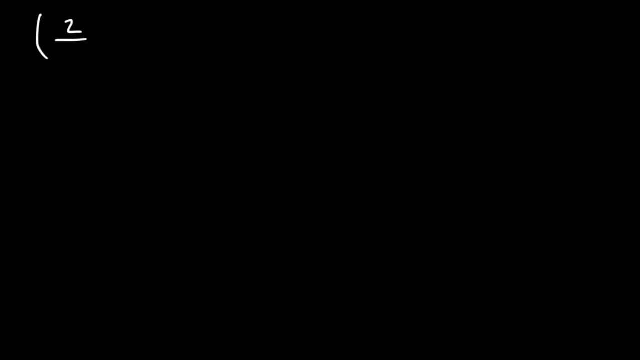 Let's try another example. One involving fractions. 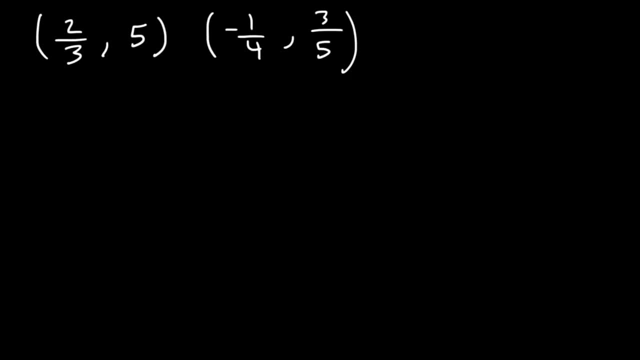 Calculate the slope of the line that connects those two points. 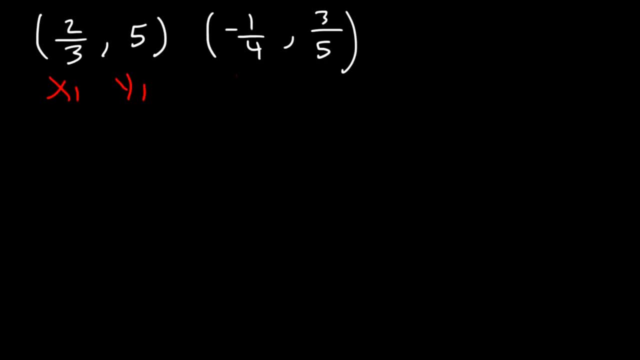 So let's identify everything. 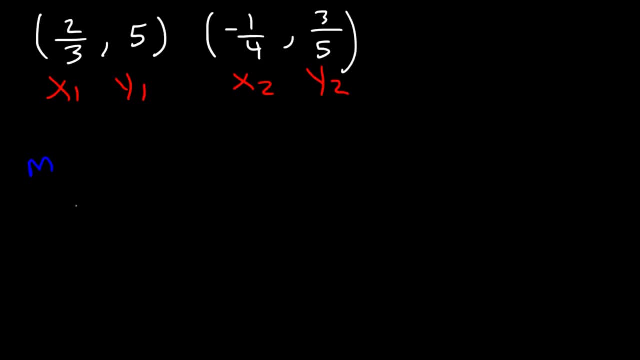 So we know the slope m is going to be y2 minus y1 divided by x2 minus x1. 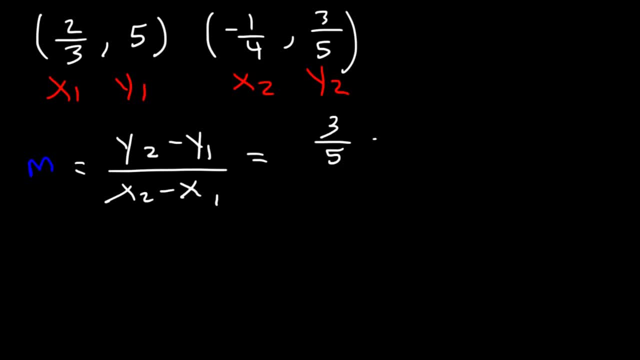 So in this example, we can see that y2 is 3 over 5, y1 is 5, x2 is negative 1 fourth, and x1 is 2 thirds. So how can we use this information to calculate the slope? How can we simplify the expression that we have? So what we have is a complex fraction. 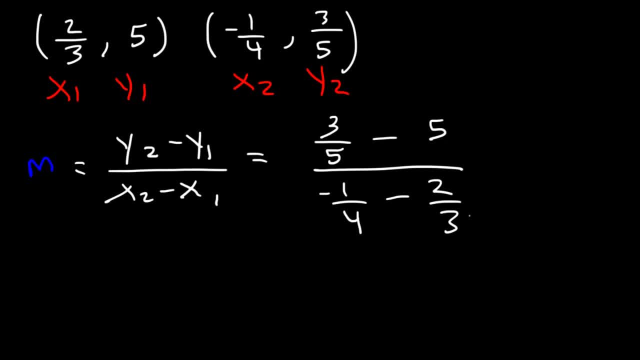 We have fractions within fractions. In a situation like this, you want to clear away the small fractions. And the only way to do that, is to multiply by the common denominator. So what is a multiple of 3, 4, and 5? If you're not sure, you can just multiply the three numbers. 3 times 4 is 12. 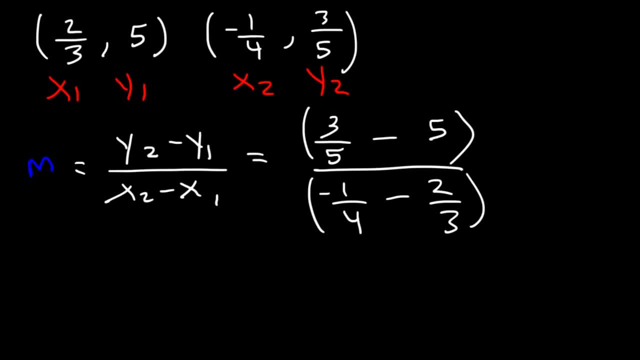 12 times 5 is 60. So we're going to multiply the top part of the fraction and the bottom by 60. That's going to clear away off many fractions. 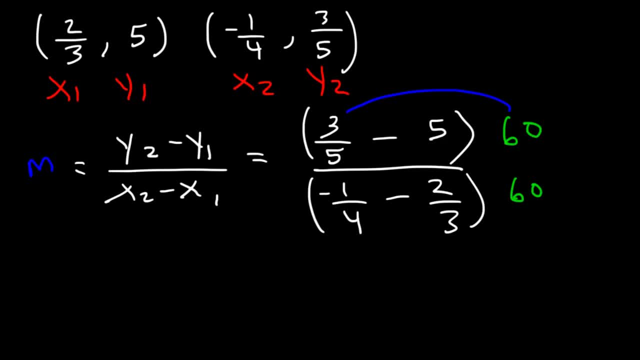 So 60 times 3 fifths, how much is that? Well we know 60 divided by 5 is 12. 12 times 3 is 36. 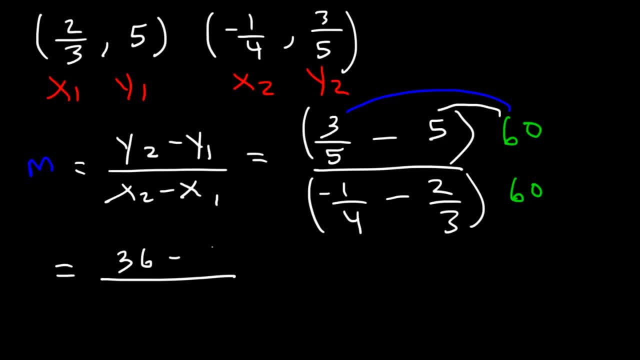 Next we have 60 times negative 5. If 6 times 5 is 30, 60 times 5 is 300. You've got to add the 0. 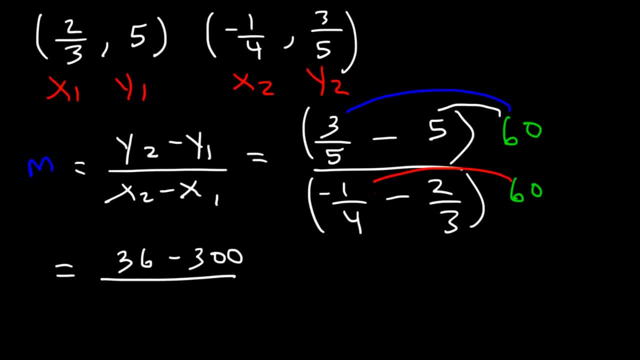 And then what's 1 fourth of 60? 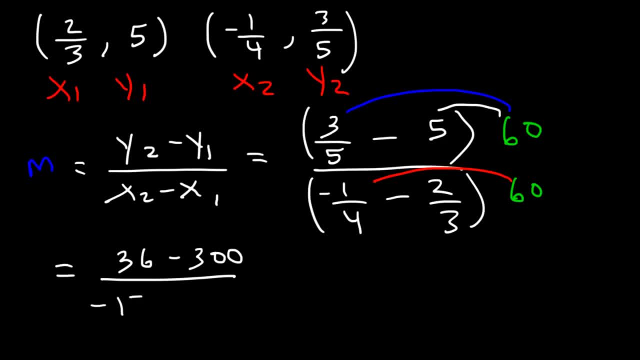 60 divided by 4 is 15. But there's a negative in front, so it's going to be negative 15. 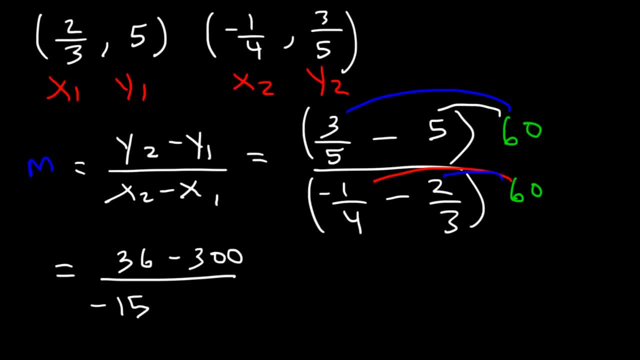 And then what is 2 thirds of 60? 60 divided by 3 is 20. 20 times 2 is 40. 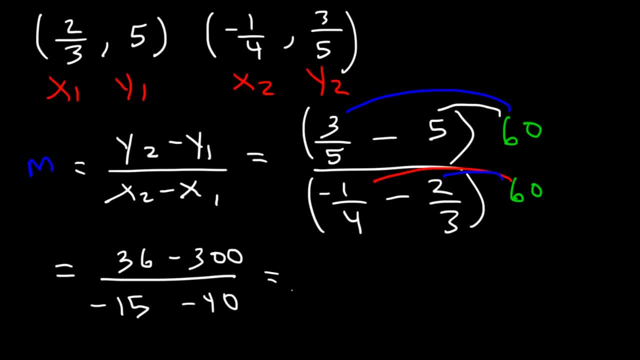 Now 30, I mean 36 rather, minus 300 is negative 264. 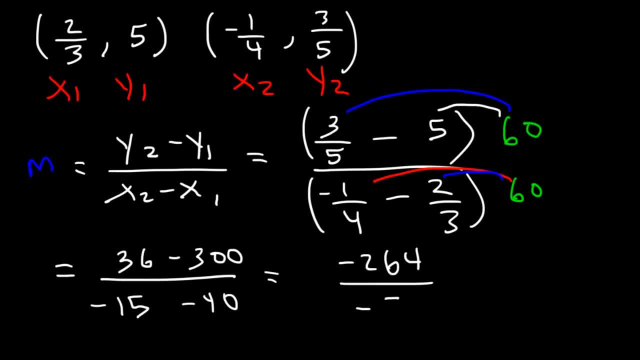 Negative 15 minus 40 is negative 55. 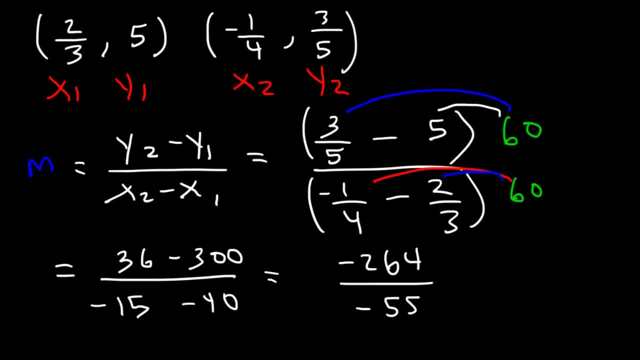 Now how can we reduce these two numbers? 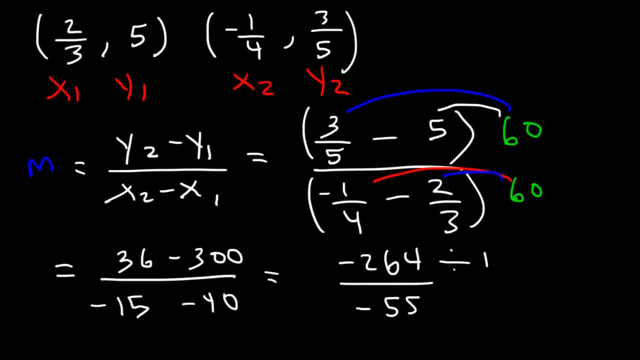 It turns out that both of these numbers are divisible by 11. And the fact that they're both negative, the negative signs will cancel. 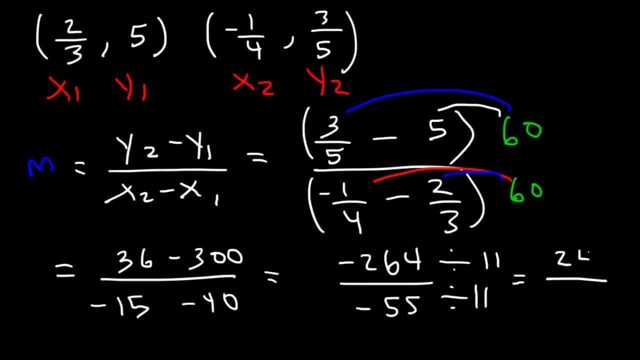 264 divided by 11 is 24. 55 divided by 11 is 5. 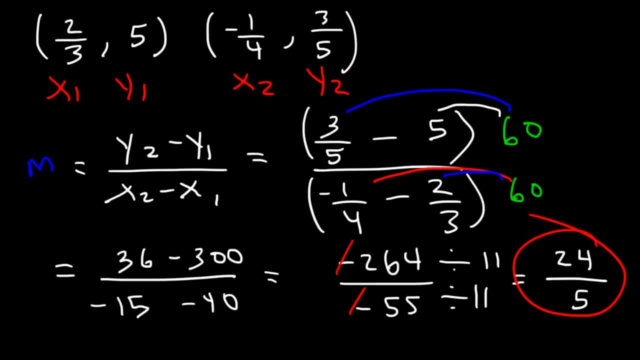 So the final answer is 24 over 5. 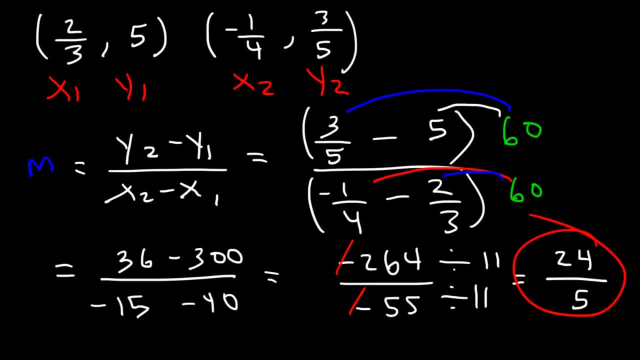 So that's the slope of the line that connects those two points. 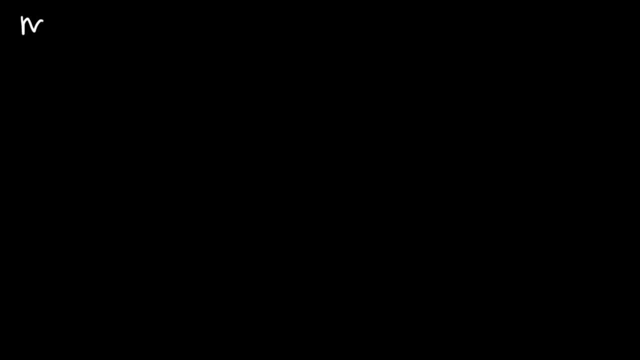 Now let's say if you're given the slope 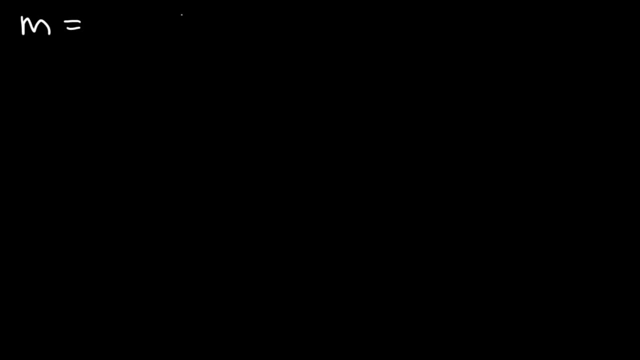 of a line that passes through the point . 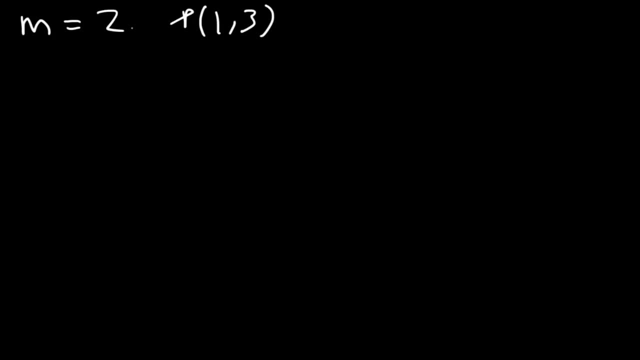 Now let's say the slope is 2. Given the slope and the point, what is the equation of the line? 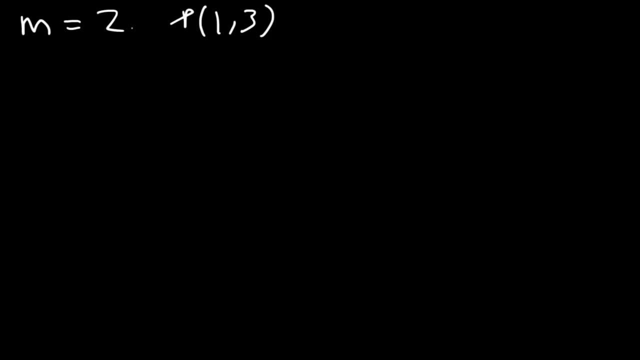 How can you write it? If you're given 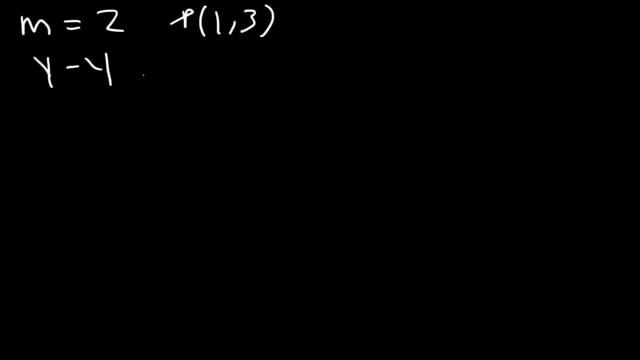 the point and the slope, you want to use the point-slope formula. y minus y1 is equal to m times x minus x1. 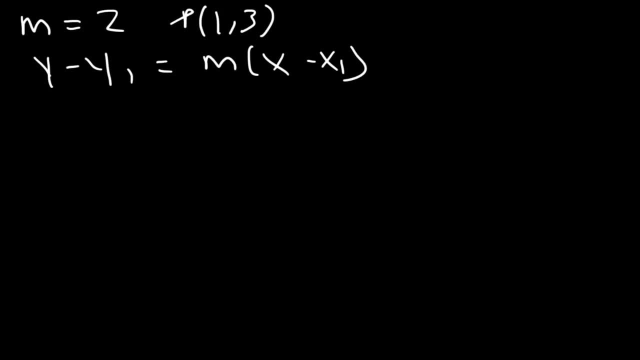 So what is x1 and y1? 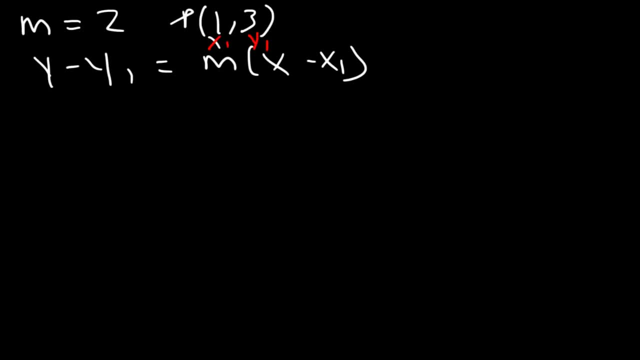 x1 is 1, y1 is 3. 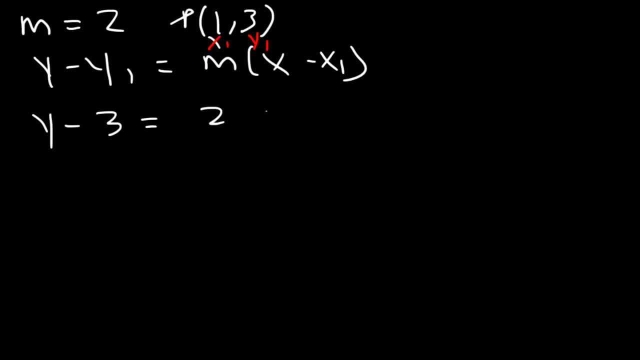 So let's replace y1 with 3, m with 2, and x1 with 1. So that's the linear equation in point-slope form. 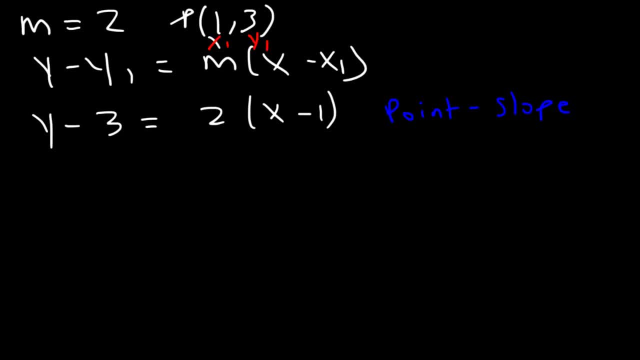 The next thing we're going to do is convert it to slope-intercept form. 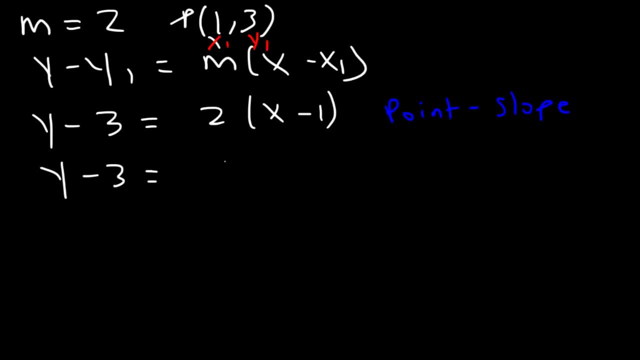 To do that, let's distribute 2 to x minus 1. So it's going to be 2x minus 2. 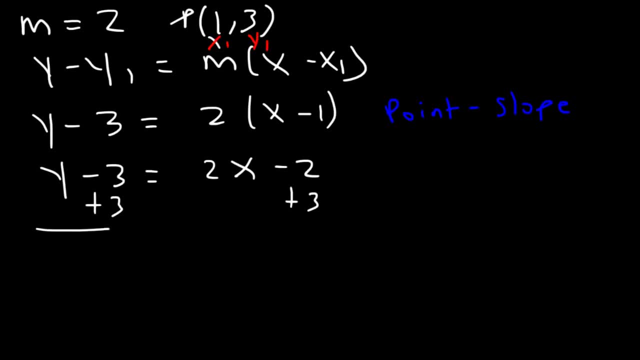 And then let's add 3 to both sides. So we've got to get y by itself. 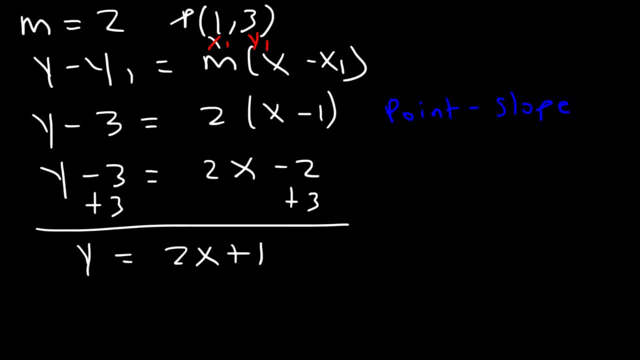 So it's 2x plus 1. So in this equation, 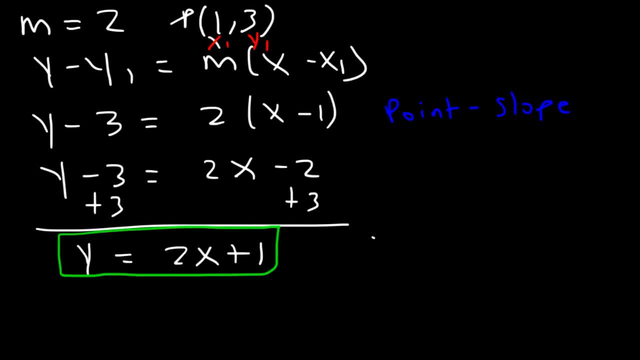 it's now in slope-intercept form. 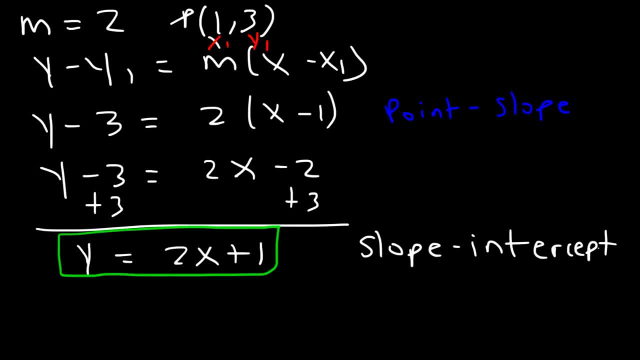 As you can see, it's in the form y is equal to mx plus b. 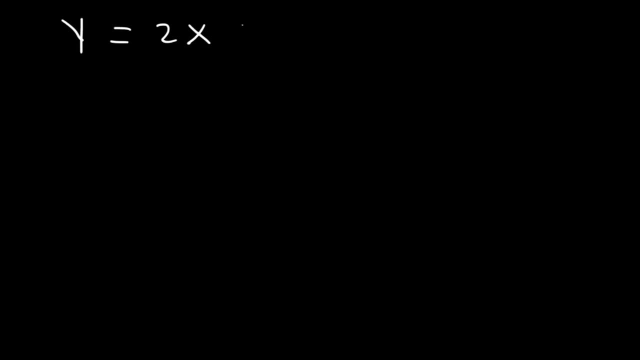 So now once we have it in slope-intercept form, if we want to, we can convert it to standard form. In this case, all we need to do is take the 2x and move it to this side. So it's negative 2x plus 1y is equal to 1. Now let's multiply everything by negative 1. 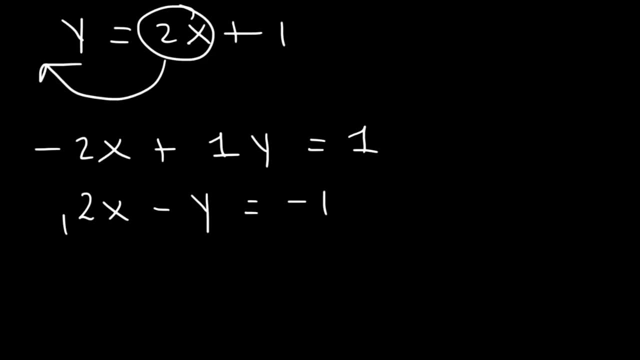 So it's 2x minus y is equal to negative 1. So now it's in standard form. 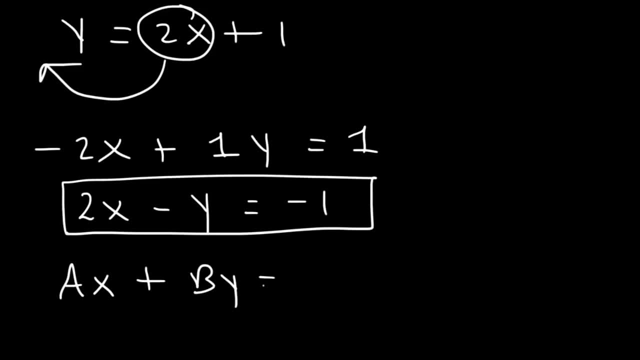 That is ax plus by is equal to c. 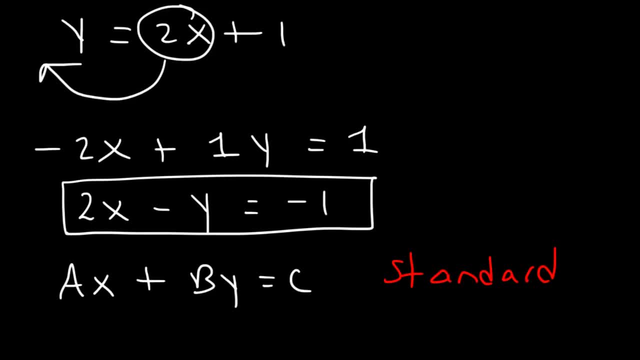 So now you know how to write a linear equation given a slope, the slope, and a point. 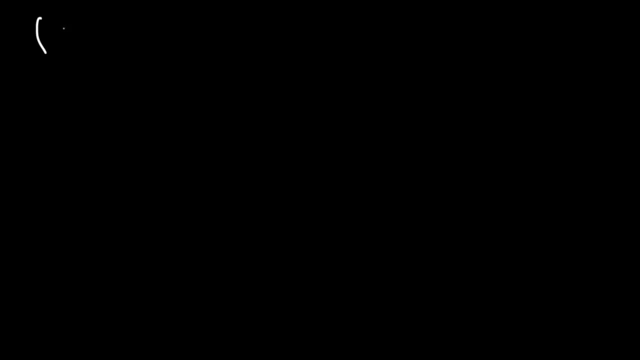 Now what if you're given two points instead? For example, let's say if you're given the point and the point . Go ahead and write the linear equation in point-slope form, slope-intercept form, and standard form. 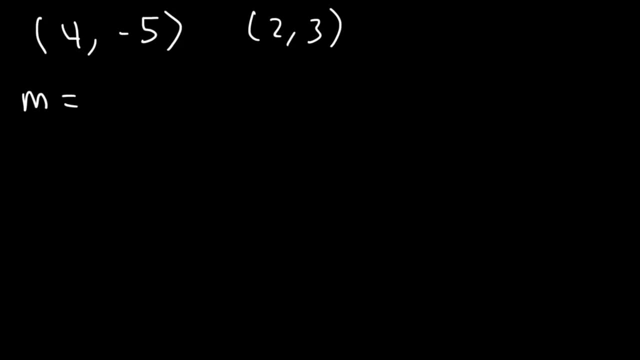 In this case, the first thing you need to do is calculate the slope. So this is x1, y1, x2, y2. So the slope is going to be y2 minus y1, which is 3 minus negative 5, divided by x2 minus x1, which is 2 minus 4. 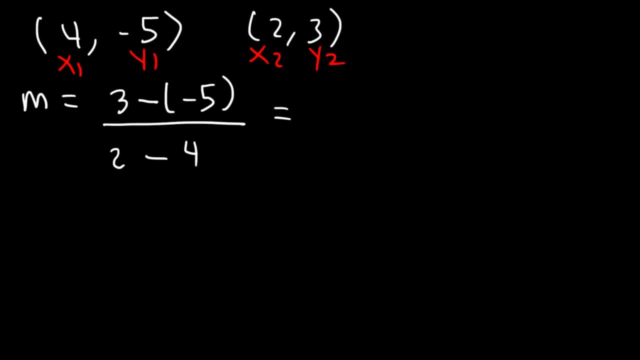 3 minus negative 5 is the same as 3 plus 5. That's 8. 2 minus 4 is negative 2. 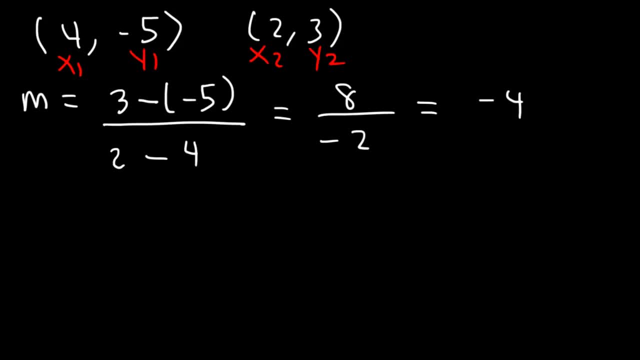 And 8 divided by negative 2 is negative 4. So that's the slope. 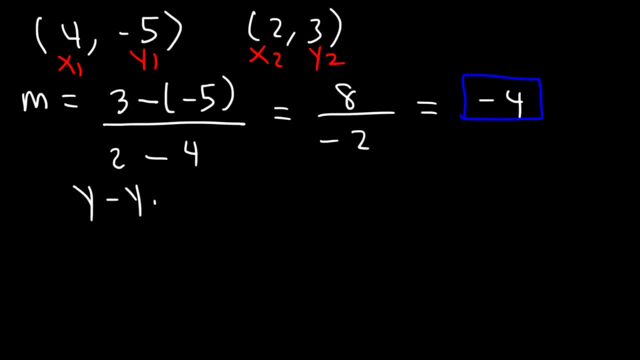 Now let's use the point-slope formula to put it to write the linear equation. 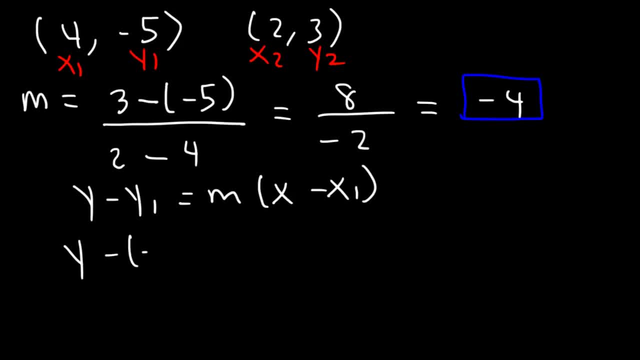 So why is y1 is negative 5, m is negative 4, and x1 is 4? 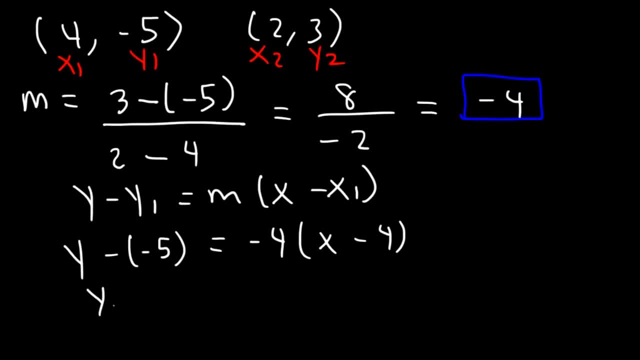 So y minus negative 5 is the same as y plus 5. 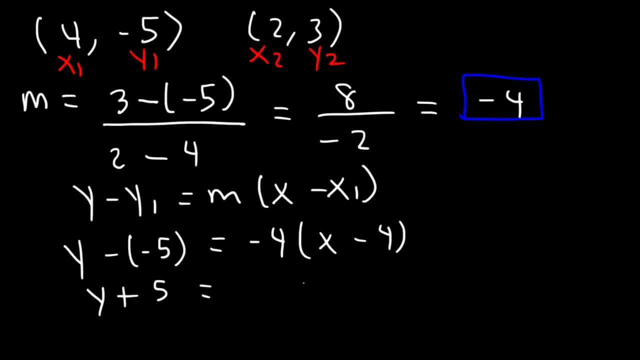 Let's distribute negative 4 to x minus 4. 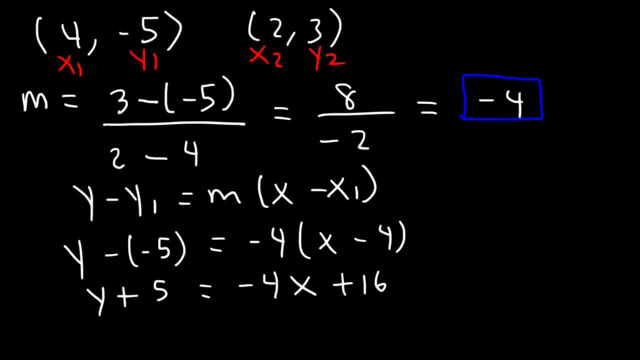 So it's negative 4x plus 16. And then let's subtract both sides by 5. So y is equal to negative 4x plus 11. 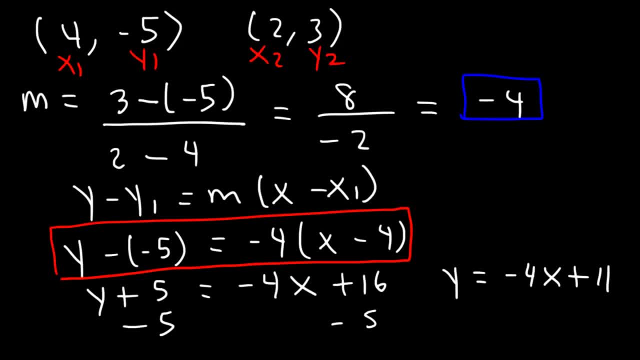 So in this form, it's in point-slope form. But here, we have it in slope-intercept form. 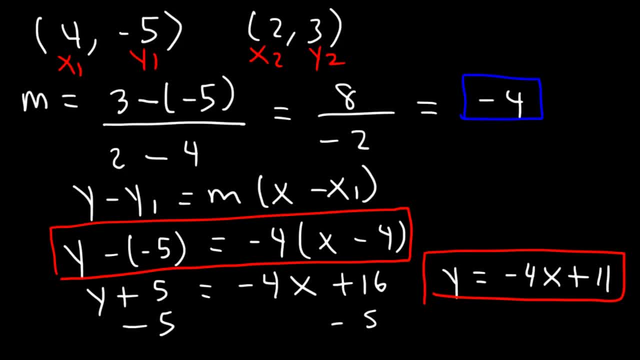 To write it in standard form, let's take the negative 4x and move it to this side. So it's going to be 4x plus y is equal to 11. So that's the answer in standard form. 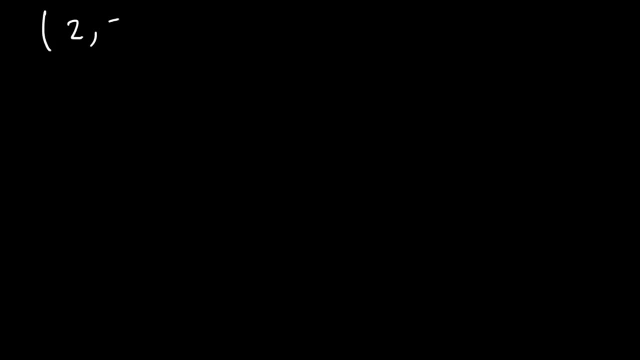 Now let's say if we have the point and the point . 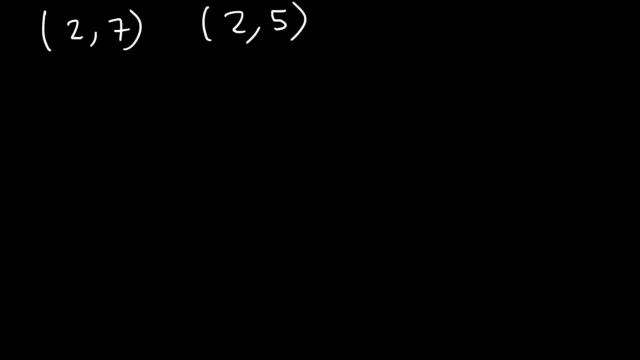 What is the equation of the line that passes these two points? 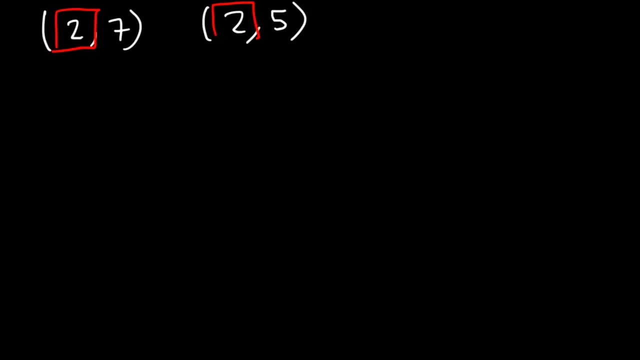 Now notice that x doesn't change. Whenever you see that, that means the slope is undefined. And it's very easy to write the equation because it's going to be a vertical line. 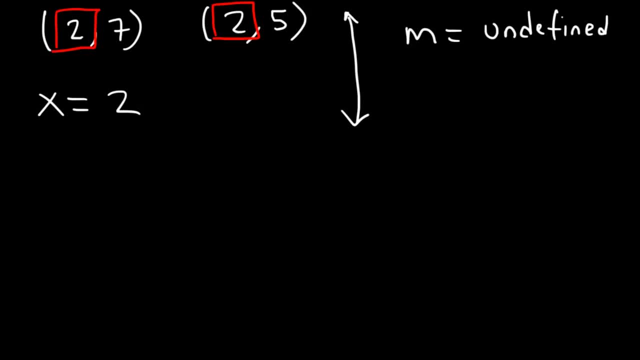 And all it is is x is equal to 2 because the x value doesn't change. So that's how you can write the linear equation whenever the x variable is the same. 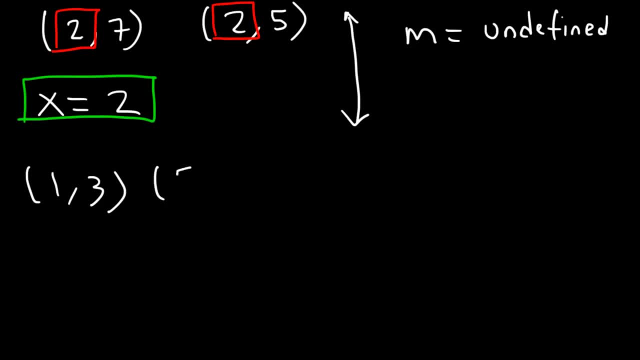 Now if you have an example where the y variable is the same, 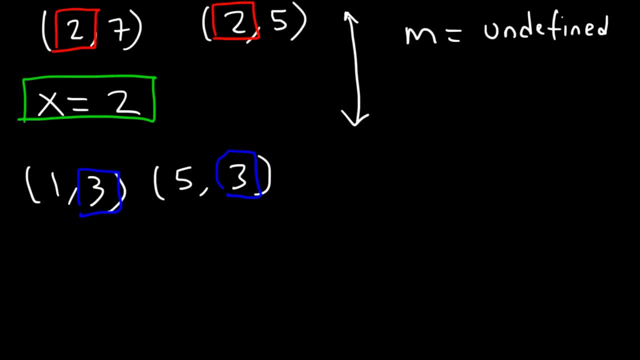 the slope is going to be equal to 0. 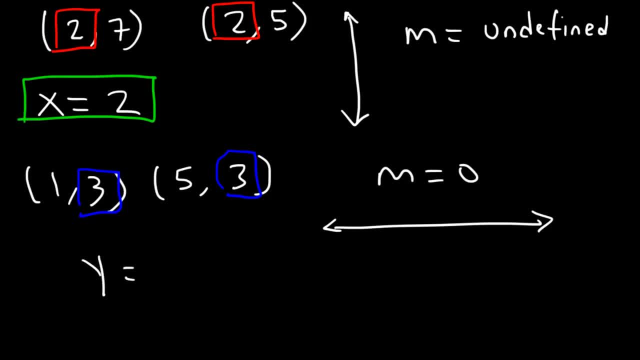 And so you're going to have a horizontal line. And the equation is simply y is equal to 3 because the y value doesn't change. 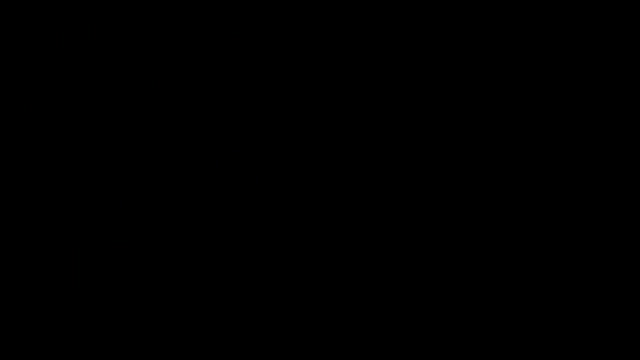 So watch out for those two examples. Now the next thing we need to talk about is parallel lines. 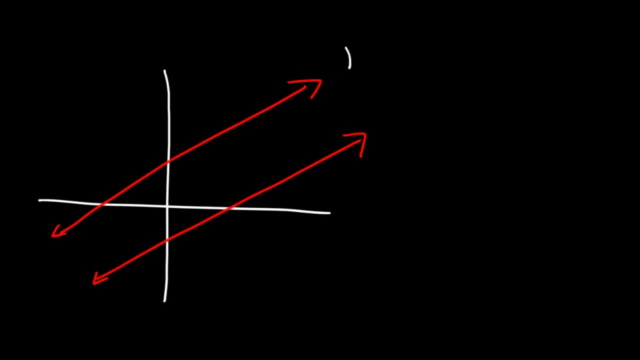 Let's say if the slope of the first line is 2, what is the slope of the second line? So when dealing with parallel lines, you need to realize that they share the same slope. So if the slope of the first line is 2, the slope of the second line is 2. 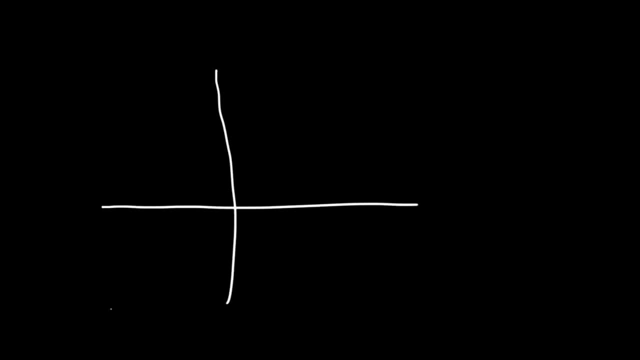 Now what about perpendicular lines? For example, let's say this is line 1. Line 2 is going to be 90 degrees apart from line 1. 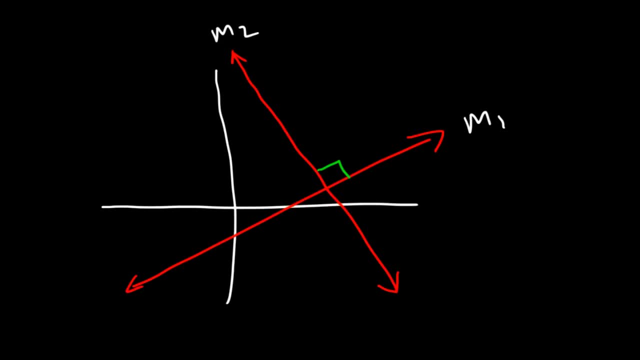 The angle between them is 90, and that makes them perpendicular. 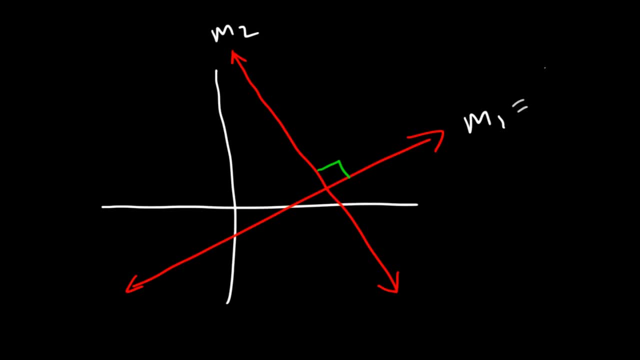 So let's say if the slope of line 1 is 4 over 5. What is the slope of line 2? 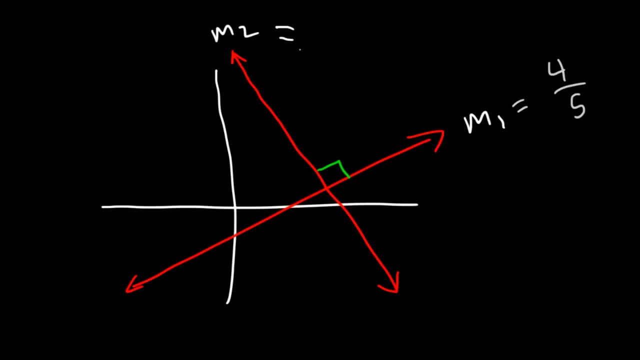 Line 2 is going to be the negative reciprocal of 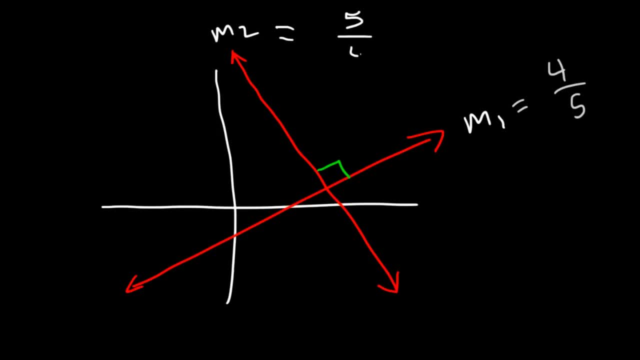 line 1. So you've got to flip the fraction. So instead of being 4 over 5, it's now 5 over 4. 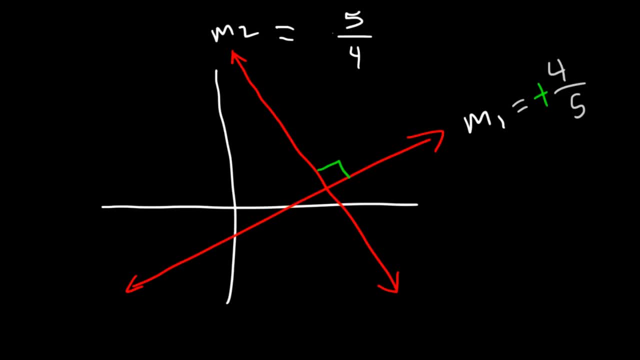 And you've got to change this line from positive to negative. 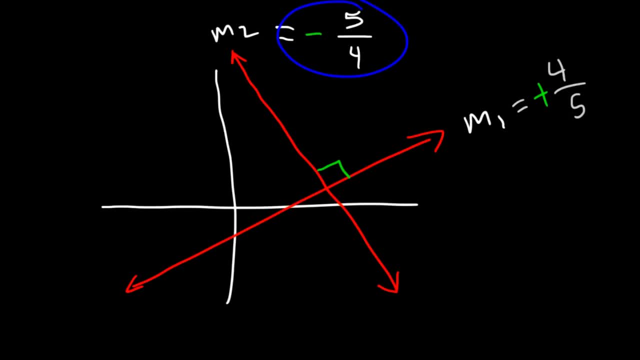 So the slope of the second line is negative 5 over 4. So that's the situation between perpendicular lines. 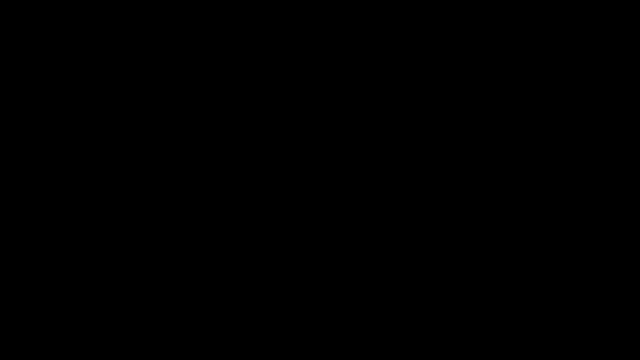 Now let's move on to quadratic equations. 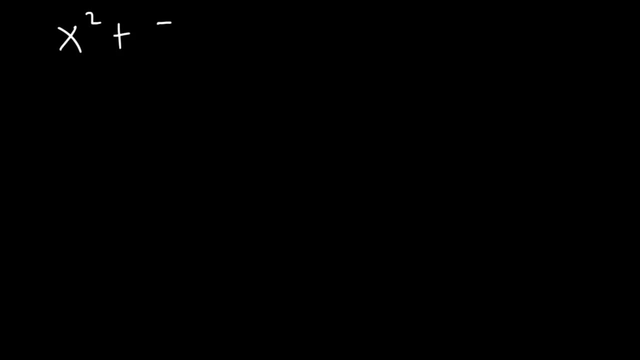 Let's say if we have the equation x squared plus 5x plus 6 is equal to 0. How can we find the value of x in this quadratic equation? 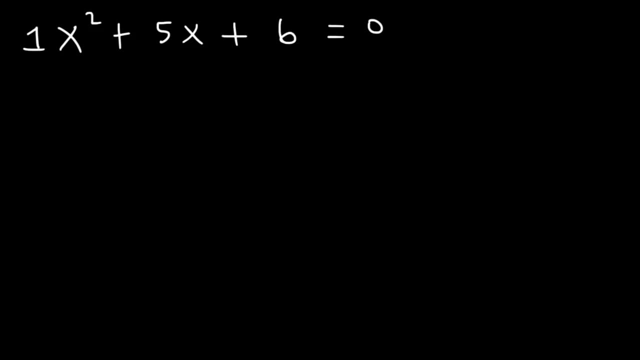 In this example, we have a trinomial where the leading coefficient is 1. What you've got to do is find two numbers that multiply to 6, but add to the middle coefficient 5. 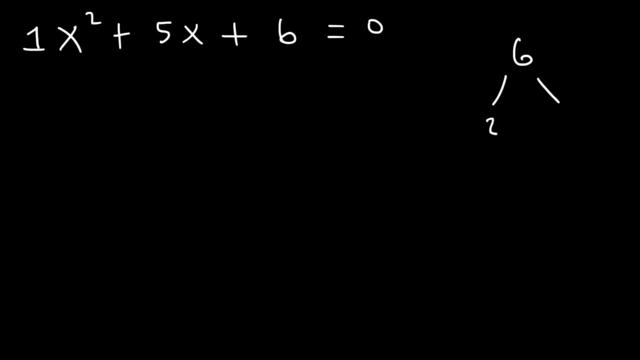 What are those two numbers? In this case, it's going to be 2 and 3. 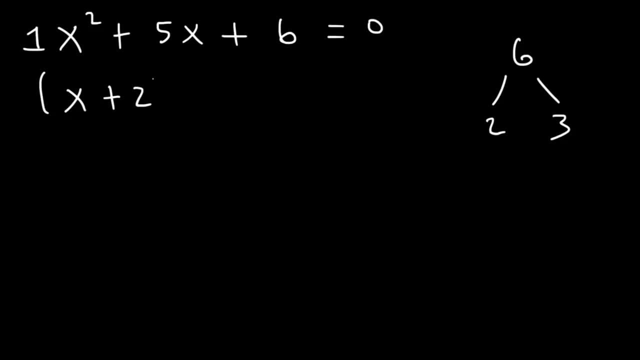 So to factor it, it's going to be x plus 2 times x plus 3. 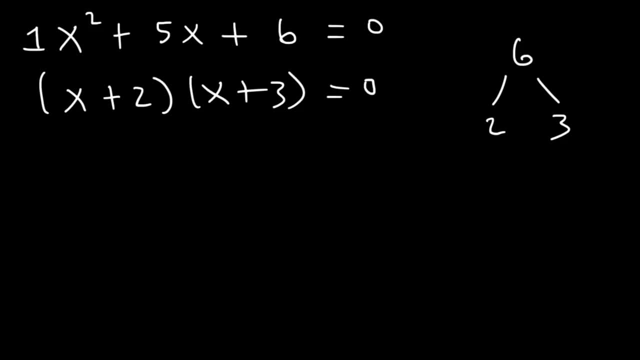 And in order to solve it using the zero product property, set each factor equal to 0. 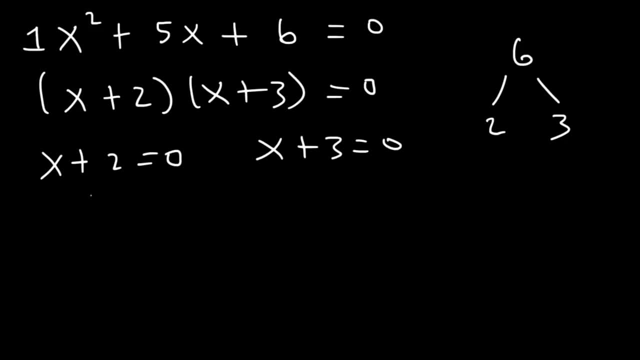 Now, if x plus 2 is equal to 0, we need to subtract both sides by 2. So we can see x is equal to negative 2. That's the first answer. 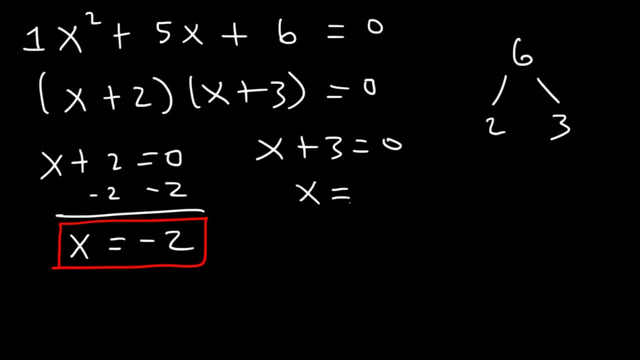 For the other one, if we subtract both sides by 3, we can see that x is equal to negative 3. 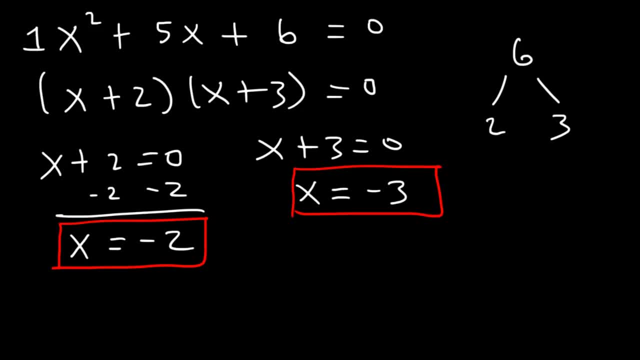 So those are the two answers in this particular equation. 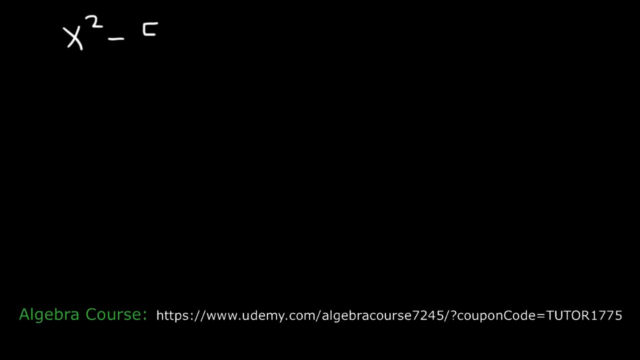 Here's another example. Let's say that x squared minus 5x minus 24 is equal to 0. Go ahead and find the value of x. So find two numbers that multiply to negative 24, but add to negative 5. So let's start with 1. 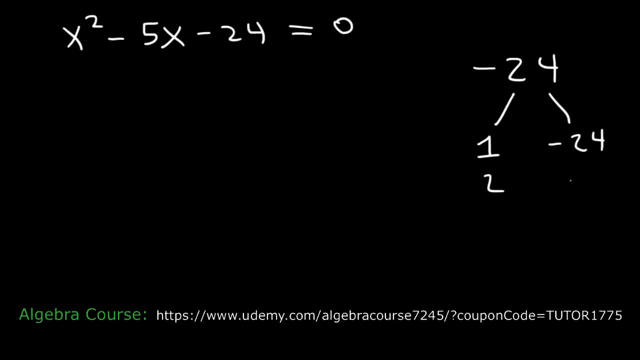 Negative 24 divided by 1 is negative 24. If we divide it by 2, it's negative 12. 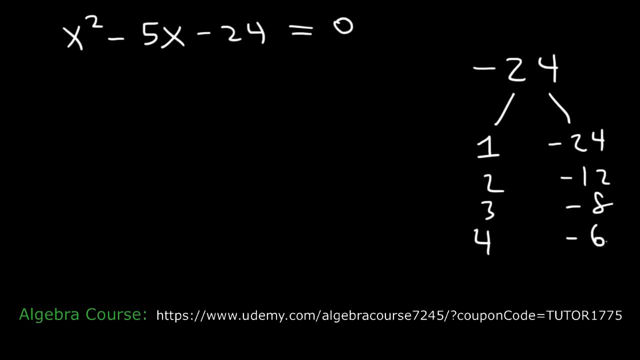 If we divide it by 3, it's negative 8. If we divide it by 4, it's negative 6. So it's good to make a list. 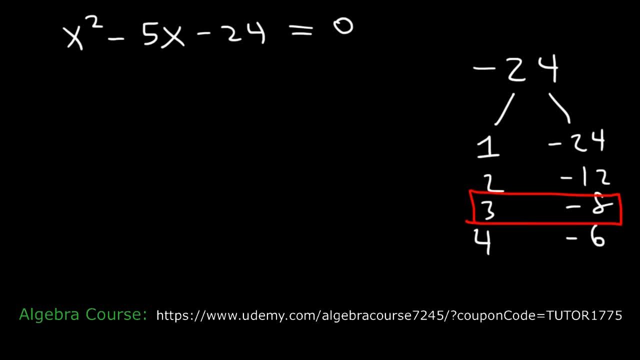 But notice that 3 and negative 8 differ by 5. That is by negative 5. 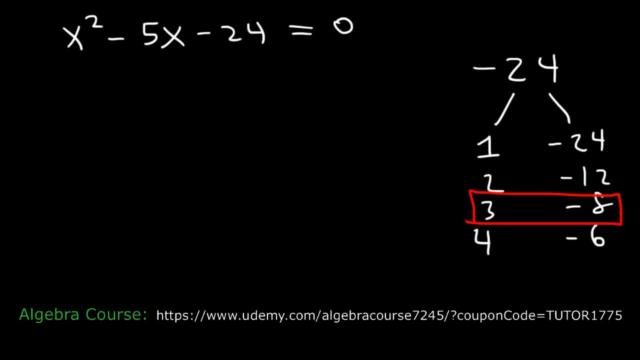 If you add them, you get negative 5. And if you multiply them, you get negative 24. 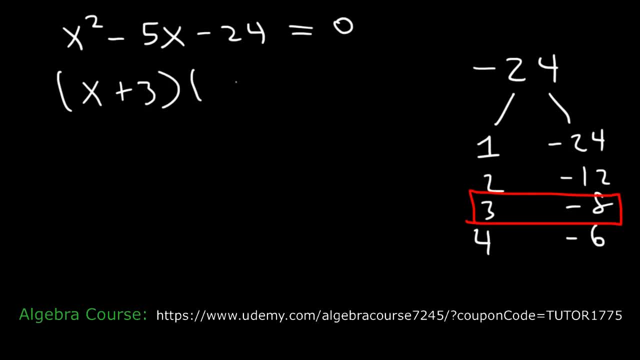 So therefore, it's going to be x plus 3 times x minus 8. 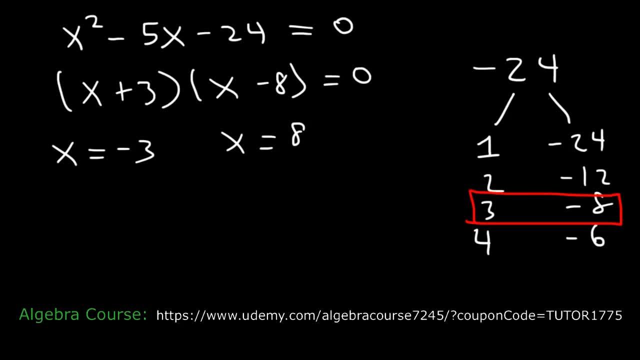 So x is equal to negative 3 and positive 8. And so that's the answer for this particular example. 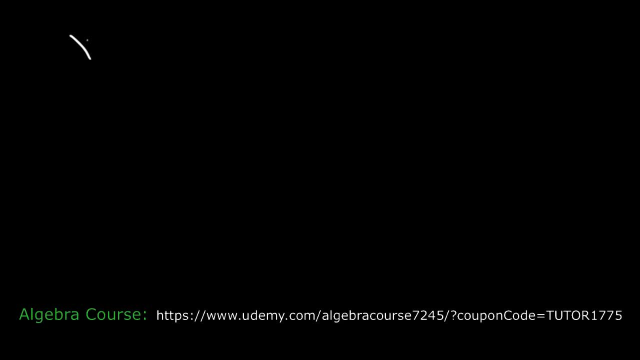 Here's another example. x squared minus 3 squared plus 4x minus 21. So what two numbers multiply to negative 21 but add to 4? So we know 7 times 3 is 21. So which one is it going to be? Negative 7 and 3 or 7 and negative 3? Positive 7 plus negative 3 adds up to 4. 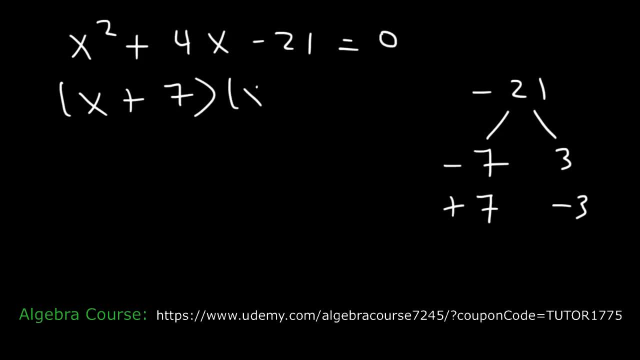 So therefore, it's going to be x plus 7 times x minus 3. So x is equal to negative 7 and positive 3. 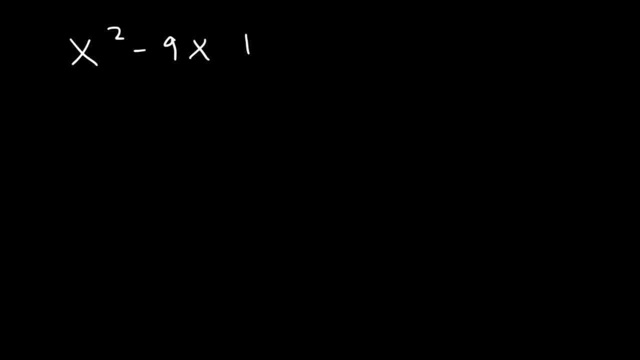 And let's try another example. x squared minus 9x plus 18. So what two numbers multiply to 18 but add to negative 9? 6 times 3 is 18 but that adds to positive 9. 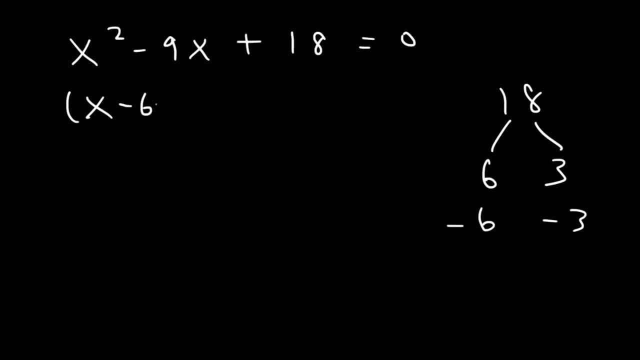 So it has to be negative 6 to negative 3. So it's x minus 6 times x minus 3. So the two answers are positive 6 and positive 3. 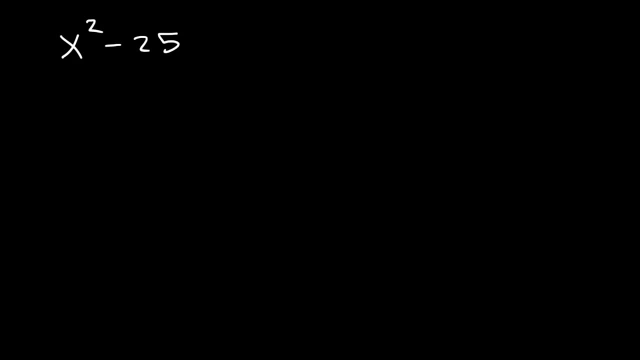 Now what about this problem? x squared minus 25 is equal to 0. 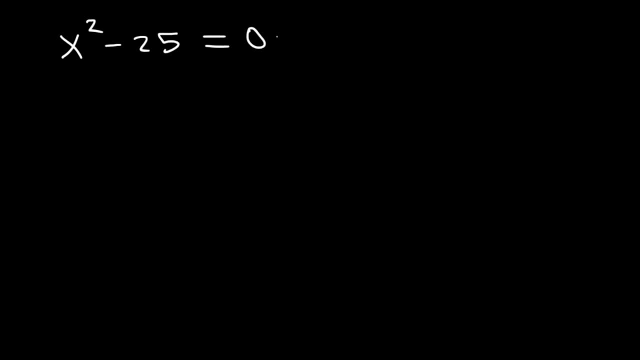 How can you factor that particular expression and at the same time find the value of x? 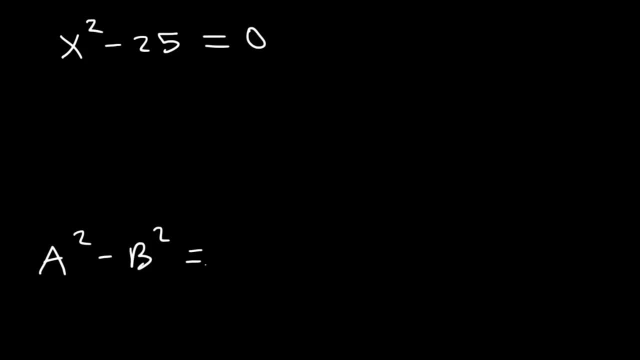 So this expression is in the form of a difference of perfect squares. To factor it, it's going to be a plus b times a minus b. So the square root of x squared is x. 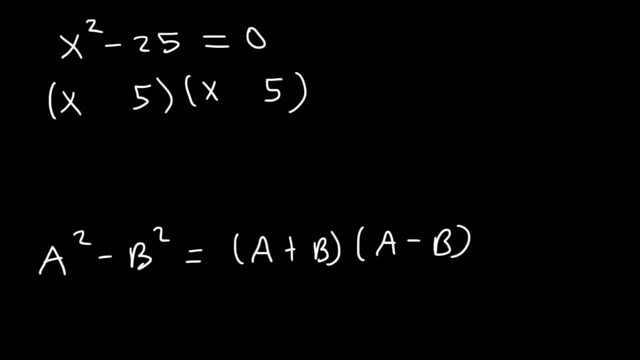 The square root of 25 is 5. So one is going to be positive and the other is going to be negative. So therefore x is equal to negative 5 and positive 5. So that's all you need to do in this particular example. 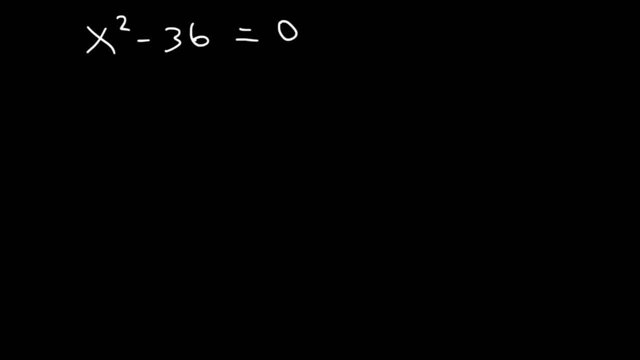 Try this one. x squared minus 36 is equal to 0. 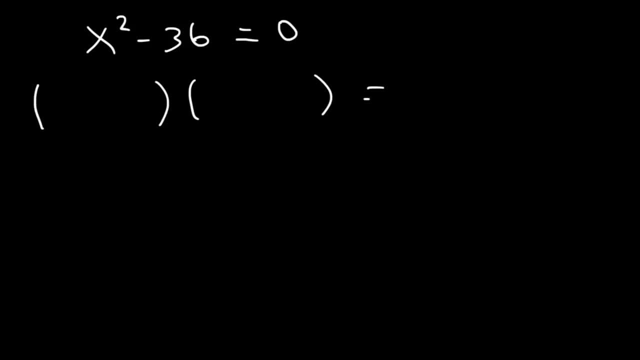 So once again we have a difference of perfect squares. 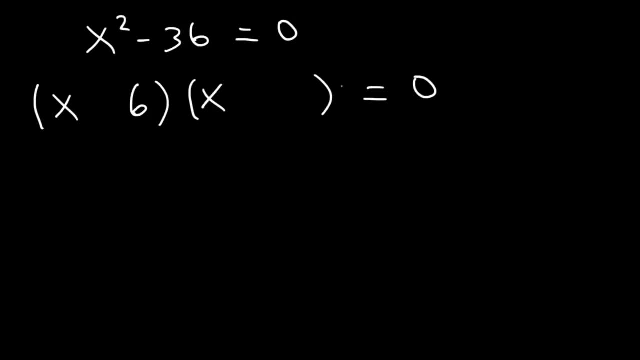 The square root of x squared is x. The square root of 36 is 6. 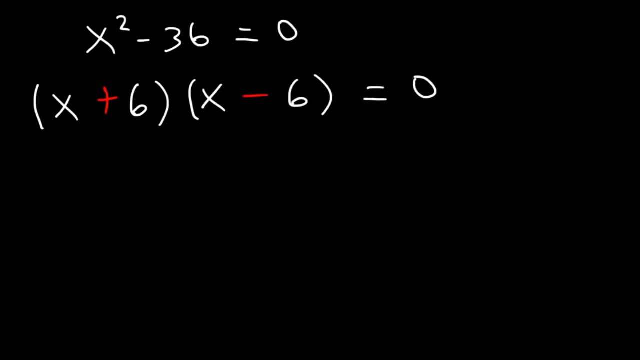 So it's going to be x plus 6 times x minus 6. So x is equal to negative 6 and positive 6. Don't forget to change the sign. 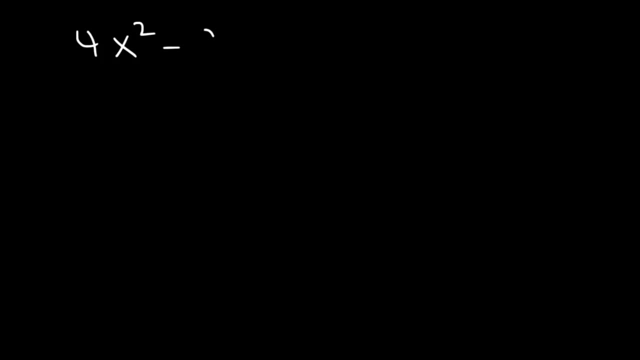 Now let's change it up a bit. What about minus 81? What is the value of x in that case? 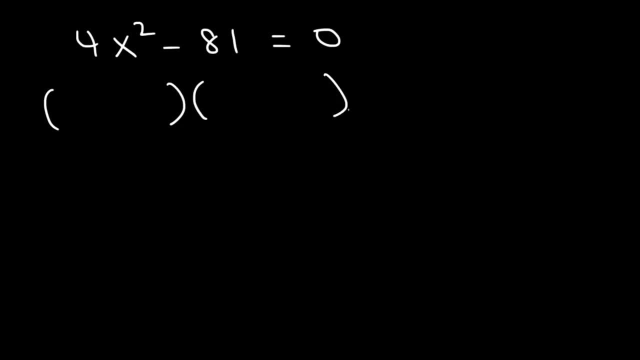 So what is the square root of 4x squared? The square root of 4 is 2. The square root of x squared is x. 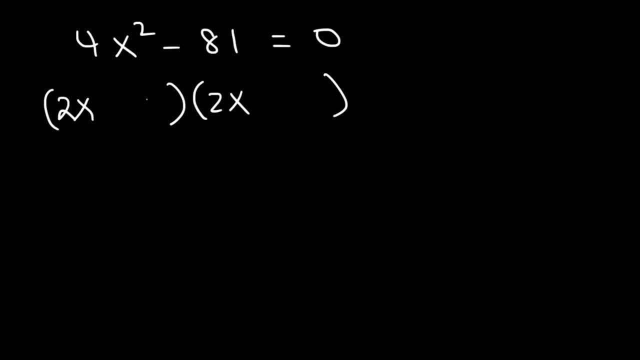 So the square root of 4x squared is 2x. The square root of 81 is 9. 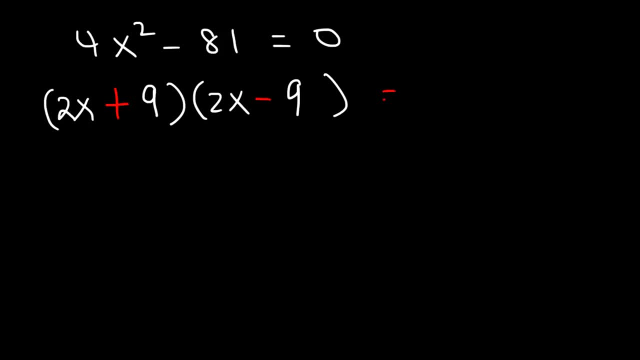 So it's going to be 2x plus 9 2x minus 9. And that's equal to 0. So if we set 2x plus 9 equal to 0, we need to subtract both sides by 9. 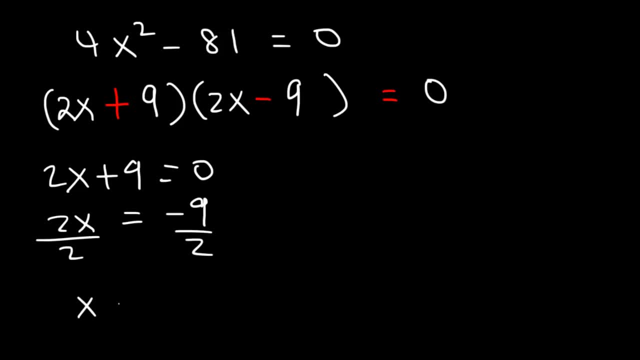 2x is negative 9 and then divide by 2. So the first answer is negative 9 over 2. Which means the other one is positive 9 over 2. So in this case, we're going to get a fractional answer. 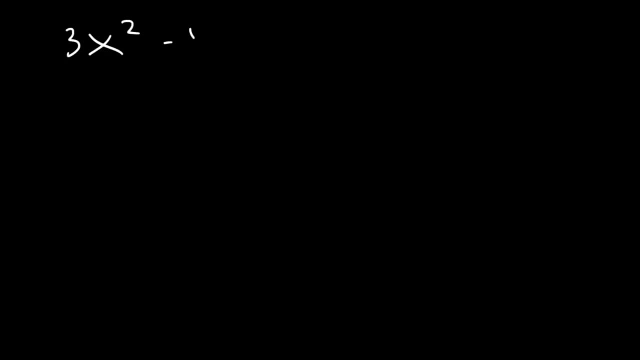 Now how about this one? 3x squared minus 48 is equal to 0. 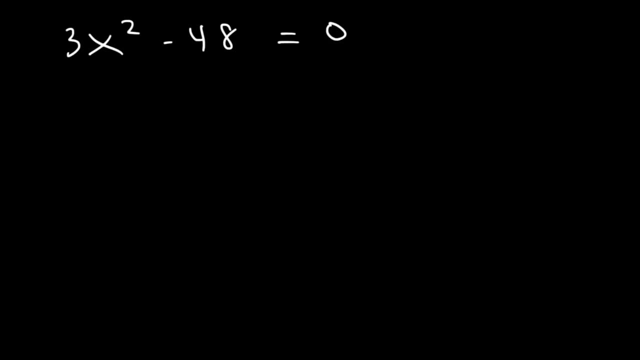 We can't really take the square root of 3. It's not going to be a nice whole number. However, what we can do is factor out the GCF, the greatest common factor, which is 3. 3x squared divided by 3 is x squared. Negative 48 divided by 3 is negative 16. 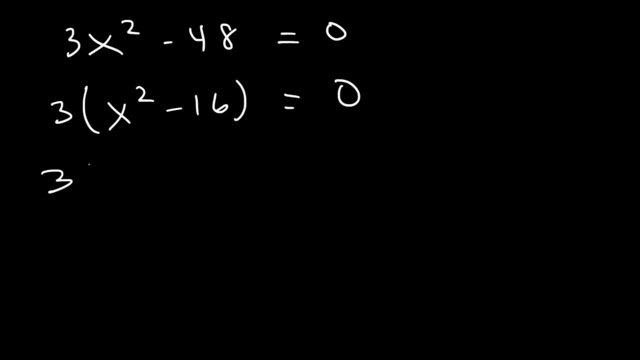 So notice that x squared minus 16 is a difference of perfect squares. 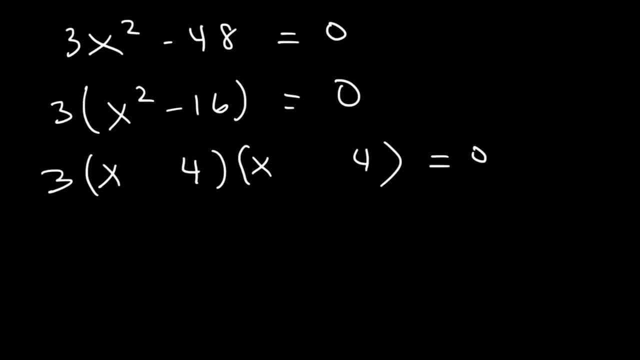 The square root of 16 is 4. So therefore, we can see that x can be equal to negative 4 and positive 4 in this particular example. 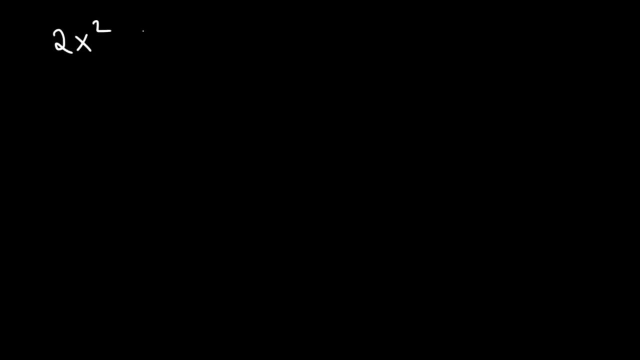 Now sometimes, you might have a quadratic equation that is a trinomial that is with three terms, 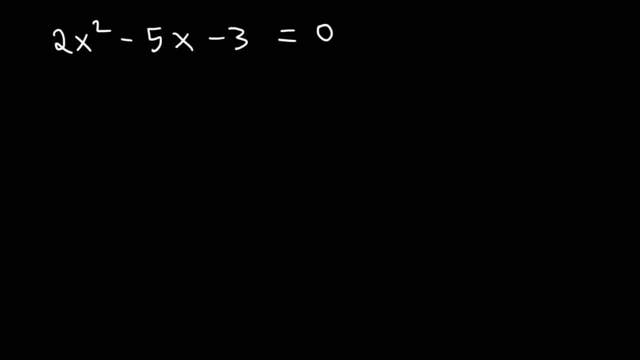 but where the leading coefficient is not 1. In a case like this, how can we factor it in order to find the value of x? 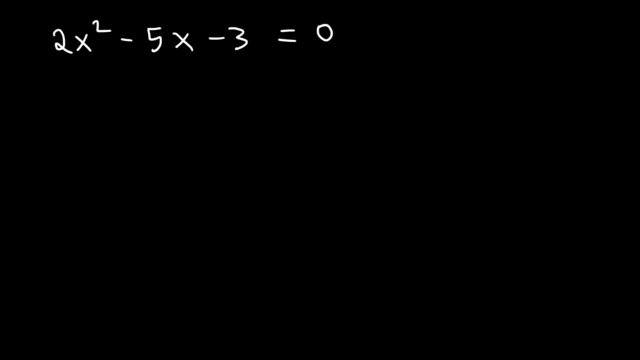 Now let's confirm our answer using the quadratic formula. 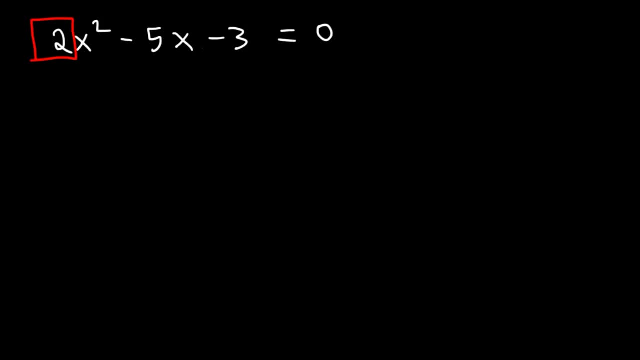 So the first thing we need to do is multiply the leading coefficient by the constant term. 2 times negative 3 is negative 6. Next, we need to find two numbers that multiply to negative 6 but add to negative 5. This is going to be negative 6 and 1. Negative 6 plus 1 is negative 5. 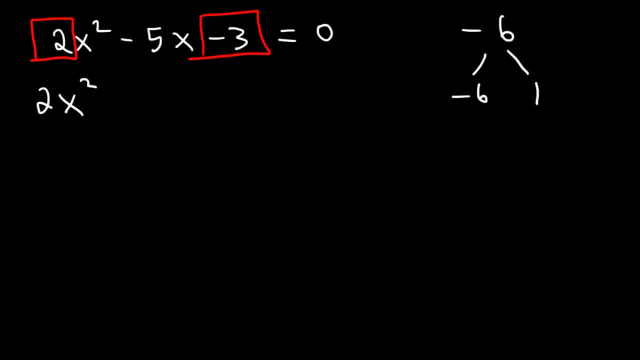 Now what we need to do is replace the middle term, that is negative 5x, with two things, negative 6x plus 1x, because they add up to negative 5x. 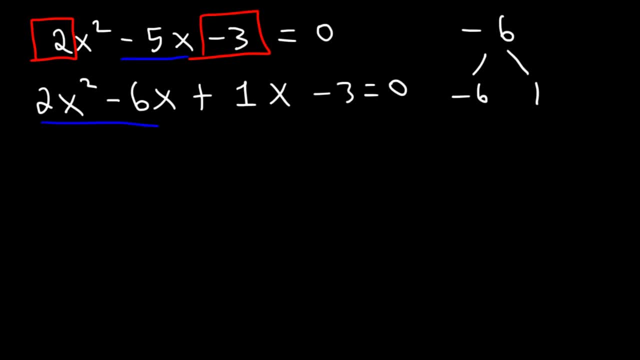 And then we're going to factor by grouping. So if we group the first two terms and the last two terms, let's take out the GCF in the first two terms. The GCF is 2x. 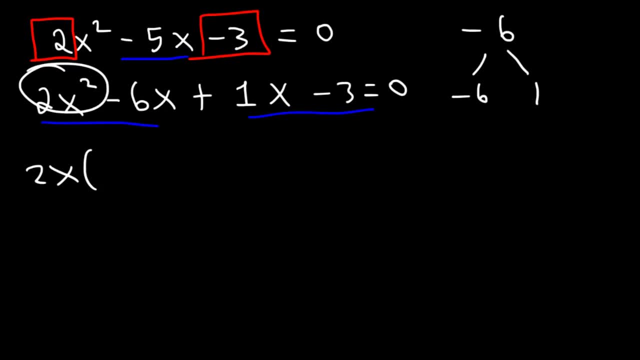 2x squared divided by 2x is x. Negative 6x divided by 2x 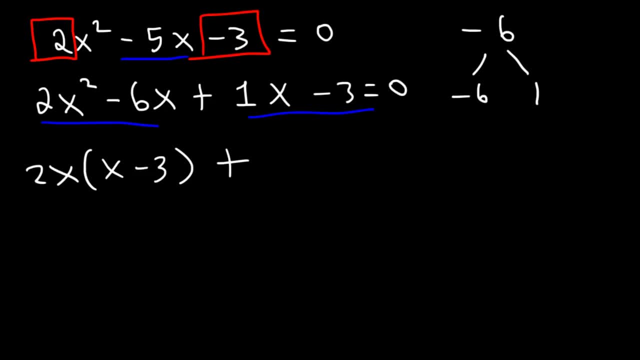 is negative 3. In the last two terms, there's nothing to take out, so let's take out a 1. And the x minus 3 will remain the same. If these two are the same, then you're on the right track. 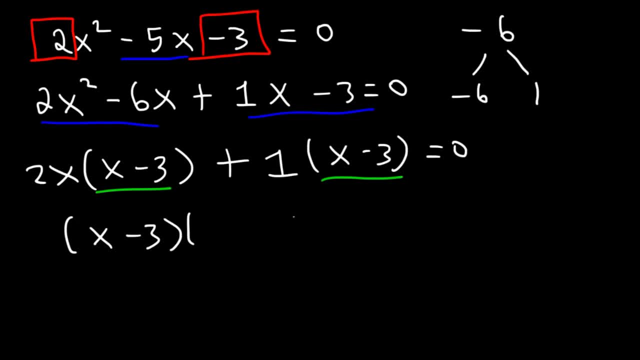 So write those two things once, and on the second parenthesis, whatever you see on the outside, that's going to go into the second parenthesis. 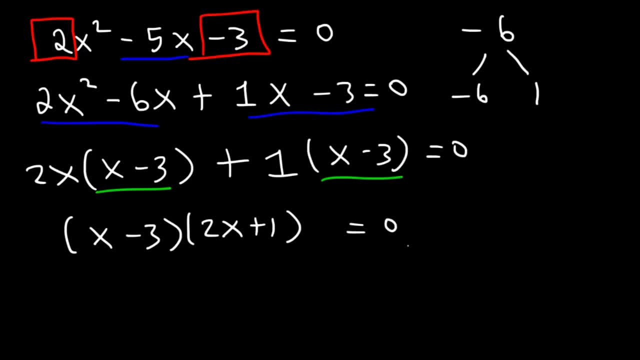 So that's 2x plus 1. So that's how you can factor the expression. 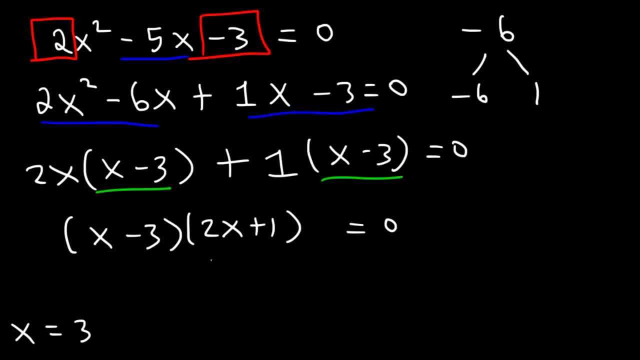 So therefore, x is equal to 3, and if we set 2x plus 1 equal to 0, 2x is equal to negative 1. 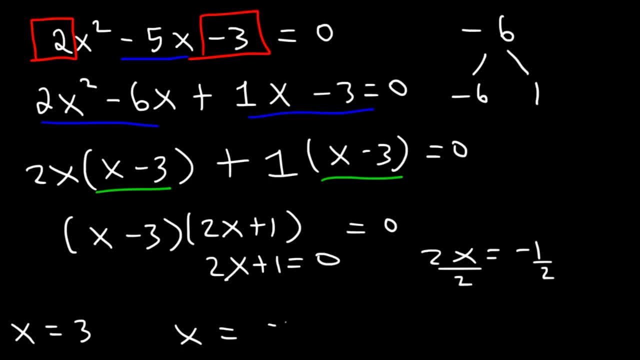 And then if we divide by 2, we can see that the other answer is negative 1 half. 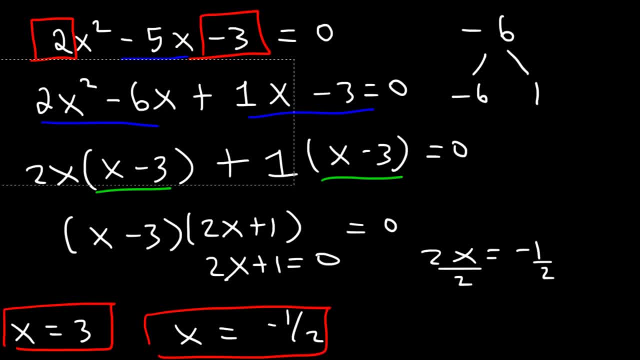 Now let's get these answers using the quadratic formula. . 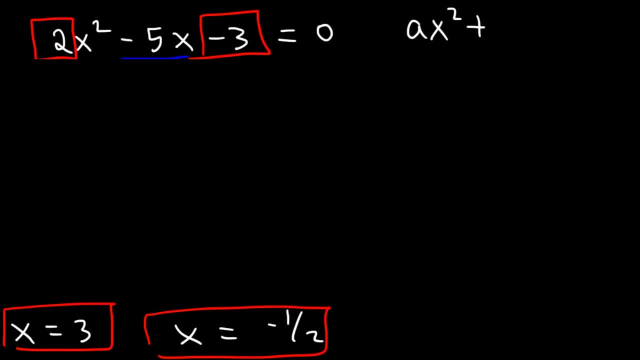 So to use the quadratic formula, it has to be in the form ax squared plus bx plus c is equal to 0. So therefore, we can see that a is 2, b is negative 5, c is negative 3. So x is equal to negative b plus or minus the square root of b squared minus 4ac 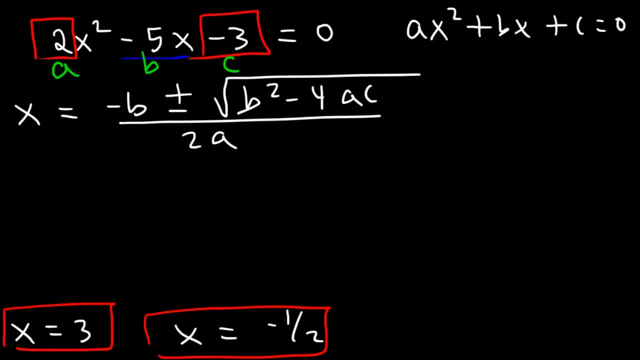 divided by 2a. That's the quadratic formula. 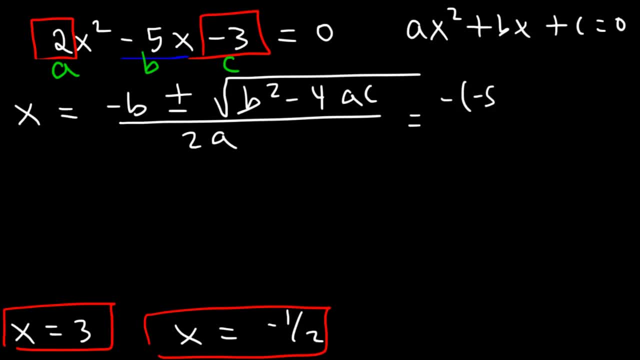 In this example, we can see that b is negative 5. 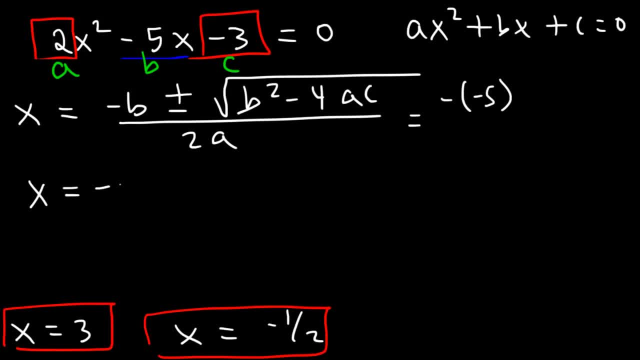 I'm going to run out of space there, so let's start here. 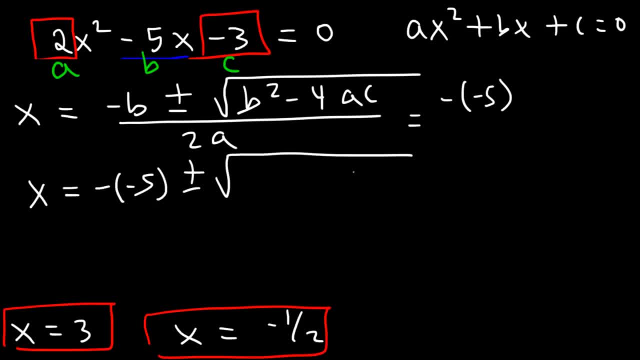 b squared negative 5 times negative 5 that's 25 minus 4 times a times c divided by 2a or 2 times 2. 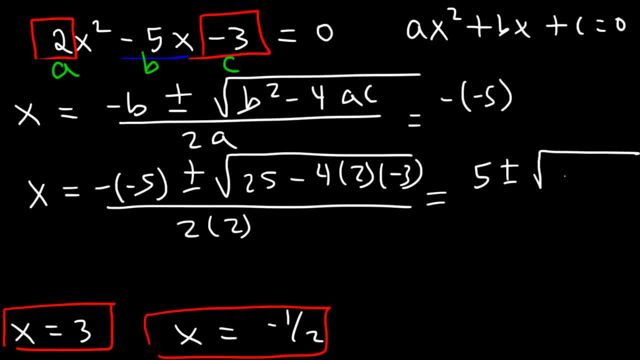 So this is going to be positive 5 and then we have 25. Negative 4 times 2 is negative 8 times negative 3, that's positive 24. And 2 times 2 is 4. 25 and 24 is 49. And the square root of 49 is 7. So we have 5 plus or minus 7 over 4. 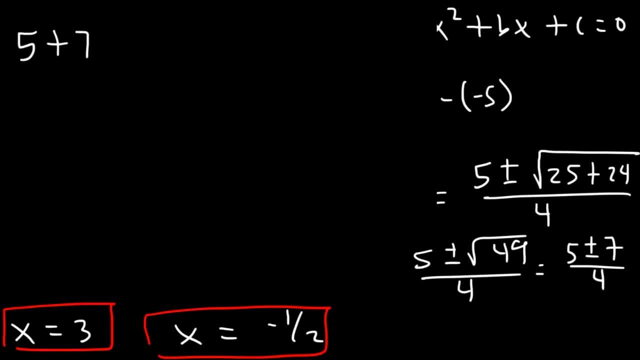 So we can write that two ways. 5 plus 7 over 4 and minus 7 divided by 4. 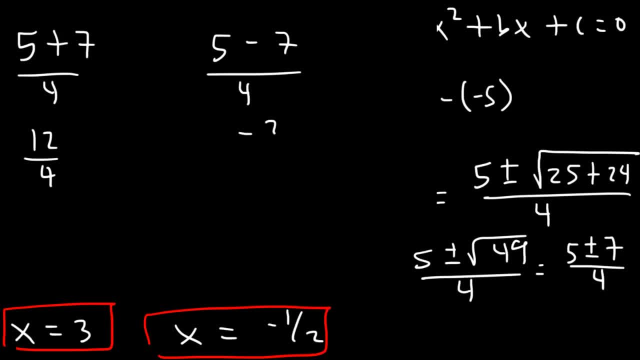 5 plus 7 is 12. 5 minus 7 is negative 2. 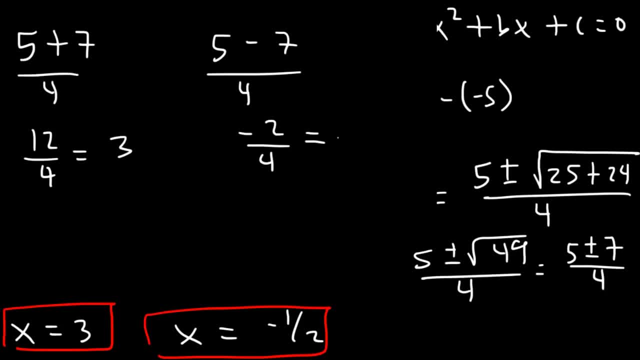 12 divided by 4 is 3. Negative 2 over 4, if you divide the top number by 2 and the bottom one by 2, this will give you negative 1 over 2. 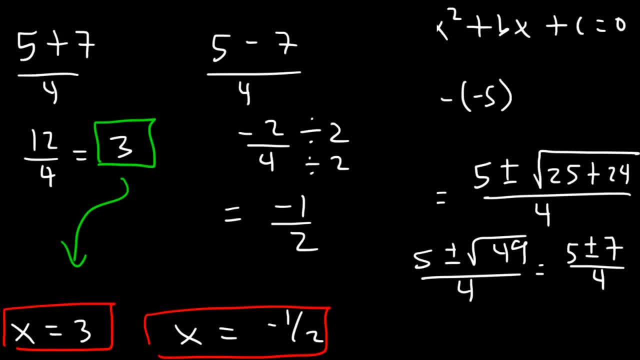 So as you can see, we have the same two answers. 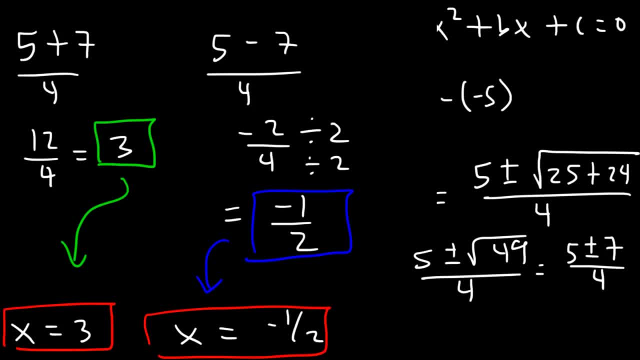 So you can solve any quadratic equation with the quadratic formula. 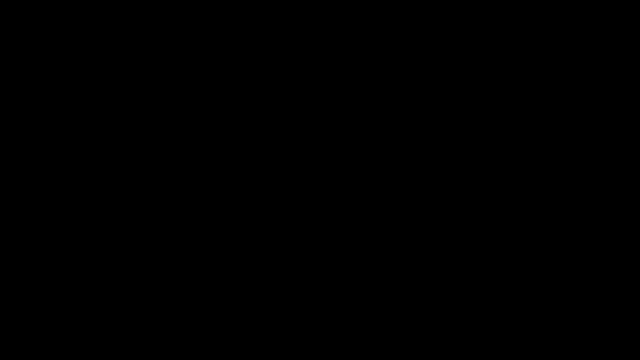 Now let's review some basic properties of exponents. 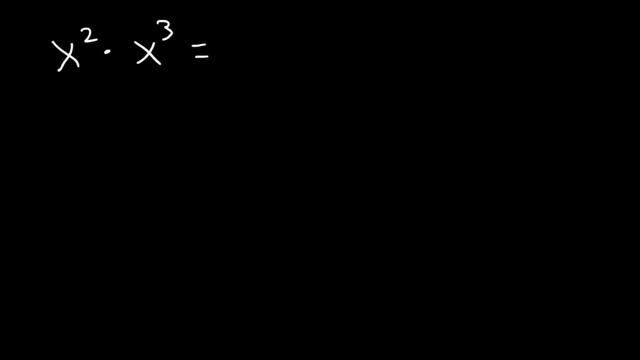 What is x squared times x cubed? Whenever you multiply two common bases you need to add the exponents. This is going to be 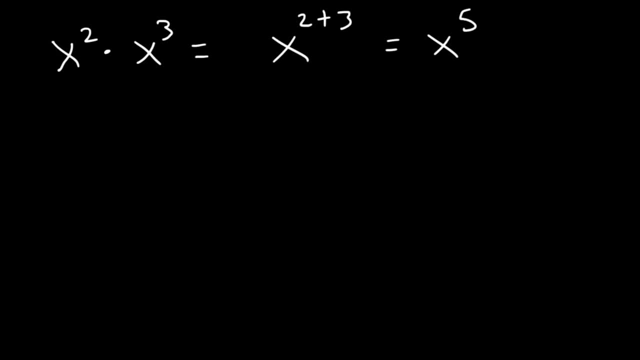 2 plus 3 which is 5. 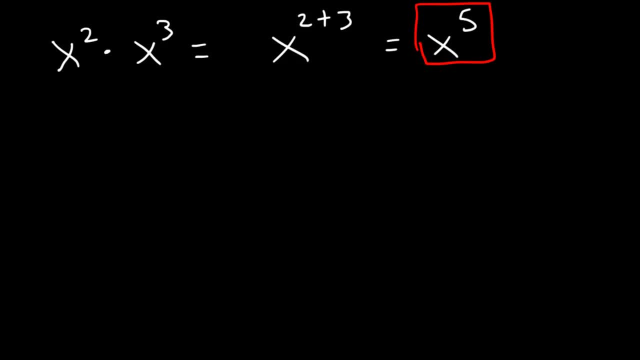 Now let's understand why. x squared means 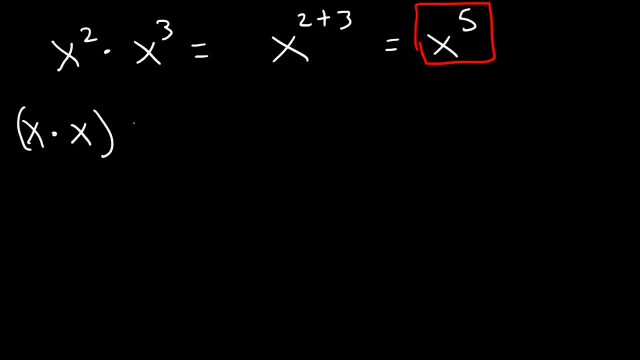 that you're multiplying two x variables together. 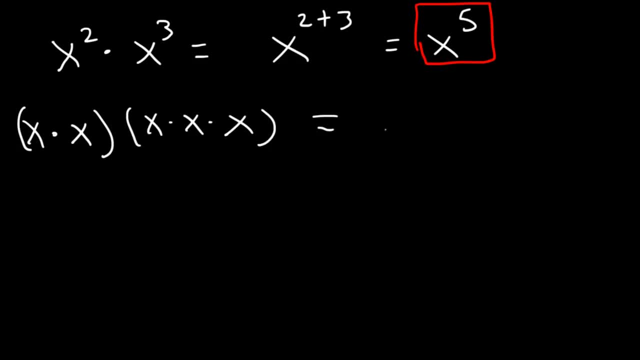 x cubed means that you're multiplying two x variables together. 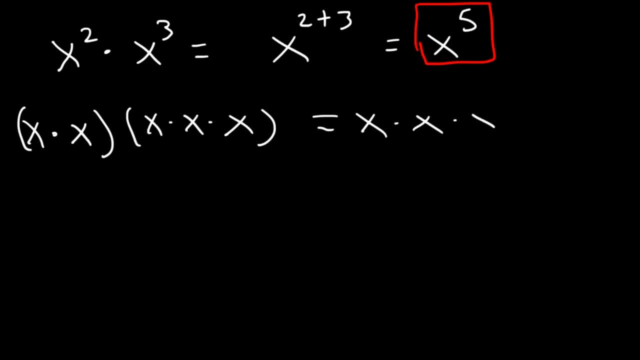 So in total, you have 5 x variables being multiplied, so therefore it's x to the 5th power. 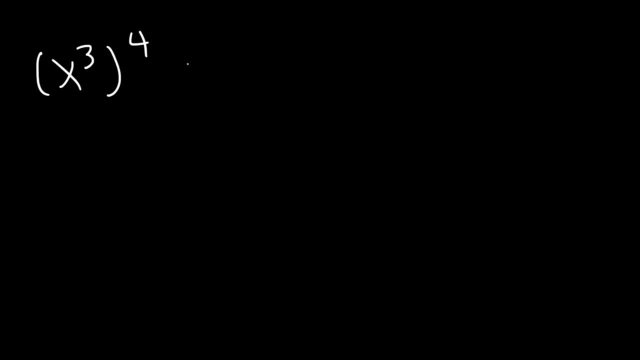 Now what if you raise one exponent to another? What do you do? In a situation like this, you need to multiply the two exponents. So it's x to the 12th. 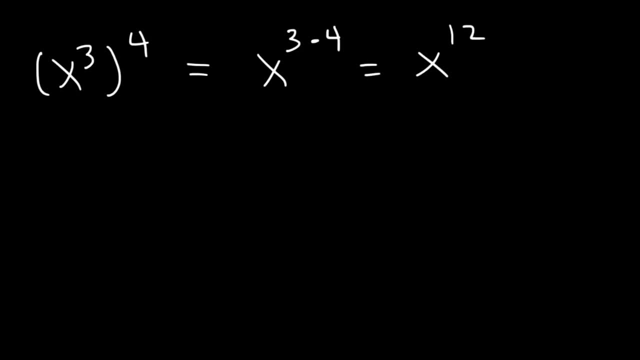 Now let's understand why. x cubed raised to the 4th means that we have three x cubed multiplied to each other. And each x cubed is basically three x variables multiplied to each other. 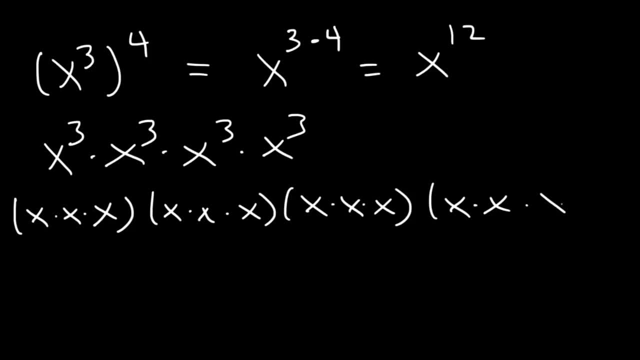 So what we have is a total of 12 x variables being multiplied, so it's x to the 12th. 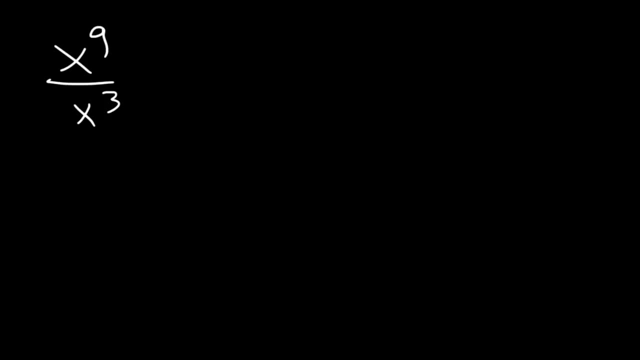 Now what about division? What do we need to do if we're dividing by a common base? If we're dividing, we need to subtract. 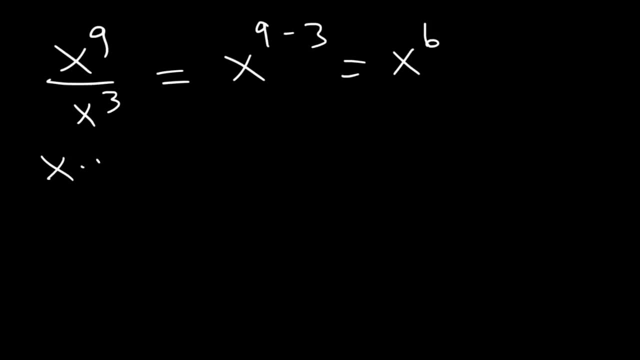 So this is x to the 6th power. x to the 9th power means that we're multiplying nine x variables together. 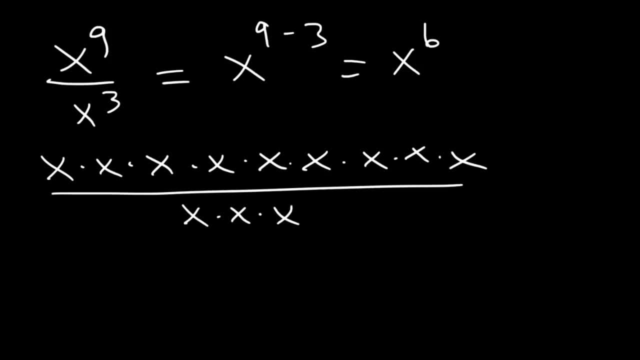 And x cubed is simply three x variables. So we can cancel three x variables together, leaving behind six x variables on top. And so that's why it's x to the 6th. 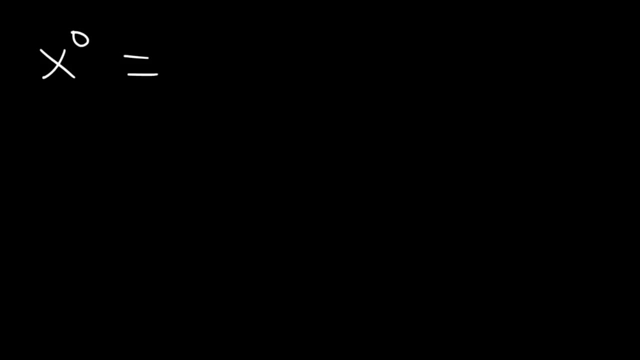 Now x to the 0th power is equal to 1. Anything raised to the 0th power is 1. So keep that in mind. 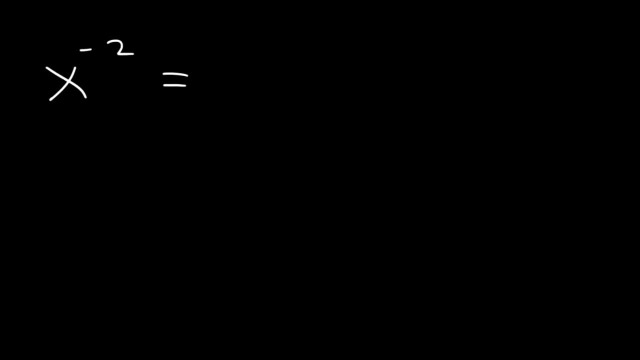 Now what if you were to see a negative exponent? Typically, in algebra, you want to get rid of any negative exponents, you want to make it positive. To do that, you need to move the x variable from the numerator to the denominator. 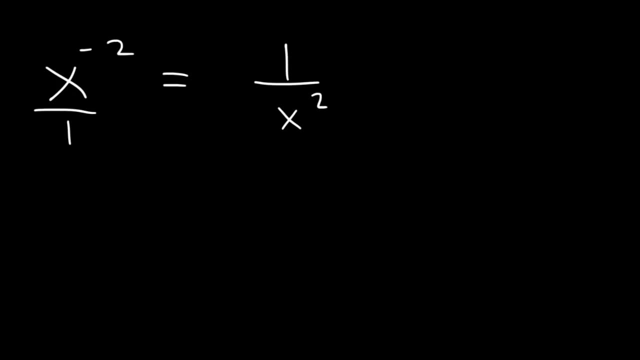 If you change its position, the sign of the exponent will change, so now it's 1 over x squared. 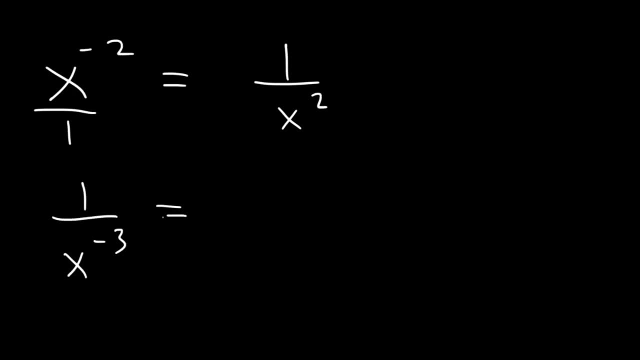 So likewise, if we have 1 over x to the negative 3, if we move the x variable to the top, the exponent will change sign. So it's going to be x to the positive 3. 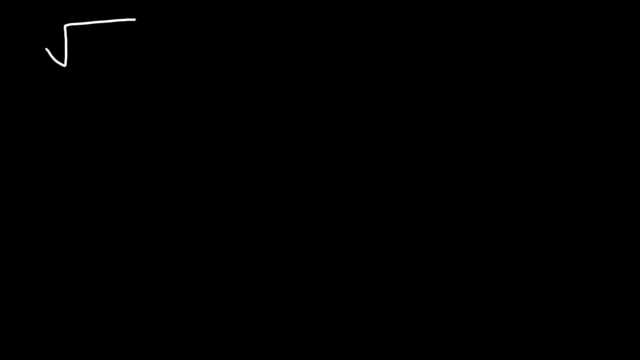 The last thing that we're going to talk about is simplifying radicals. 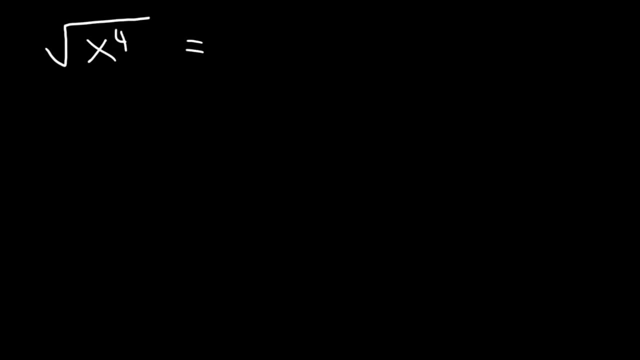 What is the square root of x to the 4th power? 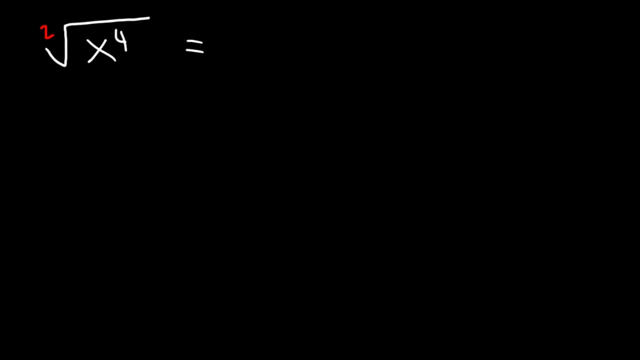 When dealing with square roots, you need to realize that the index number is 2. So this is equivalent to x raised to the 4 divided by 2. So it's x squared. 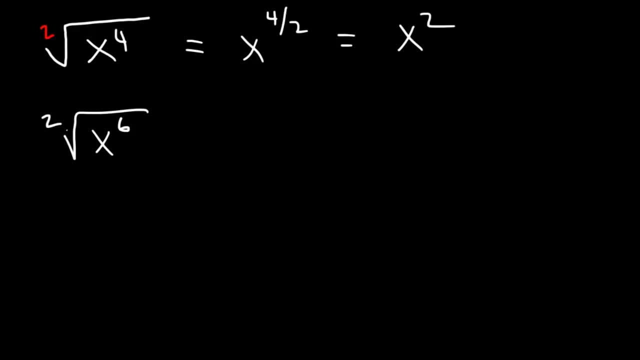 Now what about the square root of x to the 6th? 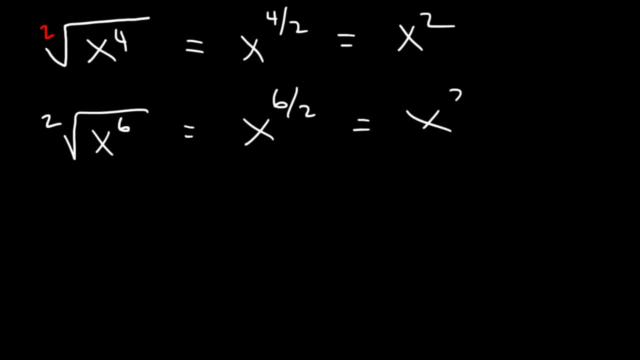 So this is going to be 6 divided by 2, which is 3. 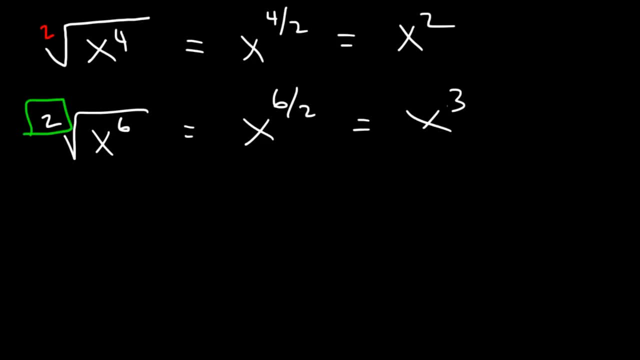 However, whenever you have an even index number, and if you get an odd exponent, technically, this should be placed in an absolute value symbol. 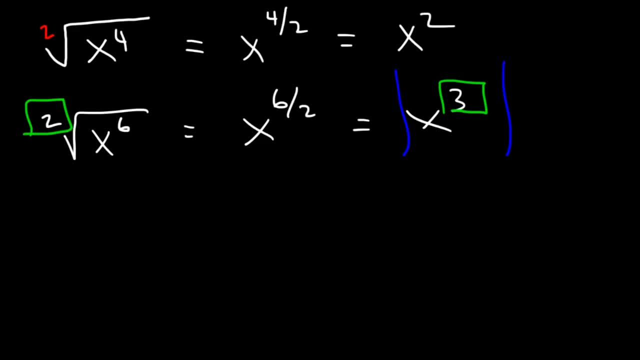 Now some teachers may not test you on this, but others will, so it's just good to know that fact. 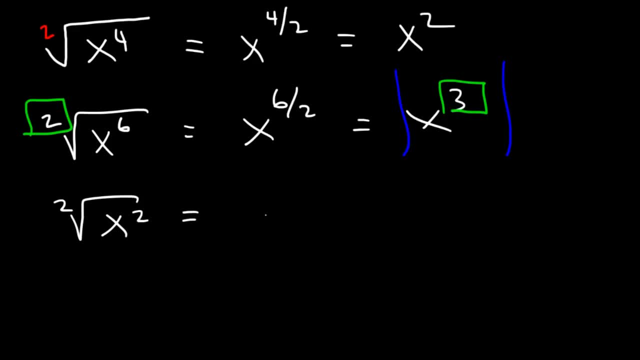 So for example, the square root of x squared is equal to basically x to the 1st power, or x. 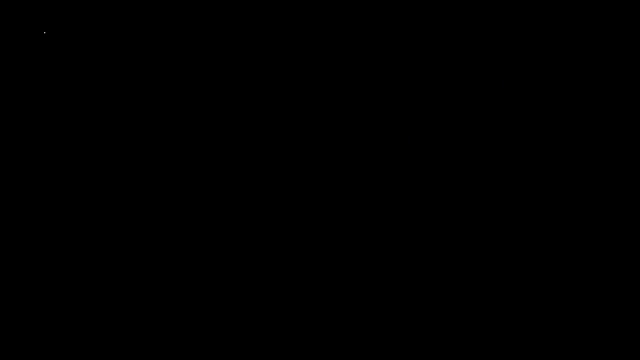 So you need to put that in absolute value. Now what about the cube root 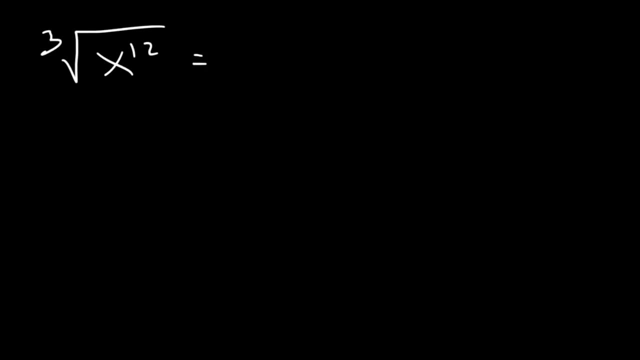 of x to the 12th? This is going to be 12 divided by 3, which is 4. 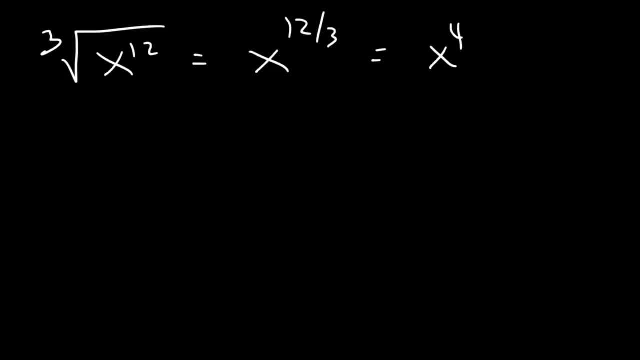 Whenever you have an odd index number, you never need the absolute value symbol. So this is just the answer.